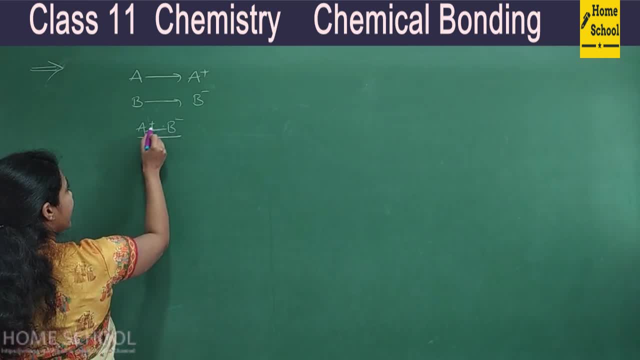 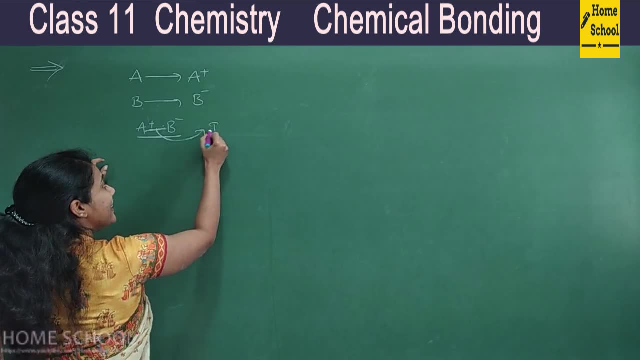 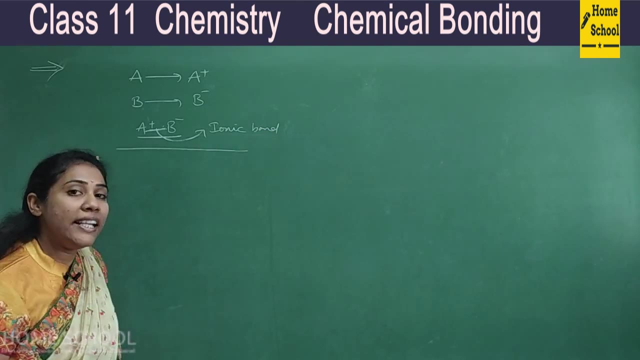 come near, they stay together and an attraction gets created between A plus ion and B minus ion, and we call that bond as ionic bond. It is ionic bond, right, Okay? And we have also studied how covalent bonds are formed. 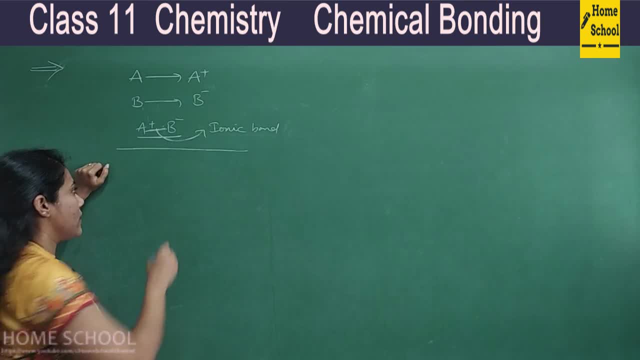 See, covalent bonds are formed by sharing of electrons. You have hydrogen, You also have chlorine. Hydrogen has one electron, Chlorine. in its outermost shell, you will find seven electron right. So what happens here? Sharing of these two electrons takes place between hydrogen and 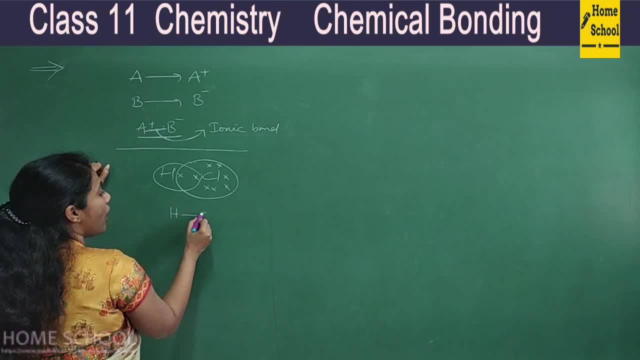 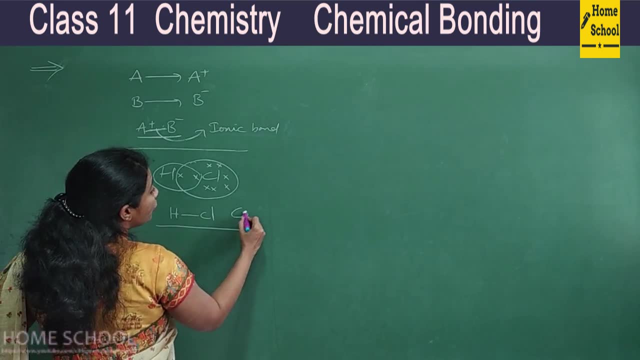 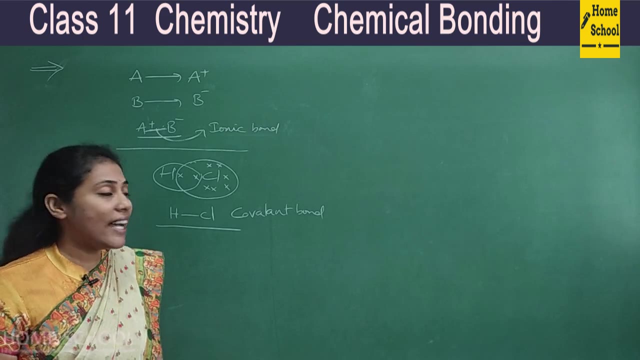 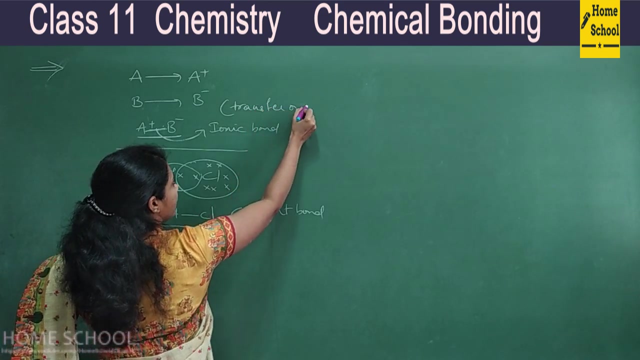 chlorine, And this leads to the formation of covalent bond between hydrogen and chlorine. So this is how our covalent bonds will form right. So in general, if I have to revise, ionic bonds are formed by transfer of electrons. transfer of electrons and covalent bonds are: 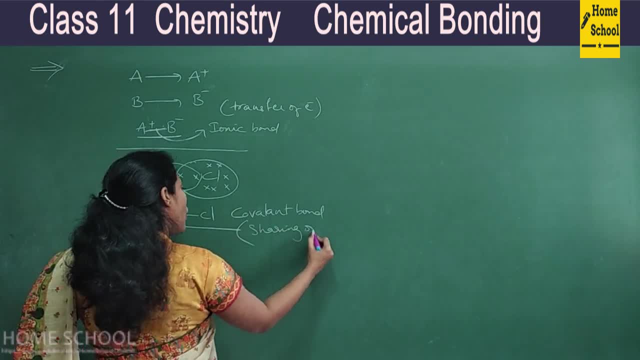 formed by sharing of electrons. So all that we have already discussed, right, Okay, And now what I am going to do is I am going to take a look at the covalent bonds and I am going to take a look at the covalent bonds. 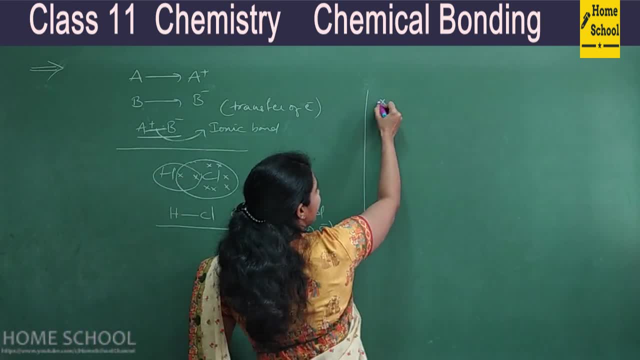 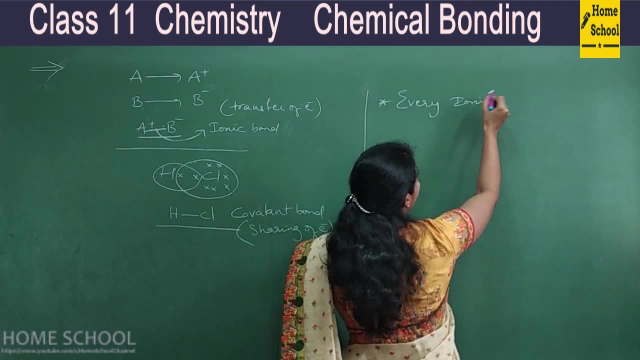 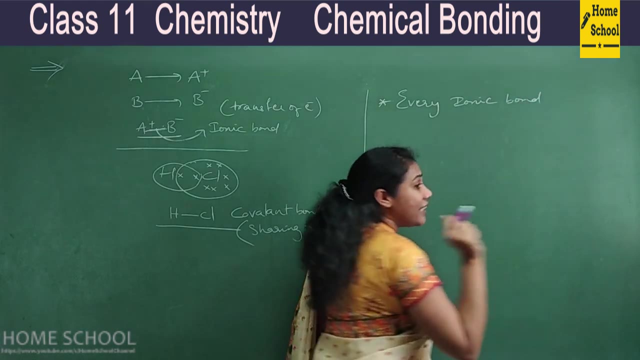 I am going to take a look at the covalent bonds and I am going to tell you ways. Every points are very, very important. Note it down: Every ionic bond, every ionic bond, has certain amount of covalent character. Okay, So no bond is 100% ionic, So you will not have a bond. 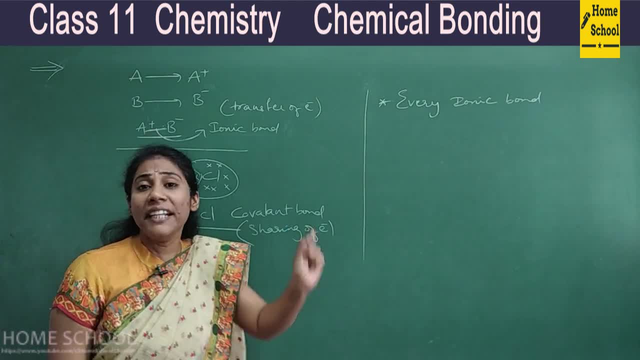 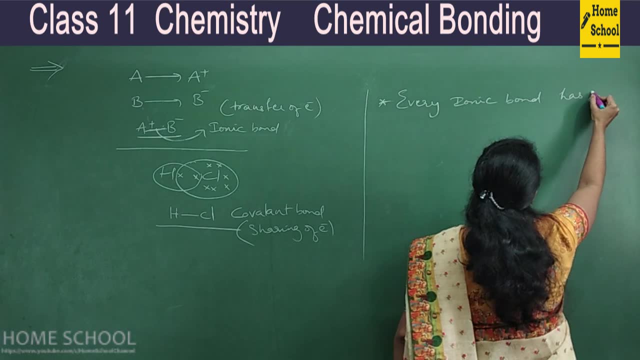 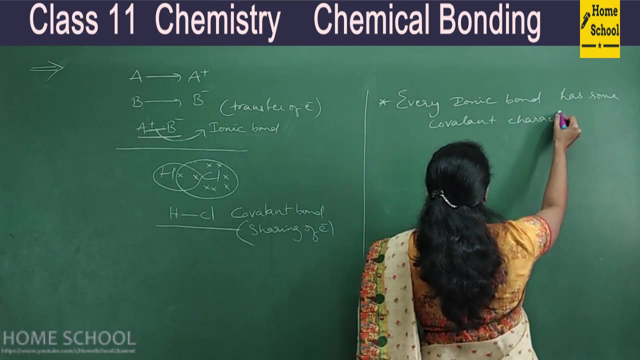 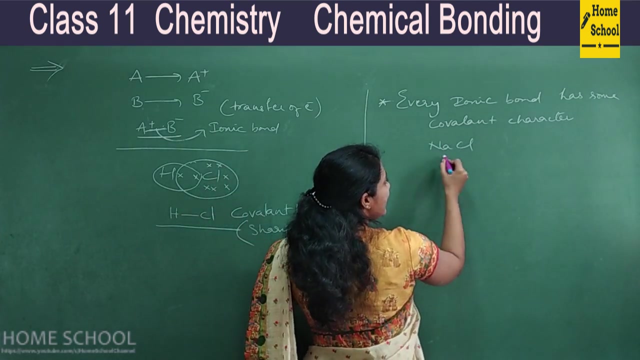 100% ionic. here. Some covalent character you will observe in ionic bond, right? So every ionic bond has some covalent character. covalent character, So how much of covalent character can be present? Say, for example, you have NaCl, NaCl- Normally we say between Na and Cl there is ionic 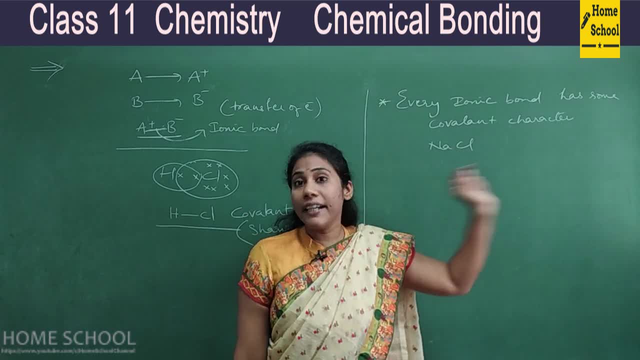 bond, But this bond is not 100% ionic. Some amount of covalent nature is there, So how do you decide that covalent nature is present? So how do you decide that covalent nature is present? So how do you? 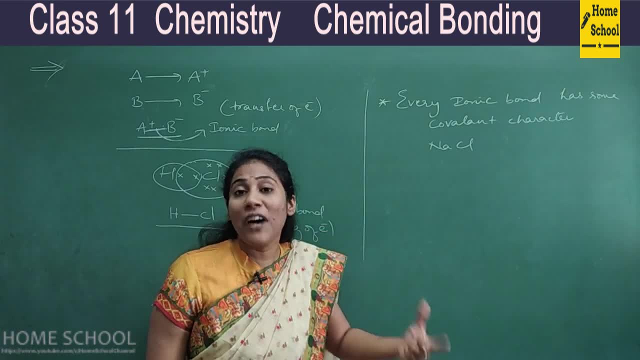 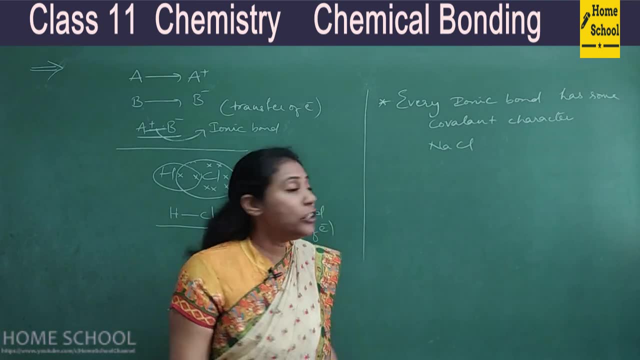 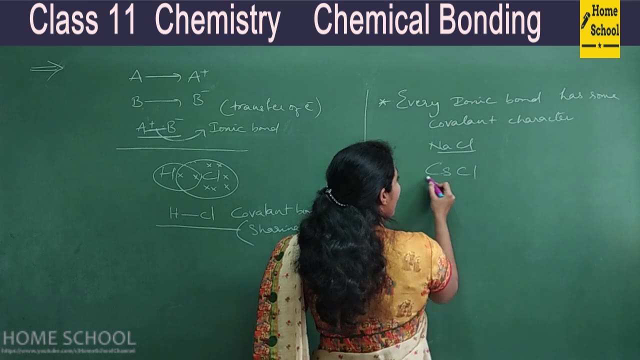 find covalent nature of ionic bond. How do you find how much extent covalent nature is there in this particular ionic compound? Or if you want to compare, say you have sodium chloride, you have cesium chloride, right? So sodium chloride is ionic compound, cesium chloride is also ionic, Both. 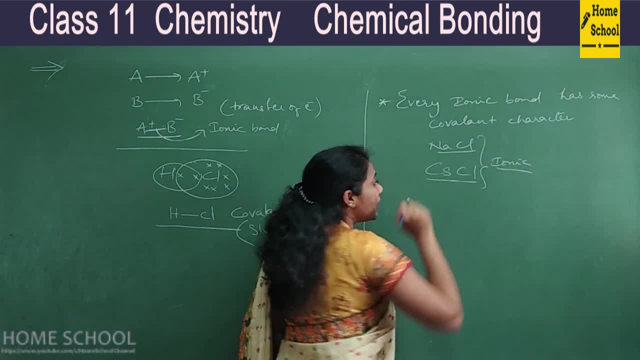 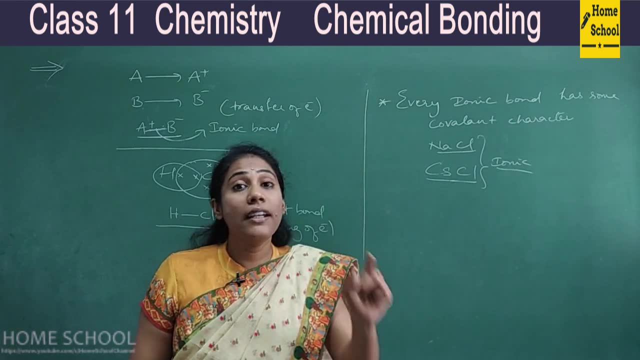 are ionic right. But in which of the compound covalent character is more? I told you, in every ionic compound there is a covalent nature of ionic bond. So if you want to compare, say you have sodium chloride right In every ionic compound little of covalent character, you will observe. 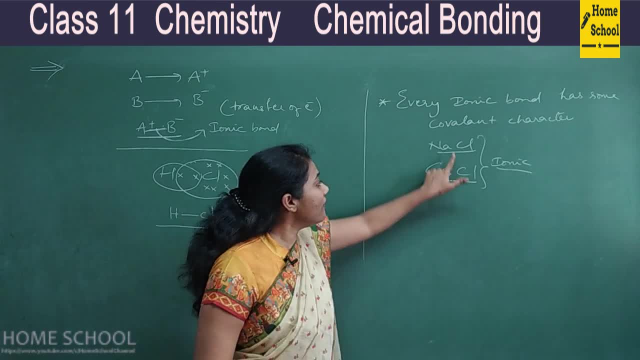 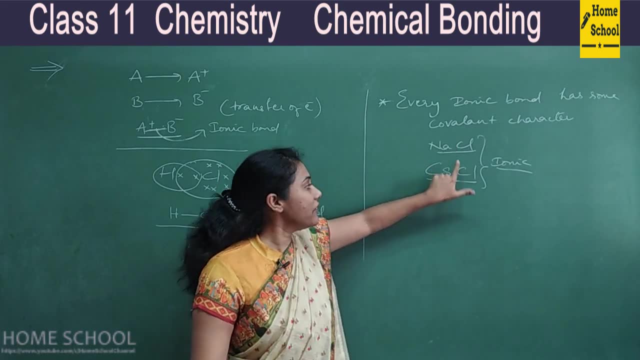 So here both are ionic compound, Both have ionic compounds. I said, covalent character is observed Here. covalent character is observed. Here, though it is ionic bond, little covalent character is observed, But in which case more covalent. 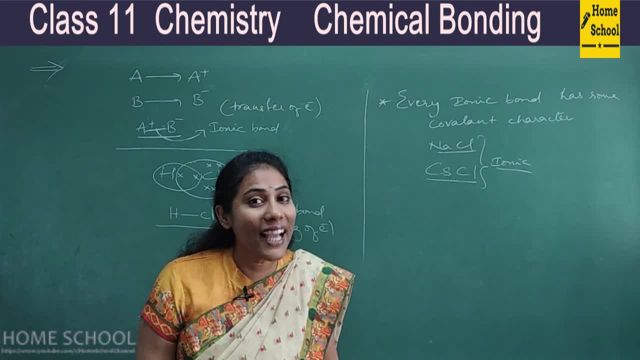 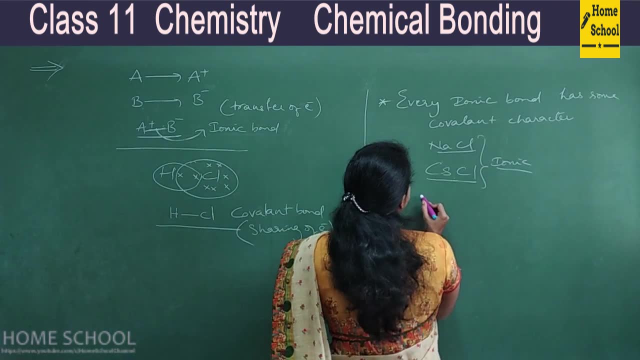 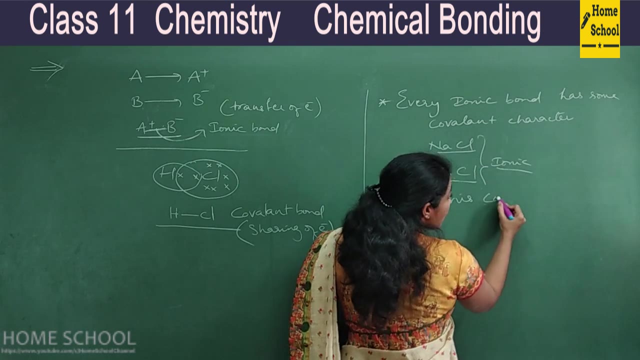 nature is there. So how do you decide that That is decided by a concept of polarization. Let us describe this concept of polarization in context, So that the bonding group can be déplônima form. Okay, So this ionic nature, this ionic, sorry, this covalent nature, covalent nature of ionic. 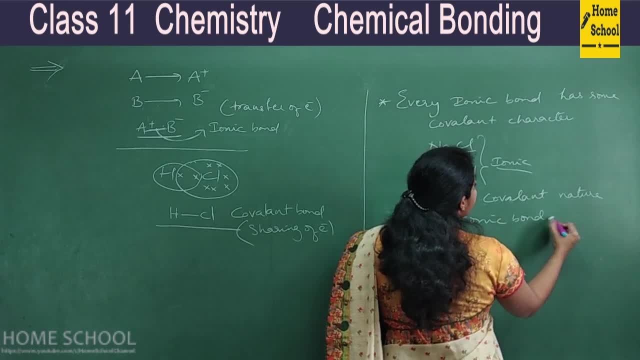 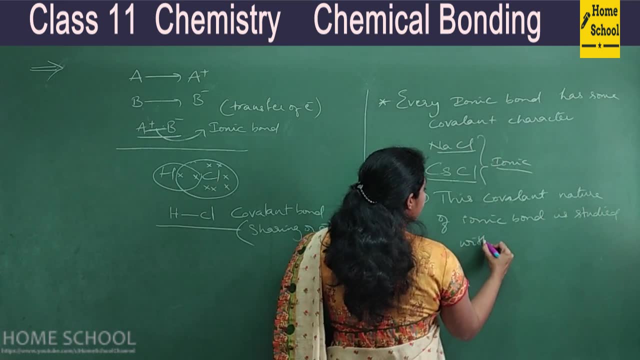 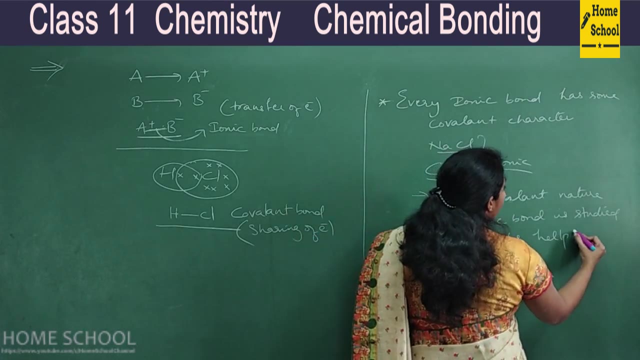 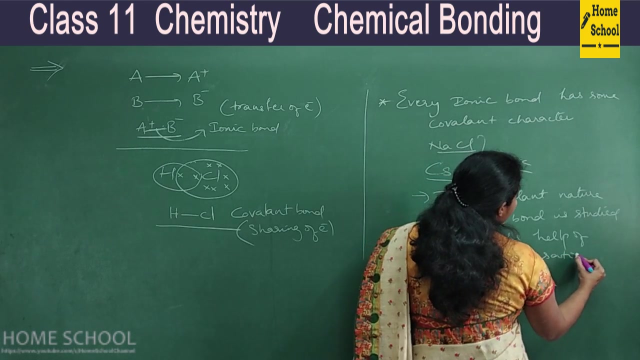 bond, of ionic bond, is studied by a concept, Okay, Studied with the help of. it can be understood in a better way with the help of, with the help of a concept called polarization, Polarization, Okay, So here, polarization. you know, for polarization there are certain conditions. 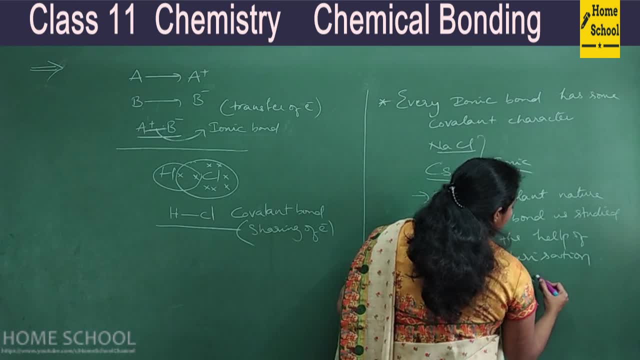 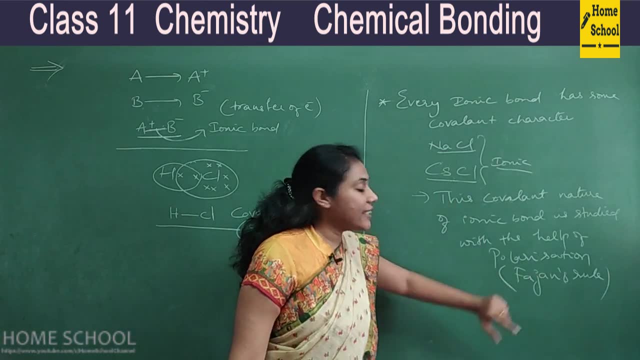 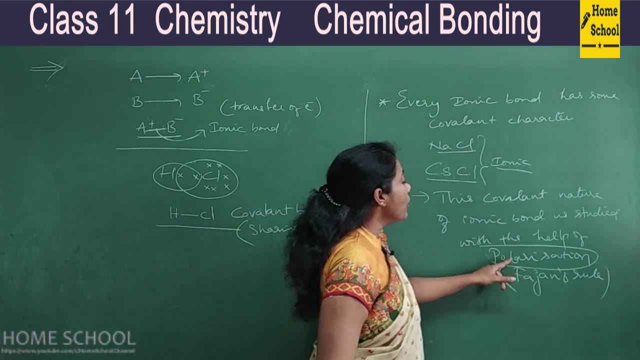 So those conditions we will study as a rule called Fasen's rule, Fasen's rule, Right? So when do you study this Fasen's rule? Fasen's rules are related to a concept called polarization. Okay, So what is polarization? 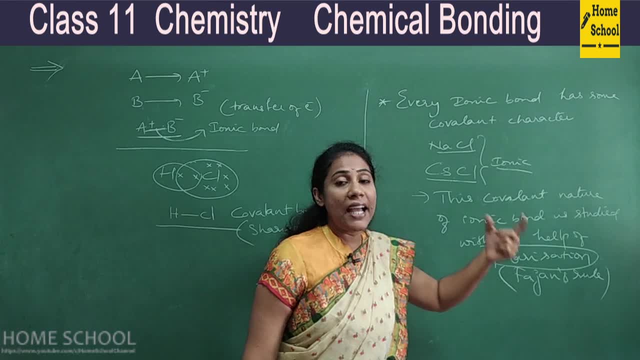 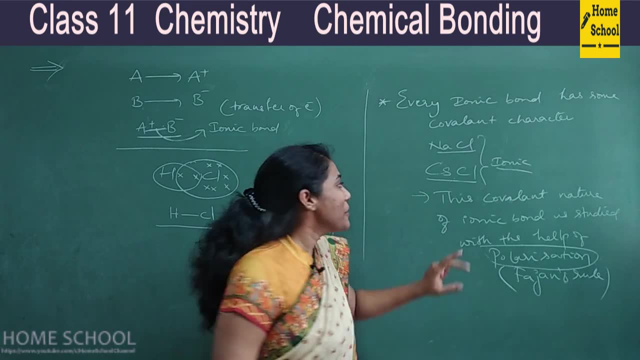 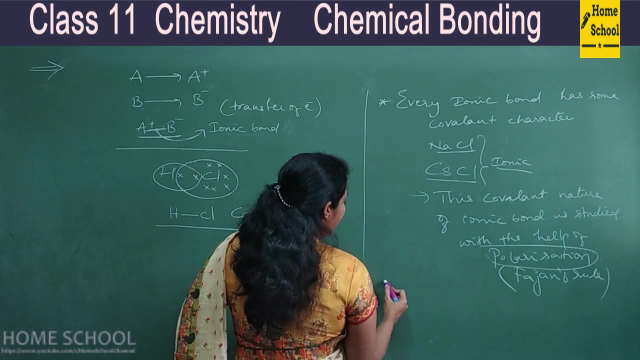 With this polarization concept, you can understand about covalent character of ionic bond in a better way, Right? So hope you understood why we have to study this Fasen's rule and what is the use of Fasen's rule. Okay, So, similarly, every covalent compound has some. 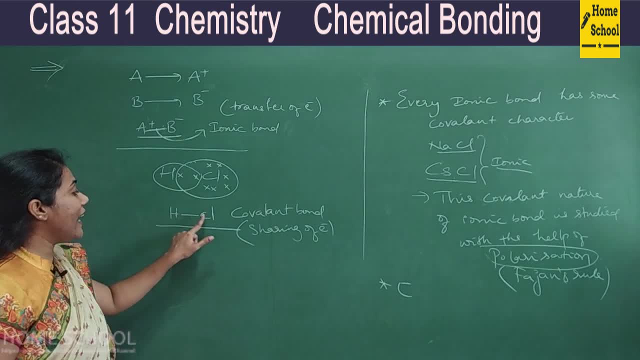 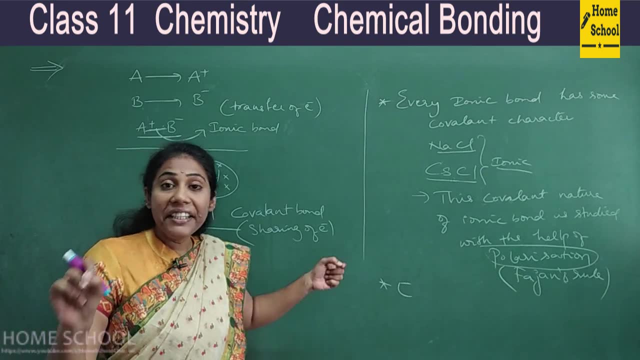 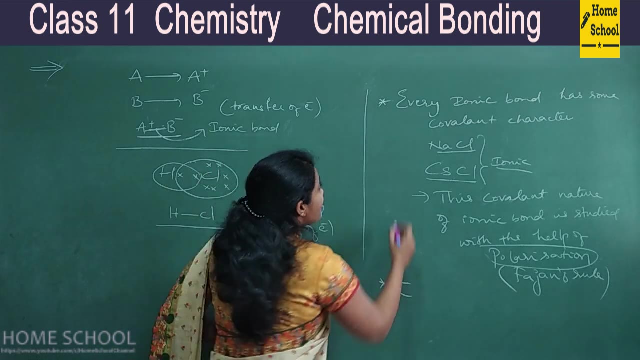 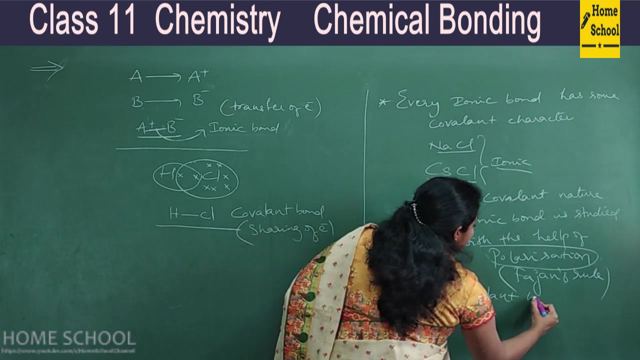 ionic nature. Okay, Say, bond between hydrogen and chlorine is covalent bond, but some amount of ionic nature is there, Ionic character is there. Okay, So that is studied by a concept of dipole movement. Okay, So what I can write here is every covalent bond covalent bond. 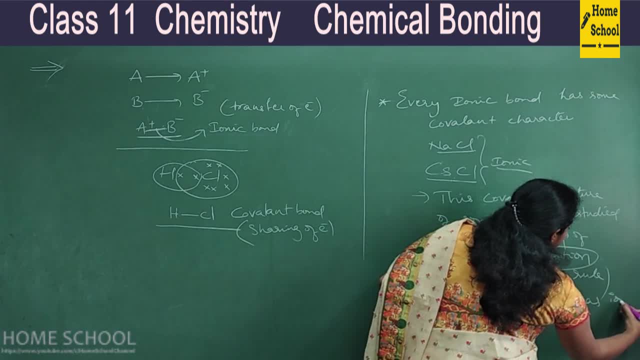 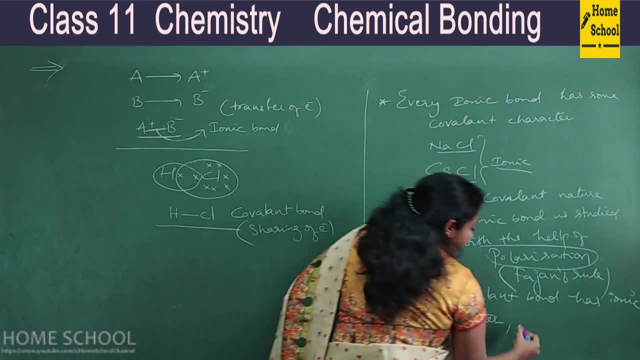 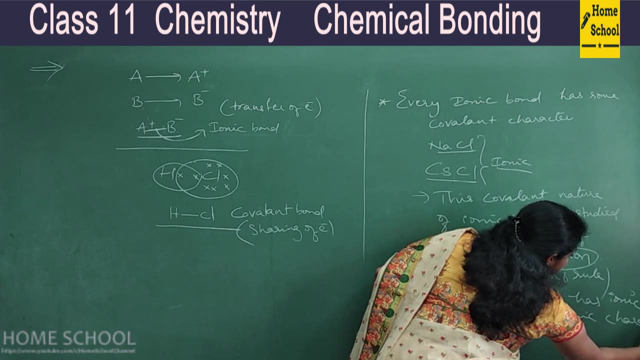 has ionic character. Okay, So each covalent covalent bond has a covalent covalent covalent bond. Okay, So we make a concept here that we can write this as Ionic nature. Okay, So ionic character. okay, so that ionic character is studied by this. ionic character is studied by: 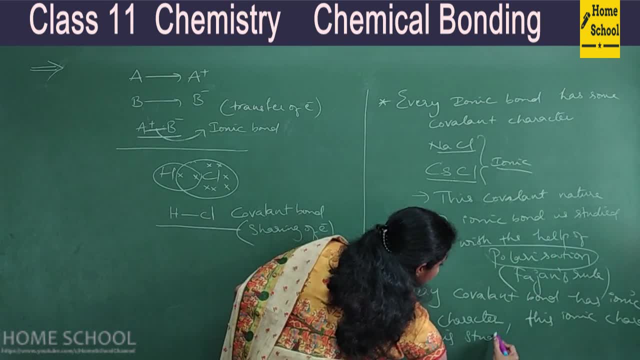 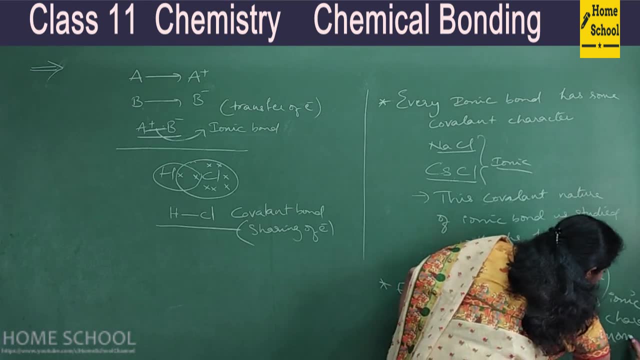 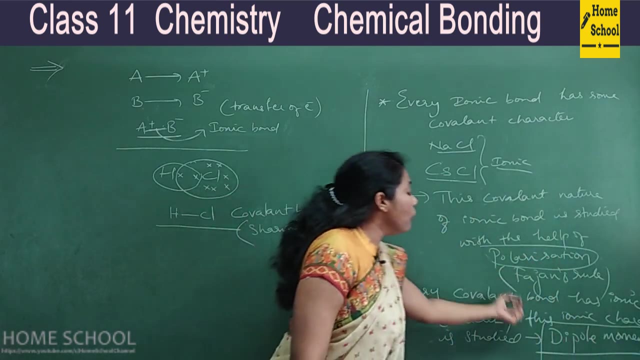 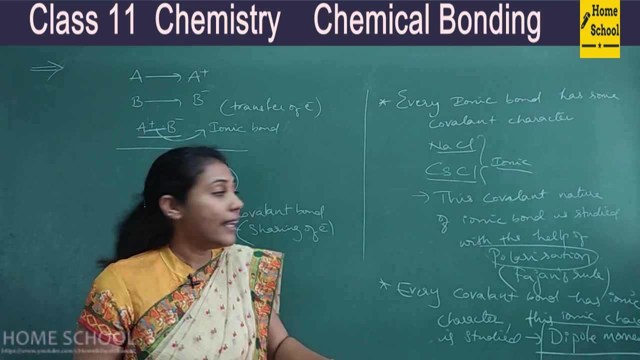 what concept studied with the help of, with the help of a concept: dipole movement. okay, so dipole movement is the concept with which we can understand to how much extent ionic character is there in a particular covalent bond. okay, and polarization is the concept, or phasen's rule is. 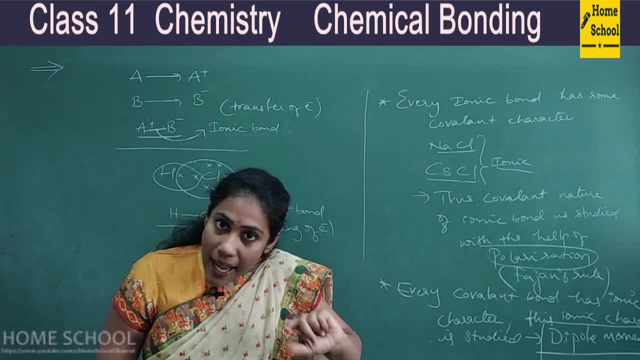 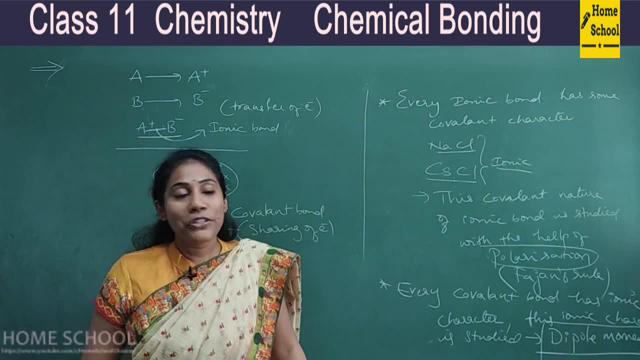 the concept that we study to understand how much covalent character is there in ionic bond. okay, so this is the concept of dipole movement. okay, so dipole movement is the concept with which we can understand to how much covalent character is there in ionic bond. okay, so this is how we have to. 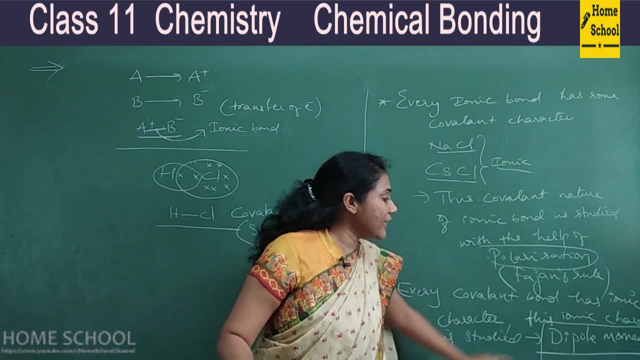 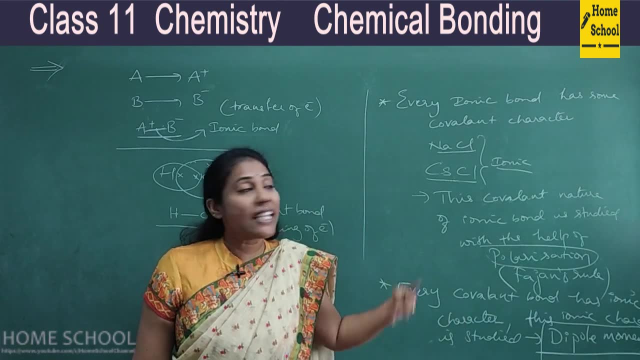 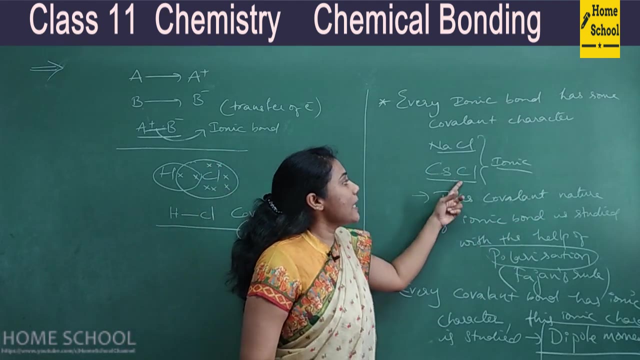 now focus on two concepts. one is polarization, the other one is dipole. moment first, let us learn about the concept of polarization. that means using which we can understand the covalent character of ionic bond. okay, so let's let's solve these types of questions. say, if two ionic compounds are given. 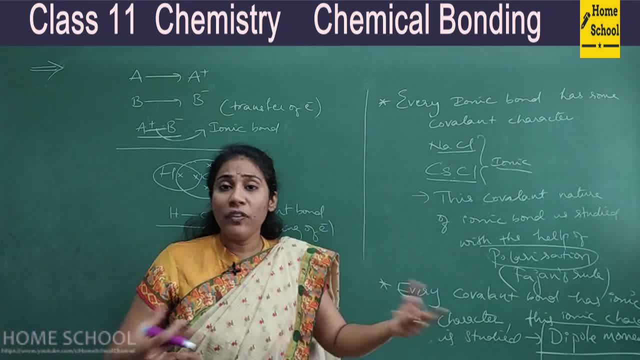 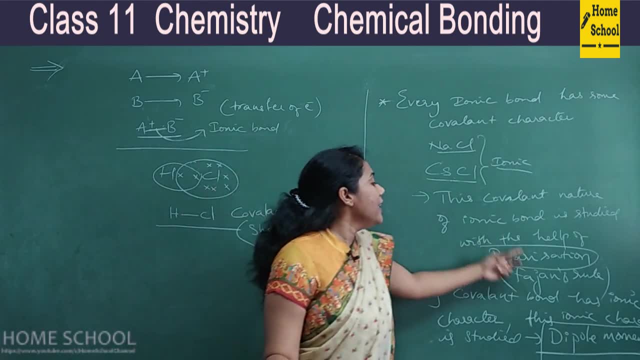 so which of them you know have more covalent character? which has less covalent character? you know all these covalent character which has less covalent character? you know all these types of questions can be solved very easily if you know phasen's rule, if you know the concept of. 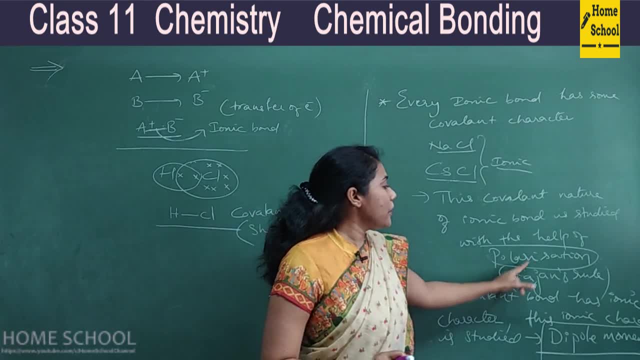 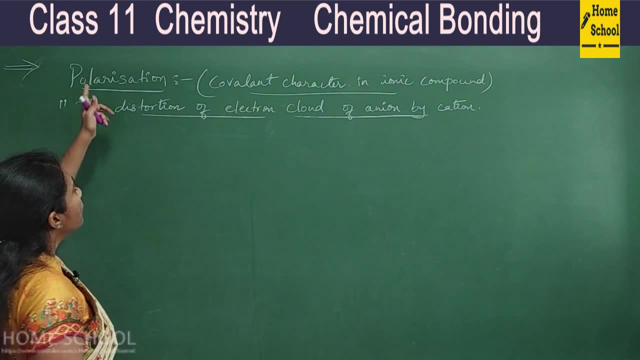 polarization. so let's quickly go for the concept of polarizations or phasen's rule. observe what happens normally here, say, as i already told you, uh, polarization means learning covalent character in ionic compound. you can look at the definition. the distortion of electron cloud of anion by cation is 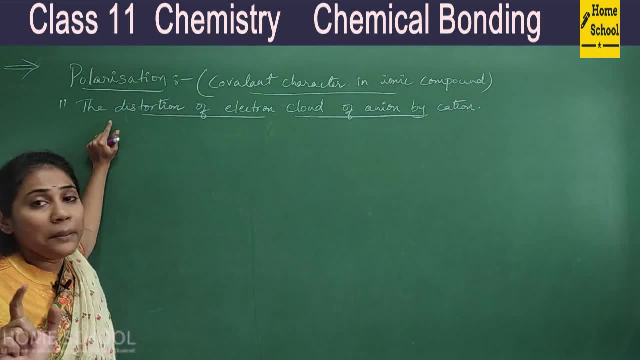 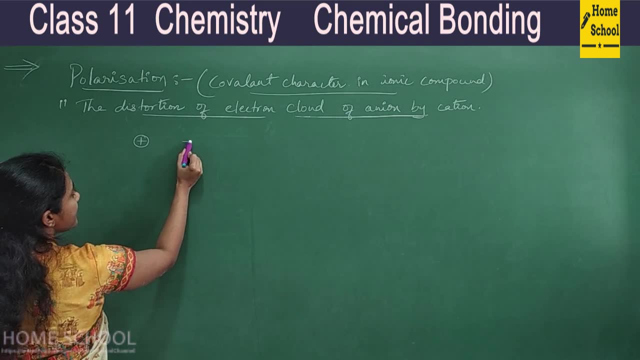 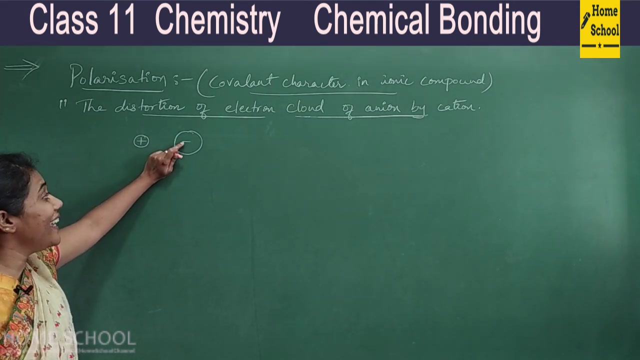 called as polarization. so what do you understand by this sentence? it's very simple. suppose: if this is our cation and this is our anion, right see? uh, you know what? every cation has a nucleus around that electrons are there and every anion will have a nucleus around that electron cloud is there. 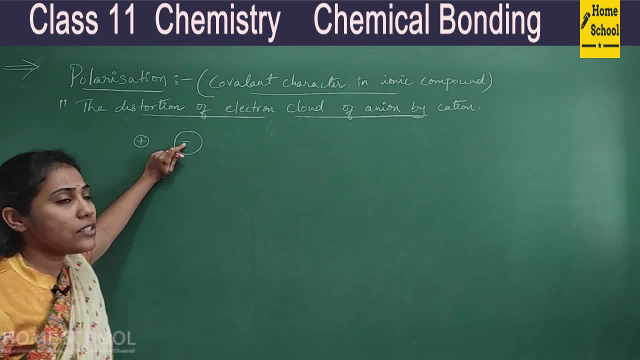 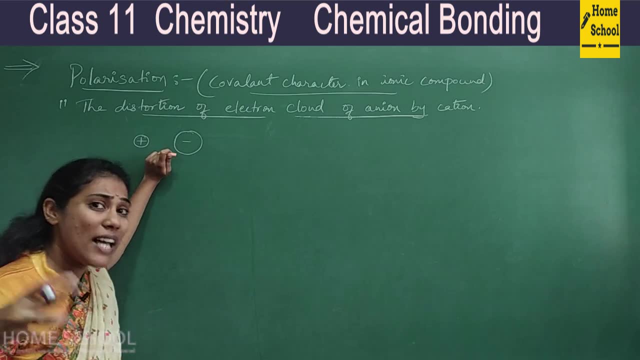 see, in case of anion, more number of electrons. so if you have more electrons around the夠 anion cation is more good. you know nonpoint. you can see anion cloud sounds like this, so i can say more electron cloud, electron cloud in the sense. 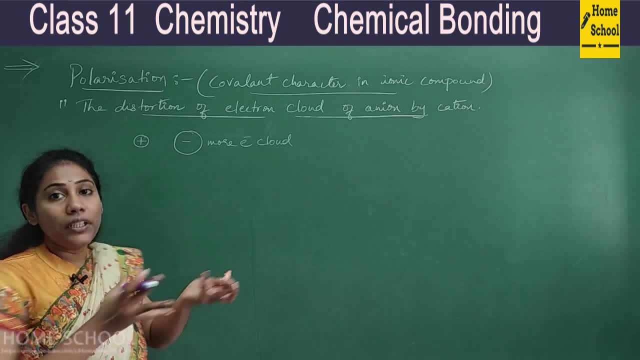 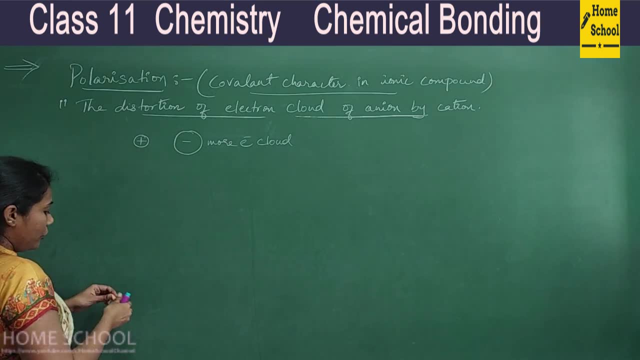 what? the area where electrons are more okay. so anion has more electron cloud, so electron density is more around the anion, right, more number of electrons- fine, see, when they come near. you know ionic bond, you know both of them should be near right. So when this anion comes near, what happens? 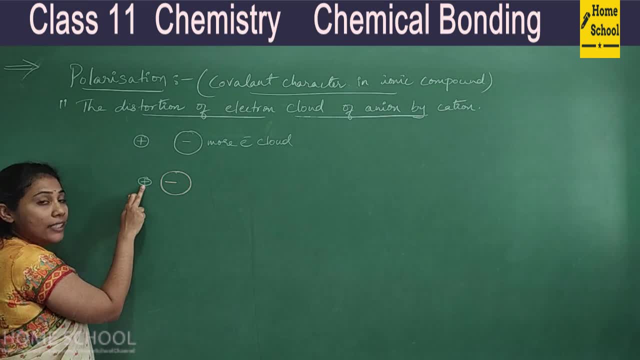 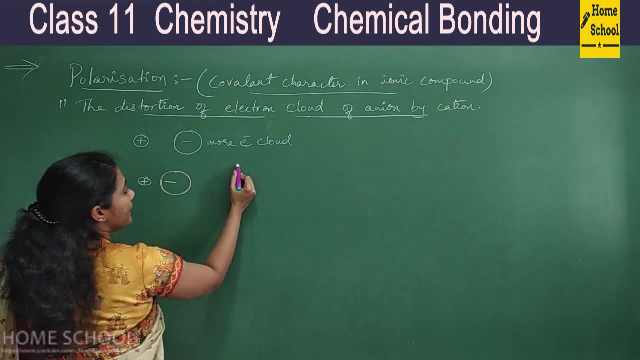 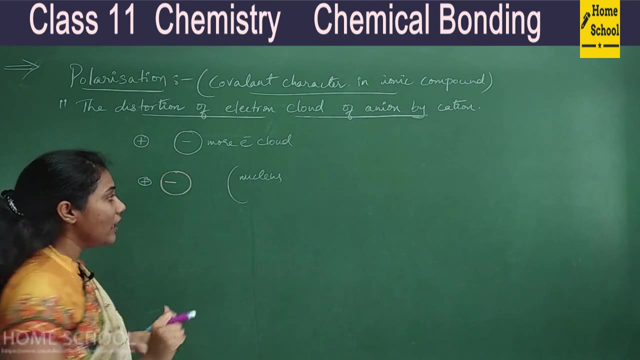 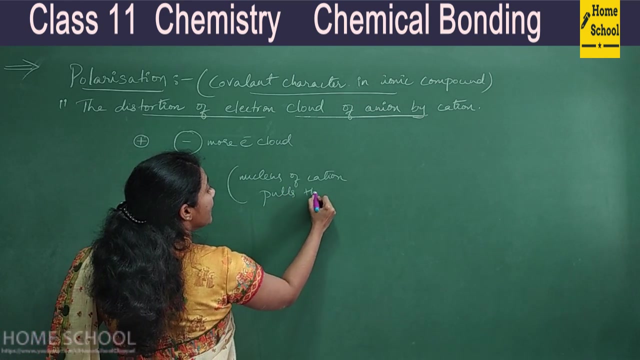 is the positive charge of cation will try to pull the electron cloud towards itself. okay, Actually speaking, what can happen here is nucleus. nucleus of cation is very strong. it is highly positive in nature, right? So nucleus of cation, what happens, pulls, pulls the electron cloud of anion. 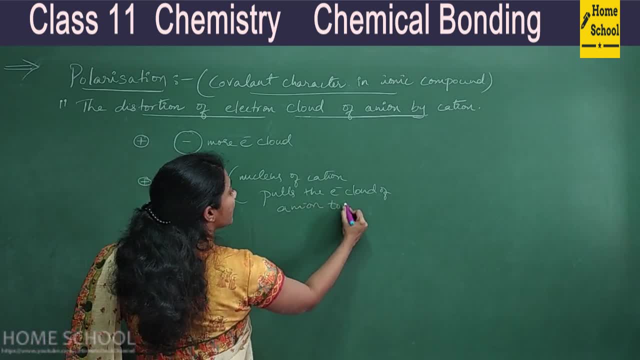 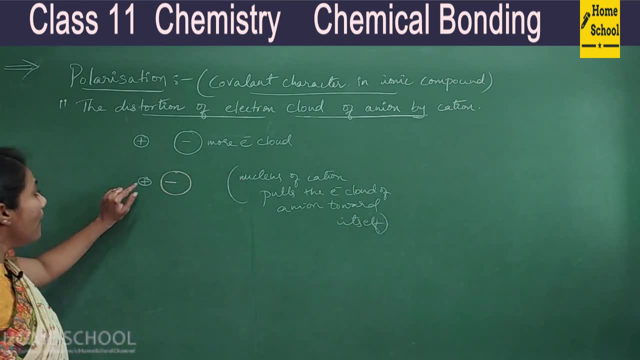 towards itself, towards itself, right? So that itself we will call it as polarization. So positive charge of nucleus is very strong in cation. okay, So this guy, it will see the electron cloud. since there is an attraction between positive and negative, you know what electron cloud will? 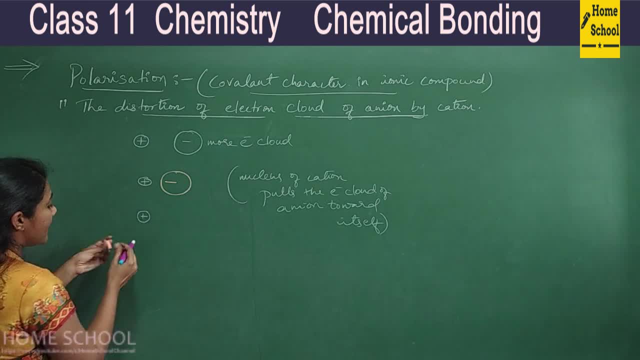 tend to move more towards. you know, this is a cation stage as it is. but electron cloud, you see it is slightly moving towards positive charge. okay, say, here deviation of ionic character took place. okay, so the electron cloud is moving more towards positive side. okay, so it's like the 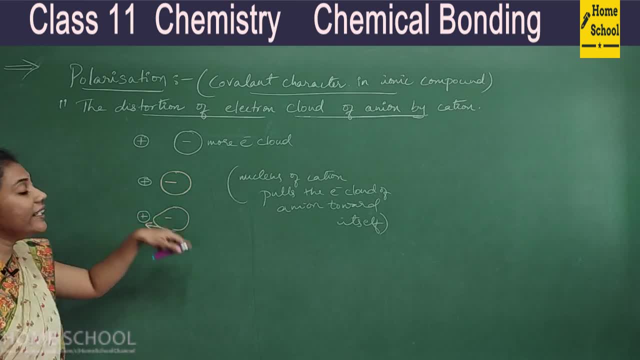 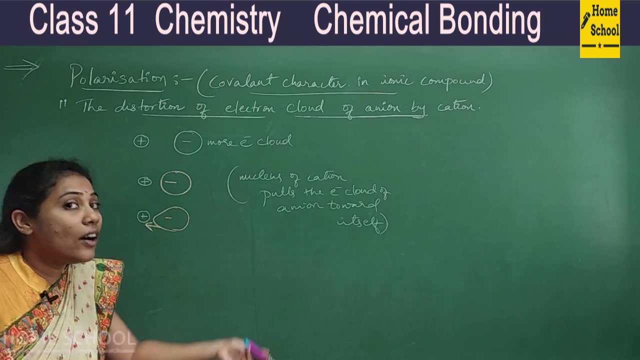 electron cloud is shared between positive and negative guy here. so if anything is shared between the ions or atoms, we call it as covalent character, isn't it? see, cations, positive charge is very strong that it is attracting, you know, the electron cloud of anion. 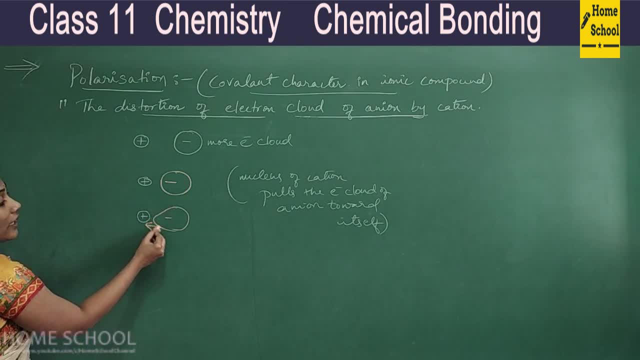 distortion in the sense what the electron cloud of anion is moving. it is distorted, it is getting deviated towards the positive cation. okay, due to this distortion, you know, ionic character got deviated slightly. covalent character is seen in a compound. okay, so this is what. this is what we call it as. 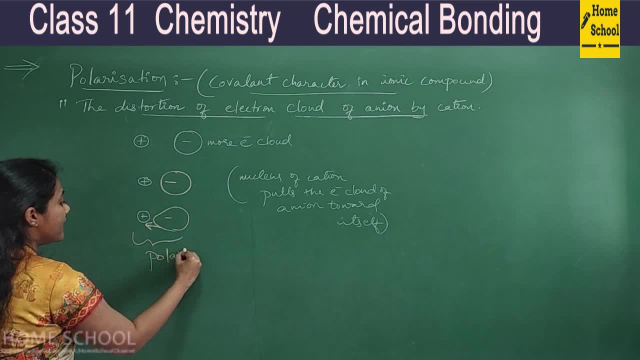 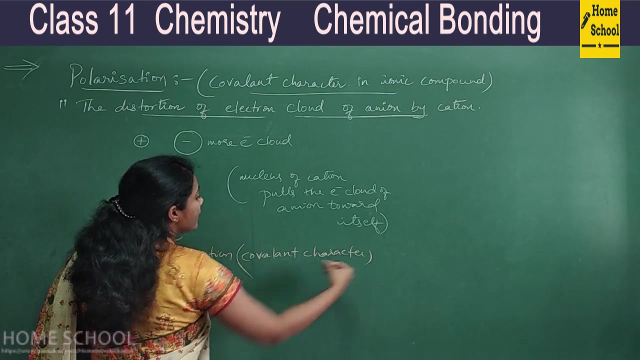 polarization. so this kind of distortion is called polarization. so once you observe the polarization, you know here the electron cloud is getting shared between this positive guy and negative guy. so more the polarization we say, more is the covalent character. okay, clear, so hope you understood. what do you mean by polarization? it is the distortion that is. 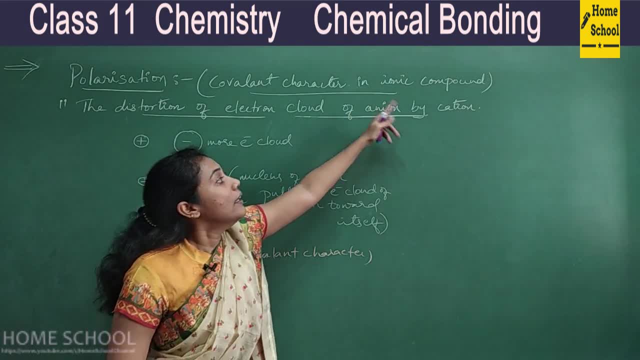 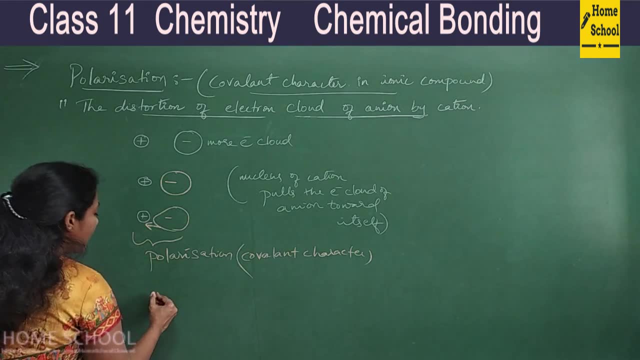 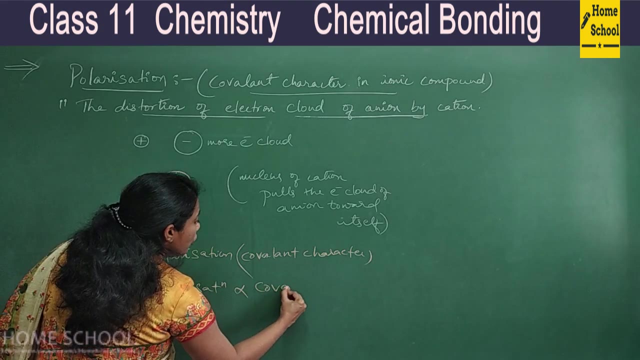 movement of electron cloud of anion by cation. okay, who is responsible for this distortion? It is the cation, right? So here our polarization. I can write: polarization is directly proportional to covalent character, right? So more the polarization, more the. 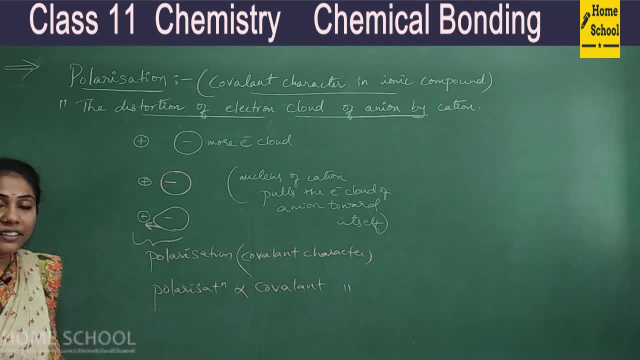 distortion you find more is the covalent character, right? So? and this polarization is inversely proportional to ionic character. When you find more polarization, ionic character is very very least okay. So that point also I can write here. polarization is inversely. 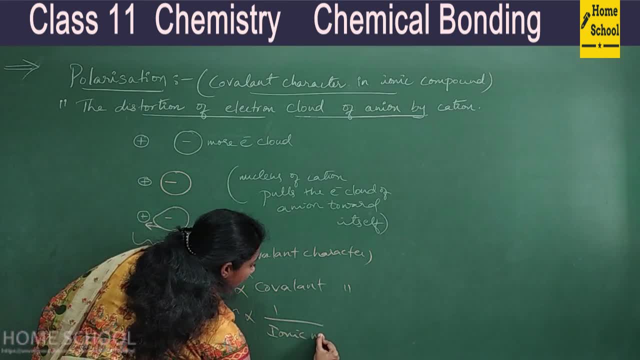 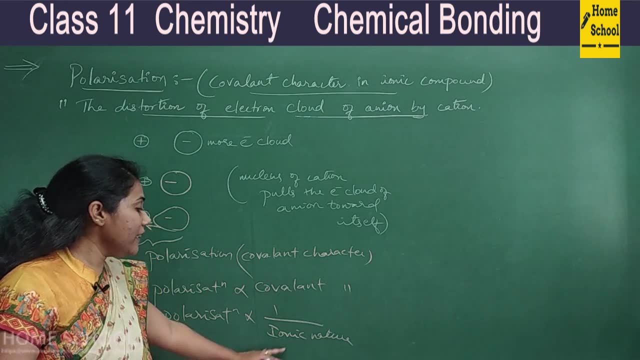 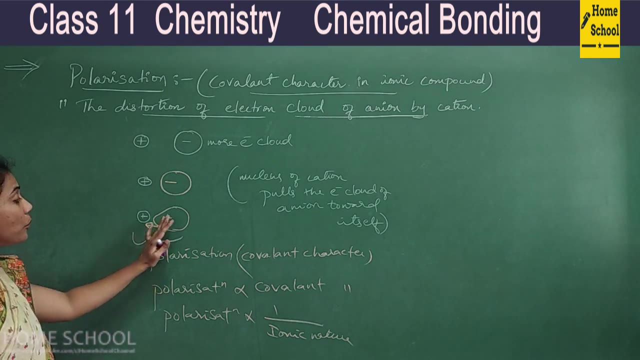 proportional to ionic character or ionic nature. okay. If covalent character is more, ionic nature will be less. okay, If ionic nature is more, covalent character will be less. right. So that way, So more the distortion you find, more the pull of electron cloud you find. 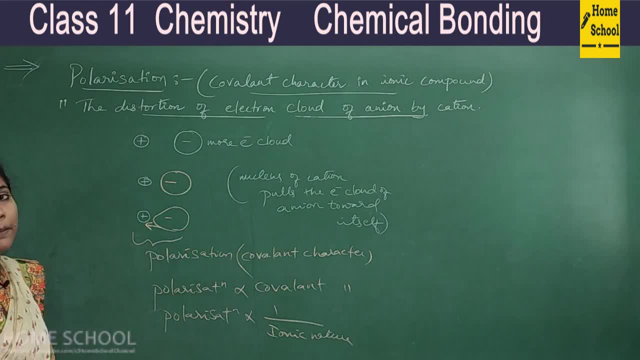 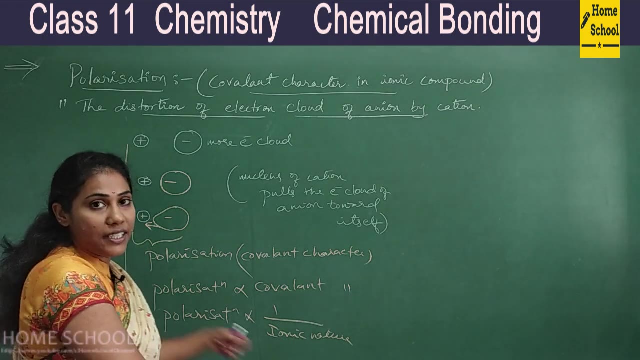 then more is the covalent character you will observe. So this is the reason behind why ionic bond has some amount of covalent character. okay, Fine, So here we will try to understand the meaning of certain words, right? So there is a word called polarizing power. 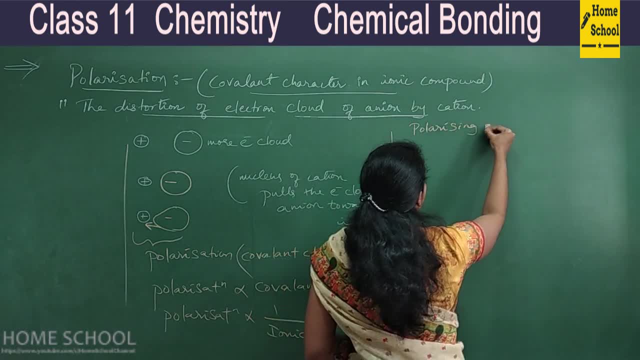 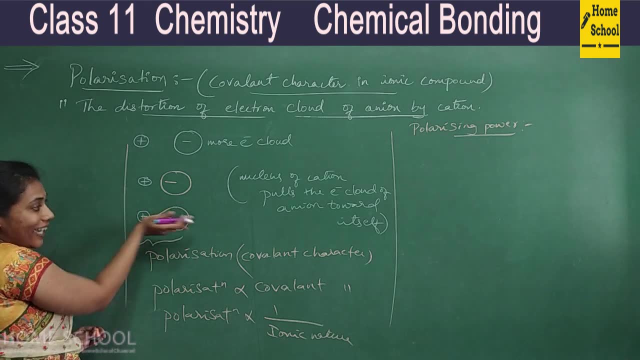 Polarizing power. So what do you mean by polarizing power? It is the ability of cation to pull the electron cloud towards itself. The cation must be more active. So if this guy is more active, then only it can pull the electron cloud towards itself. So the how much extent it? 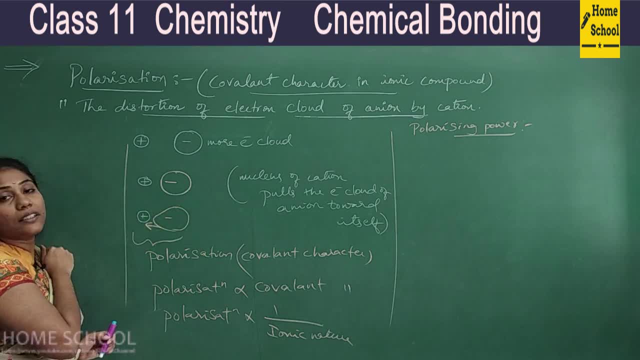 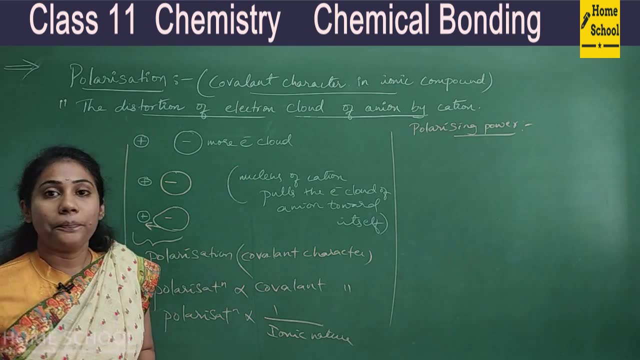 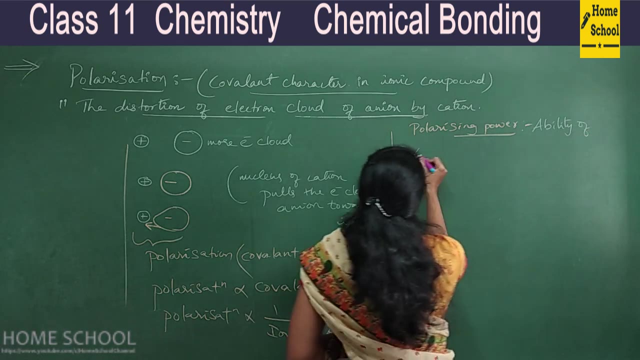 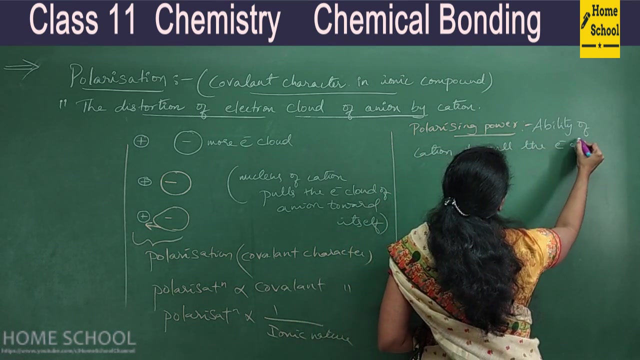 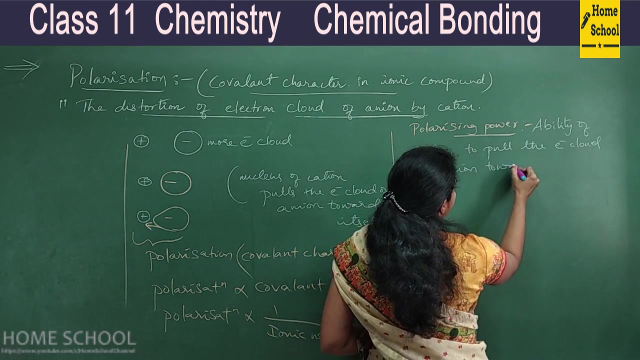 is active, how much capacity it has to pull the electron cloud towards itself. So that capacity of cation is called polarizing power. okay, So what I can write here- Ability, ability of cation, cation to pull, to pull the electron cloud of anion towards itself- is called, is called polarizing. 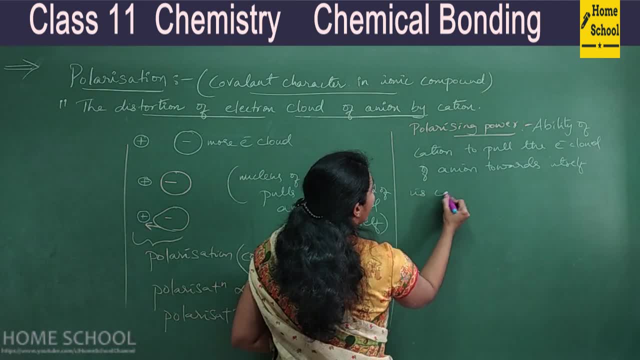 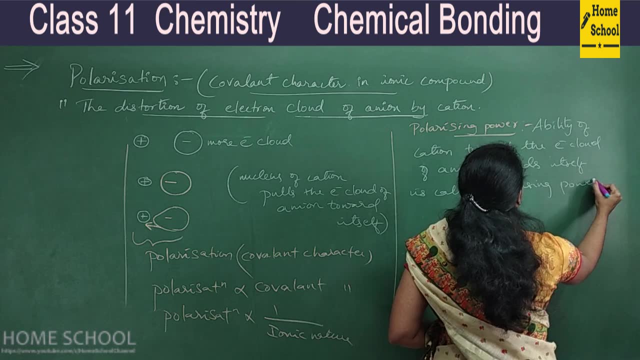 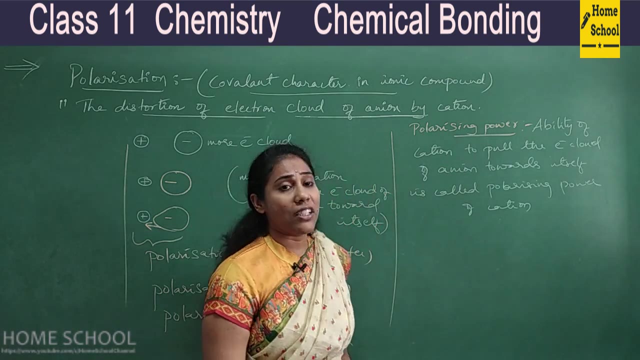 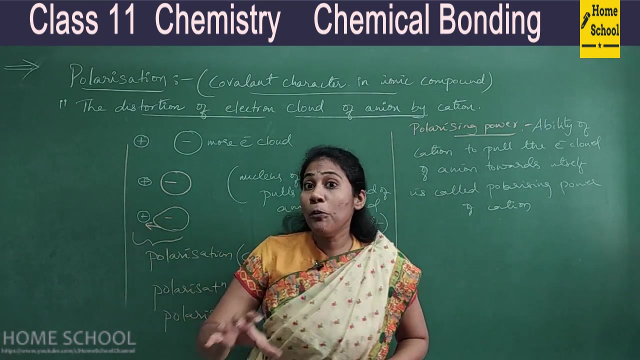 power of cation. okay, So is called polarizing power of power of cation. okay, So this is the meaning of the word polarizing power. So polarizing power is the capacity of cation With respect to cation, we will talk. okay, So how much is the cation is capable of pulling that? electron cloud towards itself. How much is the cation's capacity? How much is the cation's capacity? As we know, cation is mostly active, right? So if this cation is active then only it can pull. So polarizing power is the capacity of cation to pull the meal cation тоereal, optimistic viewers. So 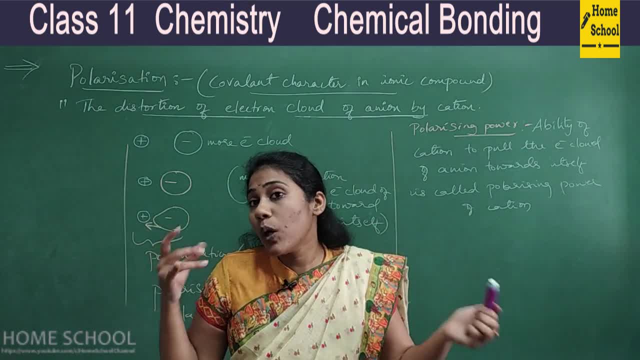 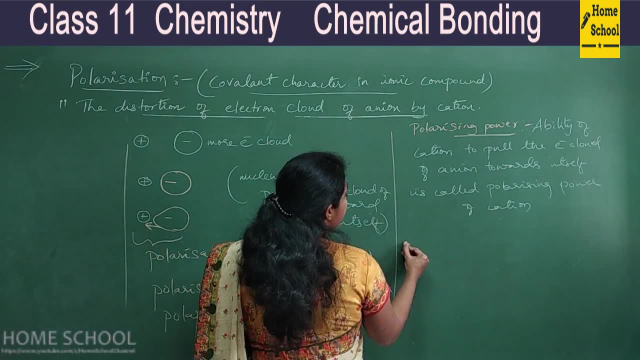 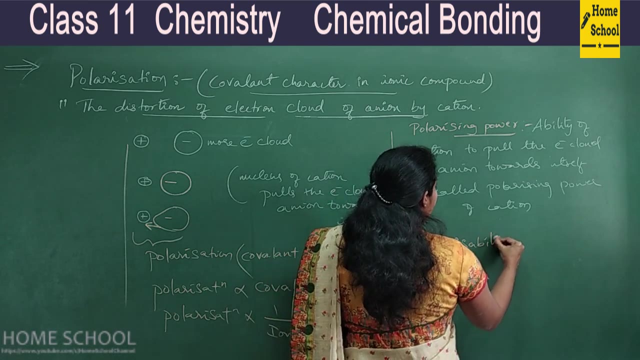 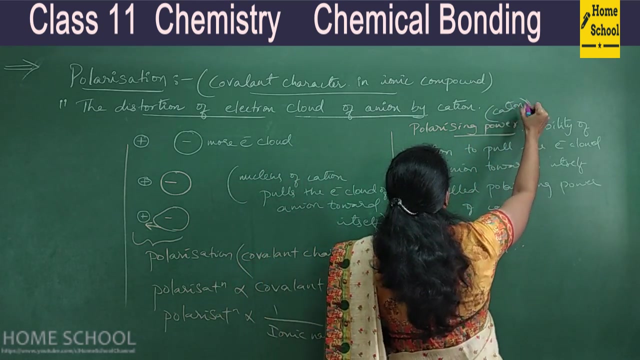 itself, so that capacity of cation is spoken in terms of, you know, polarizing power. and coming to another term that we have to concentrate, that is polarizing, polarizability, polarizability. so what do you mean by polarizability? polarizing power is something related to cation, and 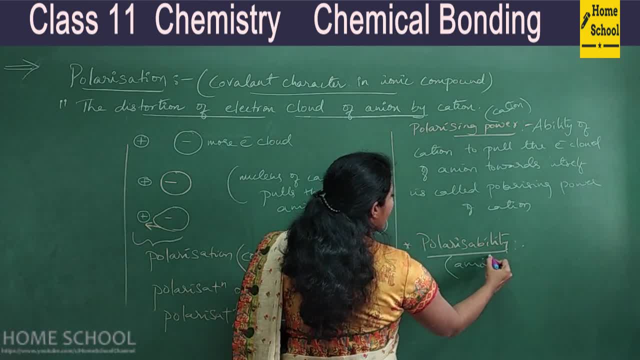 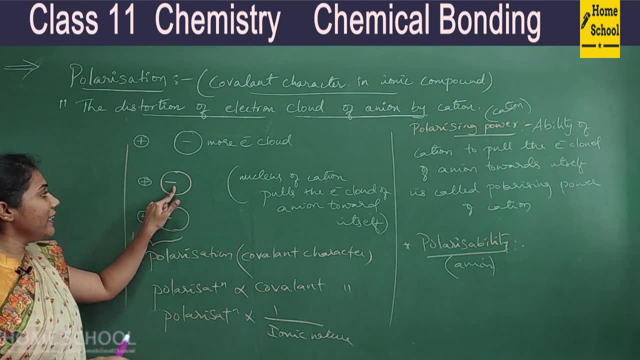 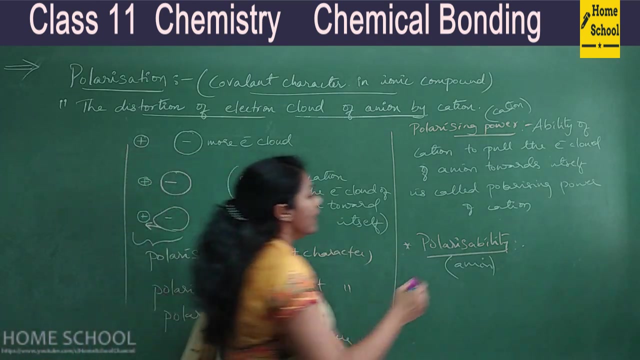 polarizability is something related to anion. okay, see to how much extent the electron cloud is going. say, if this guy is pulling, this guy must, must go. no, only then the distortion takes place. right, so the capacity of anion to go towards cation is called polarizability of anion. okay, so what is? 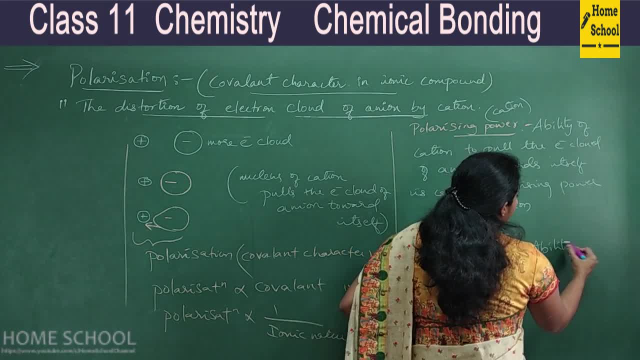 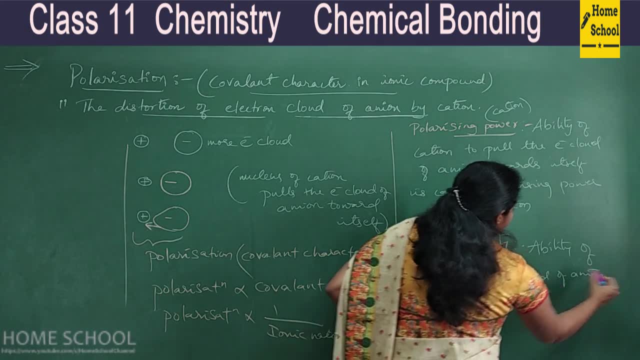 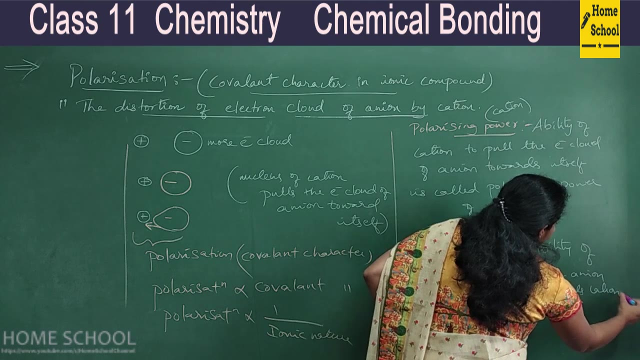 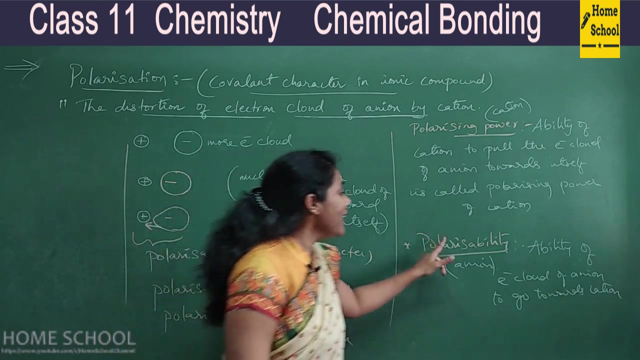 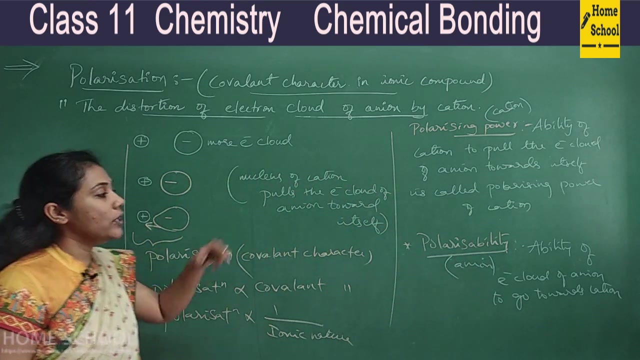 polarizability, ability of polarizability of anion, electron cloud of anion, anion to go towards, to go towards cation. i'm telling all this with the very simple words so that you can understand, so you can copy these definitions in your book. okay, so polarizability is the ability of anion to go towards. cation is called, you know, polarizability. 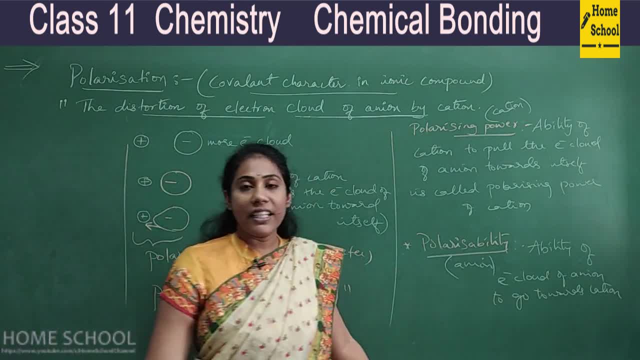 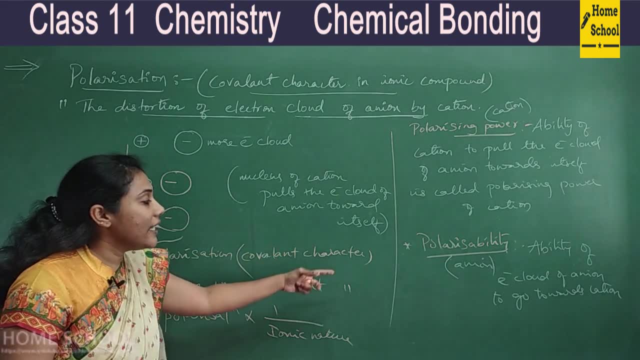 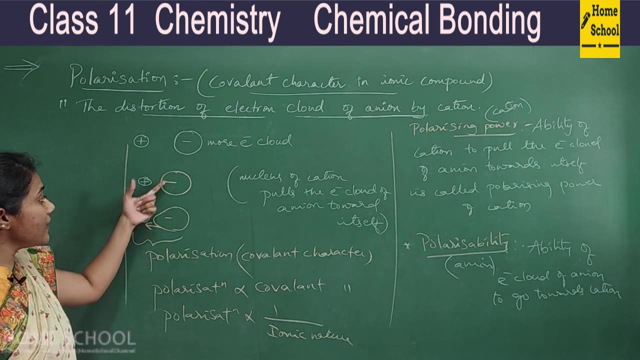 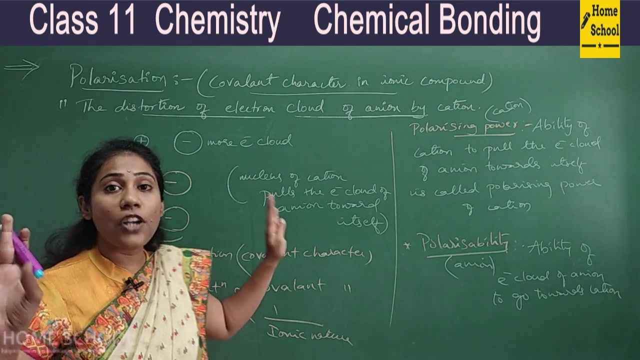 okay. so the meaning of polarizability is the ability of anion to go towards cation. teaching you jaffes. here are things. that problem of a field, polarization, can be observed in a better way if these conditions are satisfied. those conditions or rules for polarization is called phежд rule. so let us understand the rules of phage reason. so let us understand the rules of发Sab asence rule. 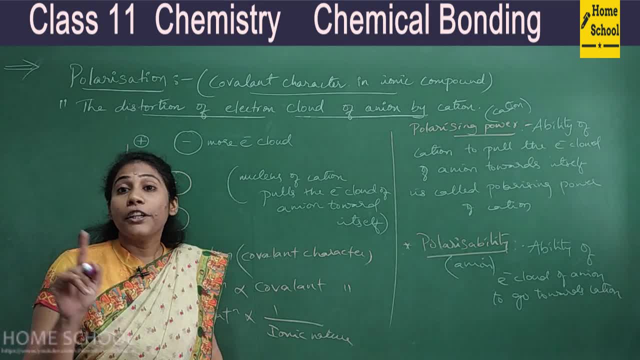 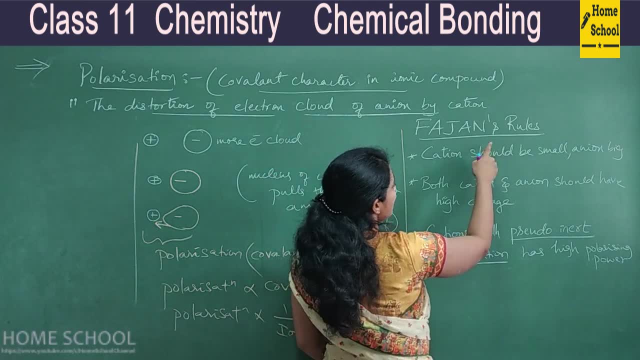 Поэтому hopes you have understood the rules of發 едов, so let us understand the rules of发上面mic phasens. see, there are three rules that you have to concentrate, three phasens rule, so phasens rule. 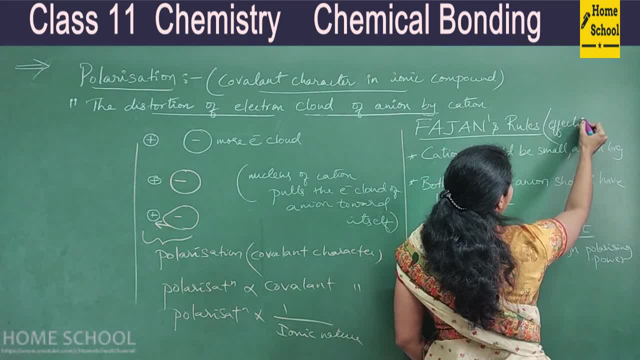 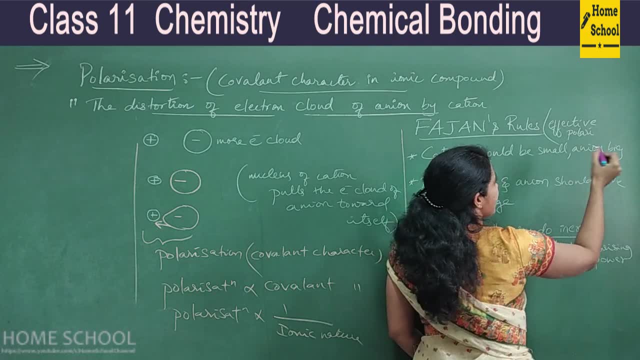 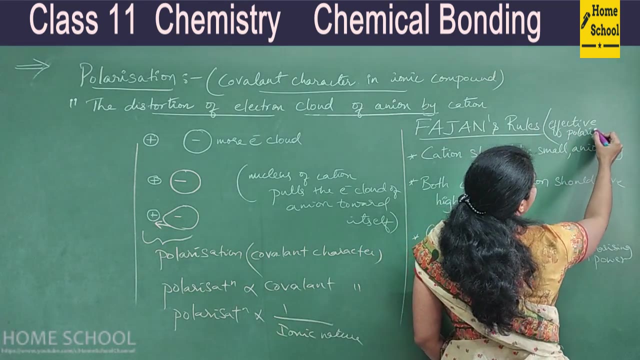 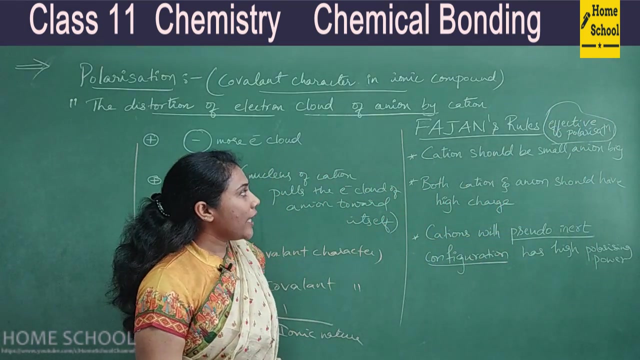 why we are studying for learning effective polarization. okay, so when do we decide that the polarization is maximum? you know to understand that we have some conditions and rules, you know. so those rules are our phasens rule. okay, learning for effective polarization. fine, look at the first rule that i have written on a board: cation should be small, anion should be. 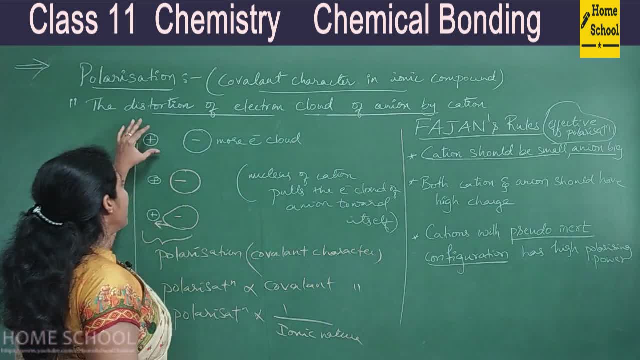 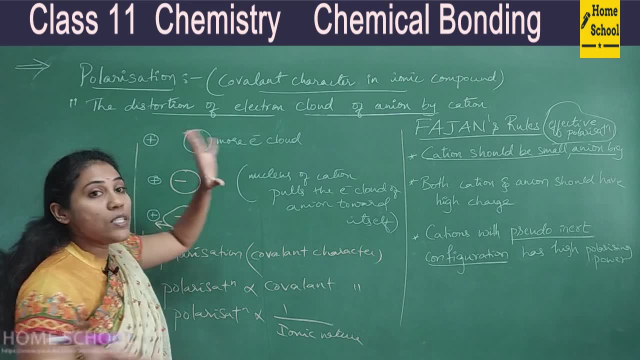 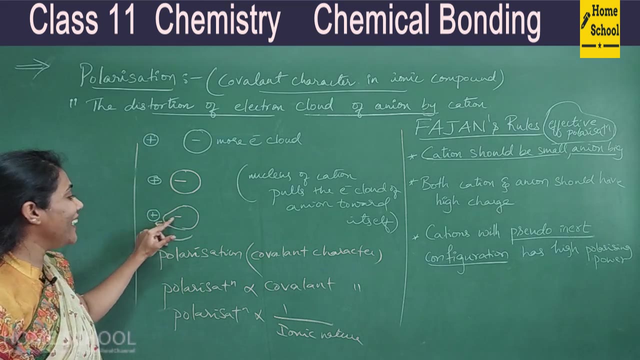 big. okay, see, any ionic bond is formed with cation and anion, right, whenever cation is very small, anion is very big, then the polarization, this distortion of, uh, you know, anion will be maximum. okay, so that is what the meaning of first rule, cation. 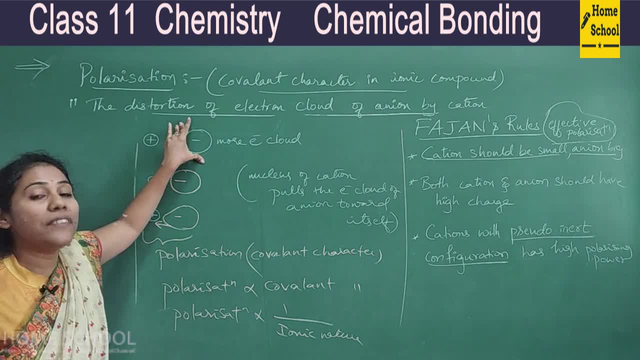 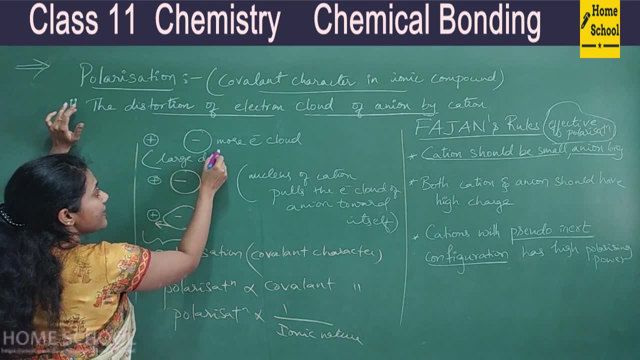 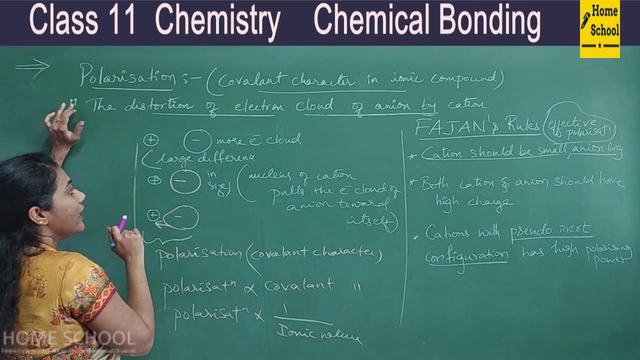 must be very, very small. anion must be very, very big. in other words, i can say that there should be a large difference in size. there should be a large difference in size. there should not be a comparable sizes. okay, so anion too much, because cation. 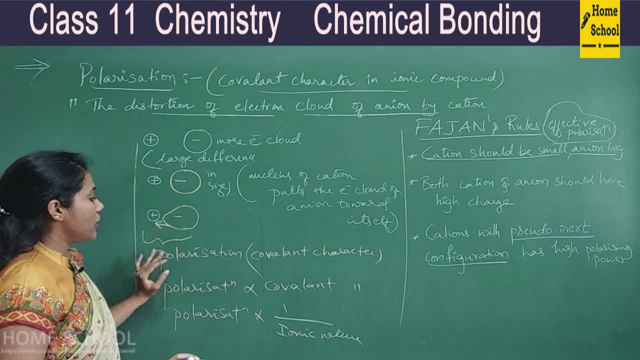 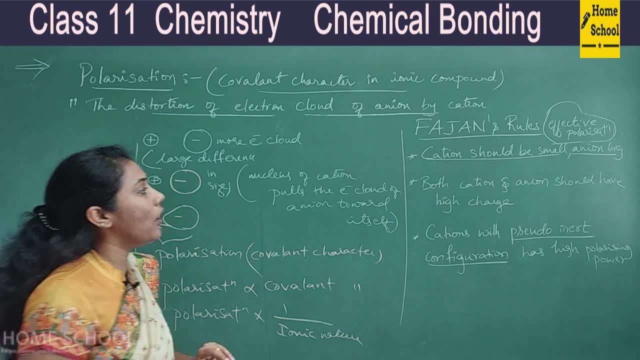 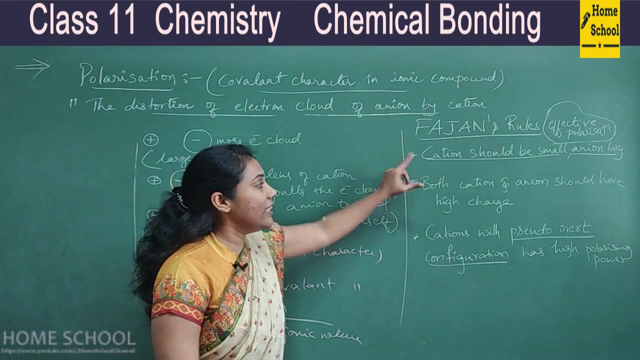 much small, then you will observe more distortion, that is, more polarization, more covalent character. so to observe more covalent character in ionic bond, cation should be very, very small. anion must be very, very big, right, very, very important condition, guys. coming to second one, both cation. 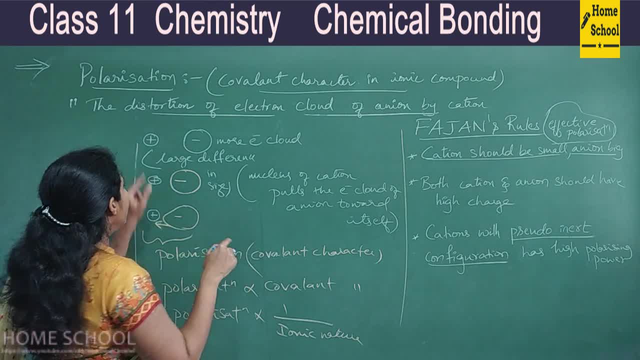 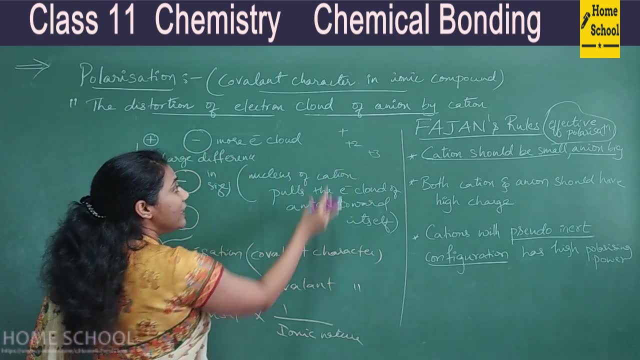 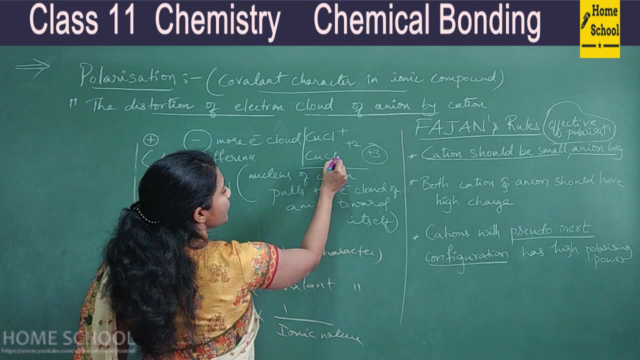 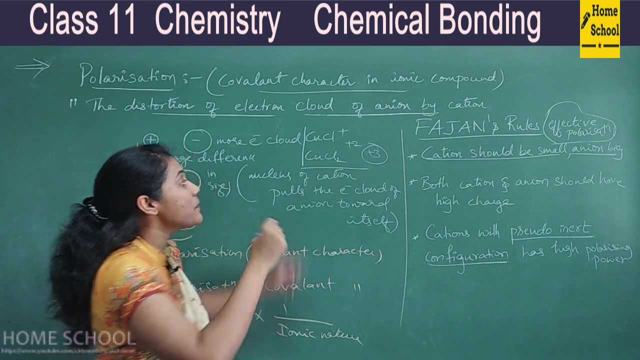 and anion should have high charge. okay, see, cations can have a charge. it can have plus one, it can have plus two, it can have plus three. so it is better if cation has high charge. suppose you have two compounds: one is cucl, other one is cucl2. okay, if i ask you, among cucl and cucl2, which one is more? 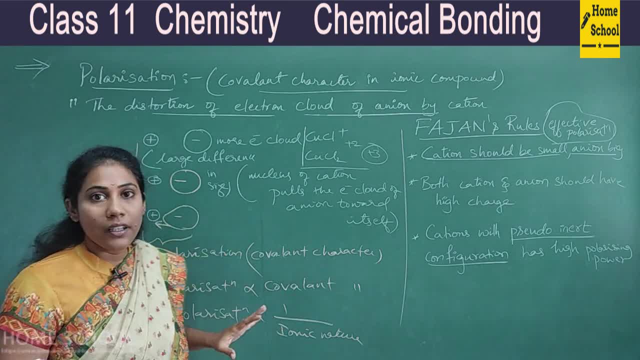 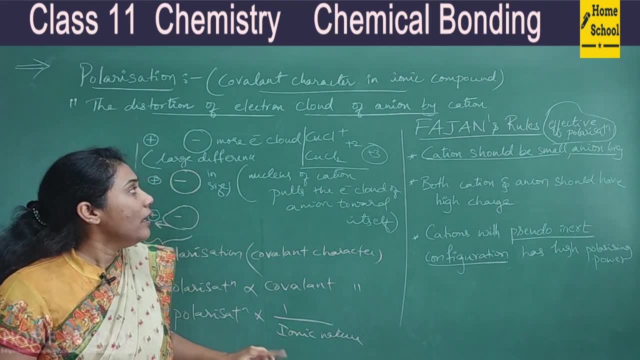 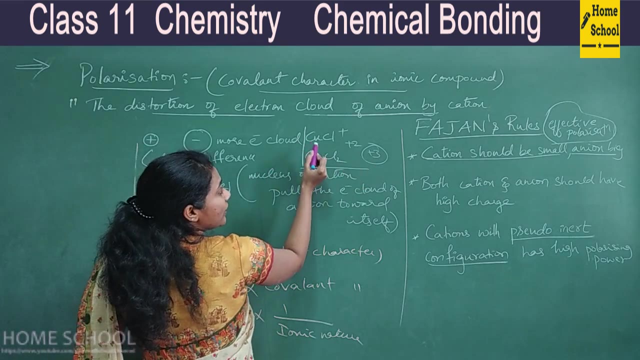 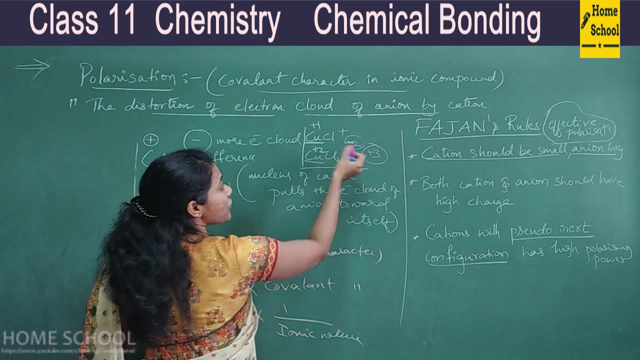 covalent. both are actually ionic compounds, right, so they have covalent character. both have more covalent character only actually speaking. but among them, which one has more covalent characters? so how do you decide? check based on the charge, here the copper's charges plus one. here the copper's charge is plus two. so more the charge, more is the covalent. 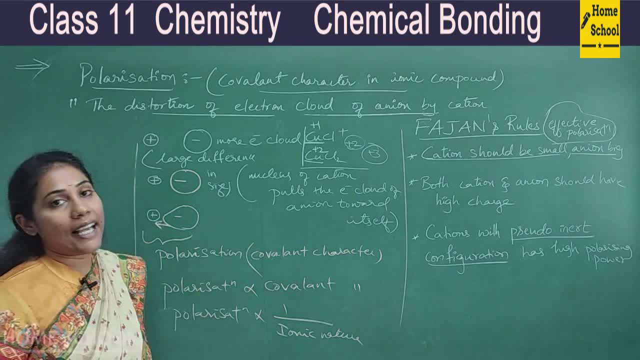 nature. okay, so this works out for both cation and anion. anion case minus one minus two, minus three, so more the charge, more the covalent nature. okay, so this works out for both cation and anionً case minus one minus two, minus three, so more the charge, more the cation. meaning Legend arm華, negative carbon derm hundred minus two, certain kind of a regular basis ofived chemistry. that Village ev muchís früh. 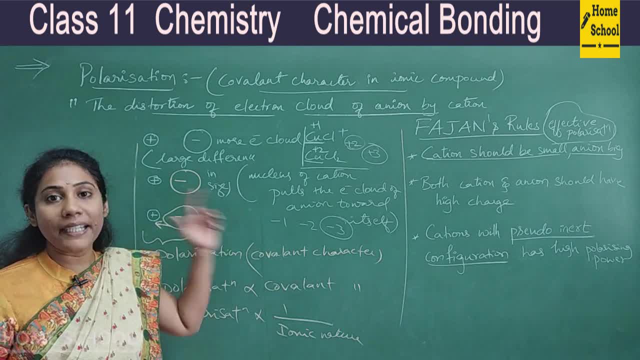 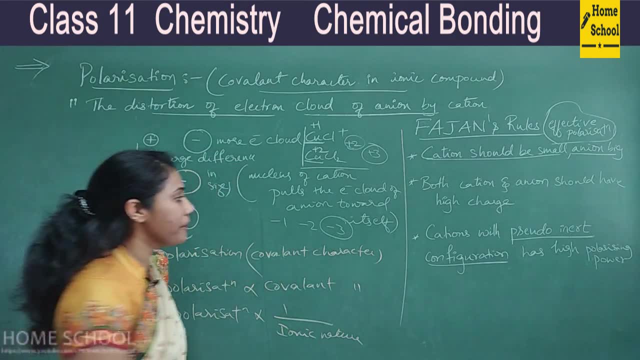 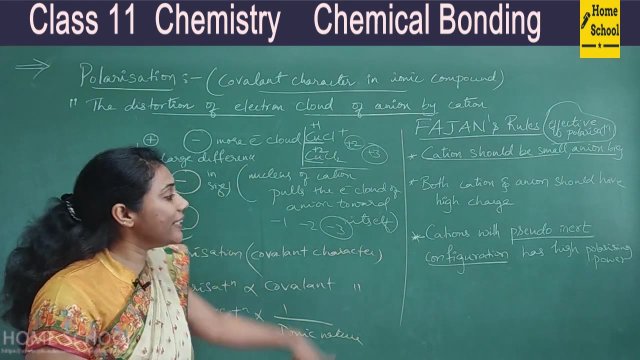 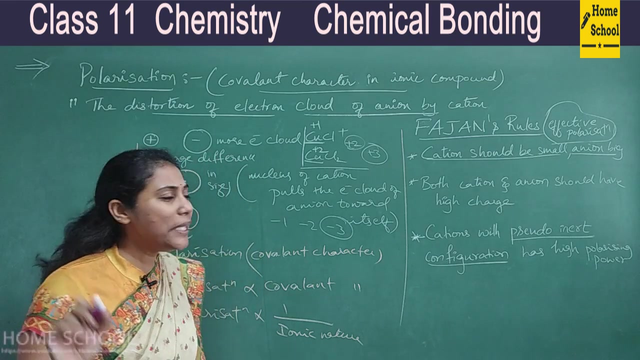 is the polarizing bubble. okay. so to observe better polarization, you know both cation and anion should have high charges. right coming to last point, this is very, very important to understand- you will observe better polarization when cations have pseudo inert configuration. so what do you? 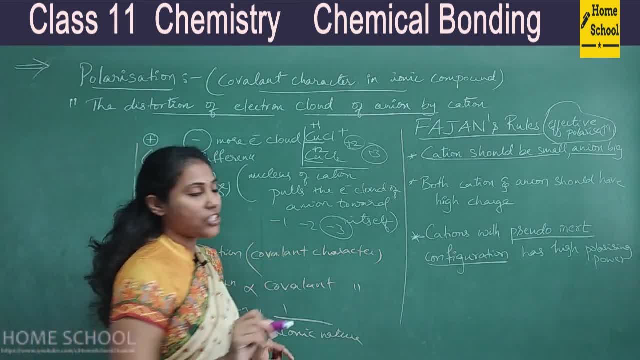 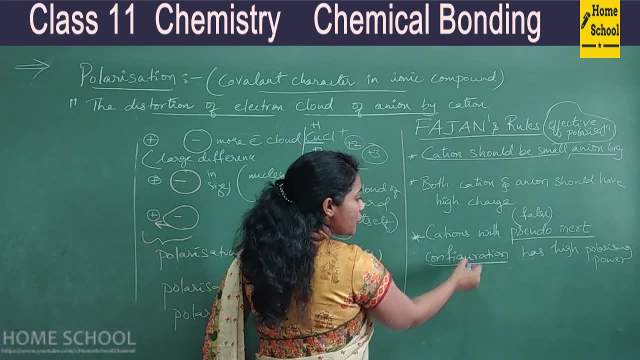 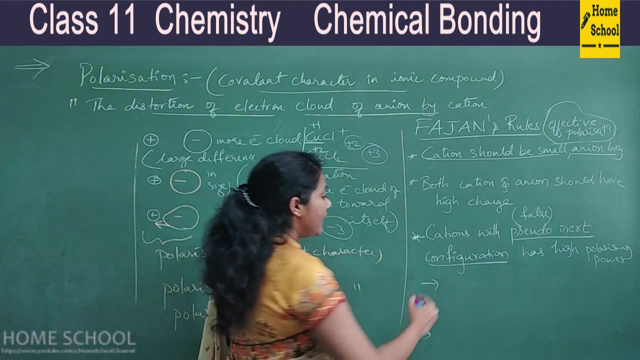 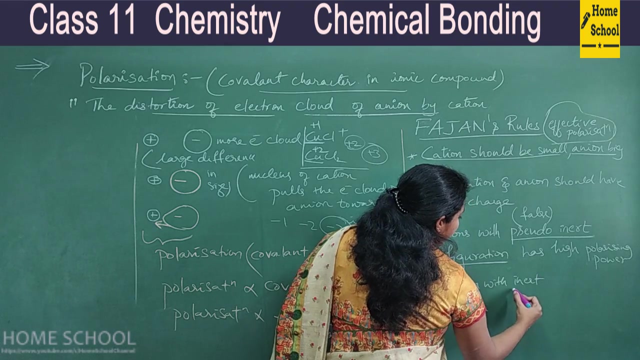 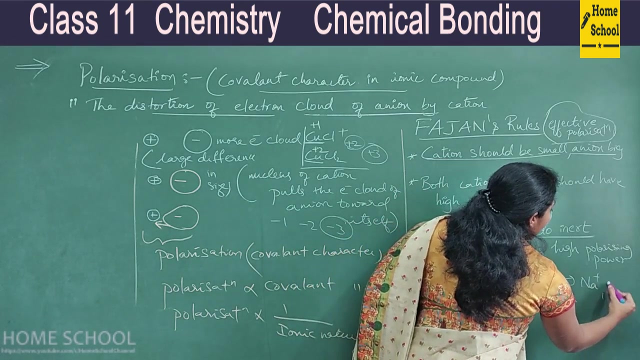 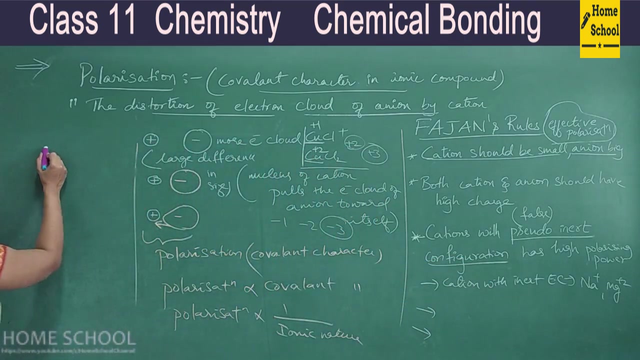 mean by the word pseudo inert configuration. the meaning of the word pseudo means false, right see. based on this point i can divide cations into three categories actually cations: cations with inert electronic configuration. inert easy means electronic configuration. okay, see na p plus mg plus two. these are examples. say na plus, you see here, na plus, what is its electronic? 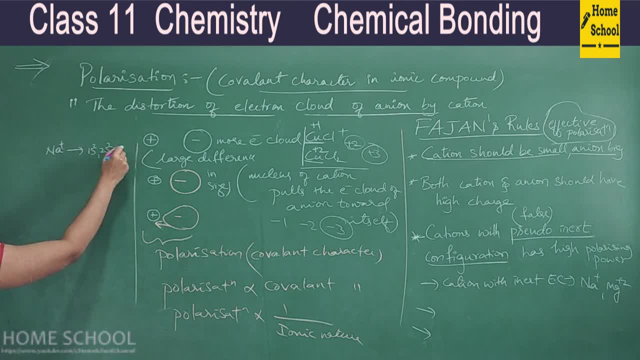 configuration: 1s2, 2s2, 2p6- right? so this is the electronic configuration of inert gas. that is neon, right? so here na plus has exact inert gas electronic configuration. this is a electronic configuration of neon, so na plus is actually showing exact electronic configuration. 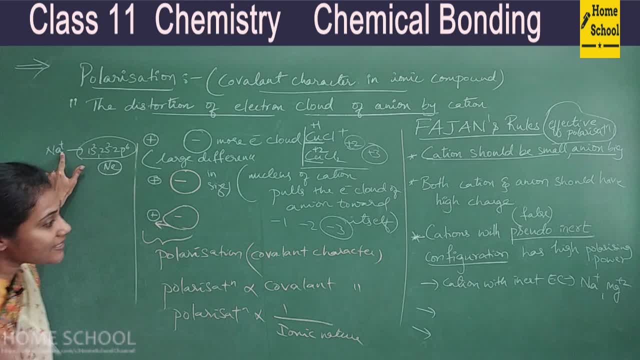 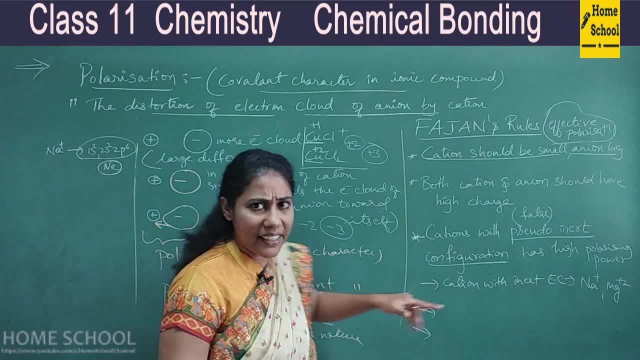 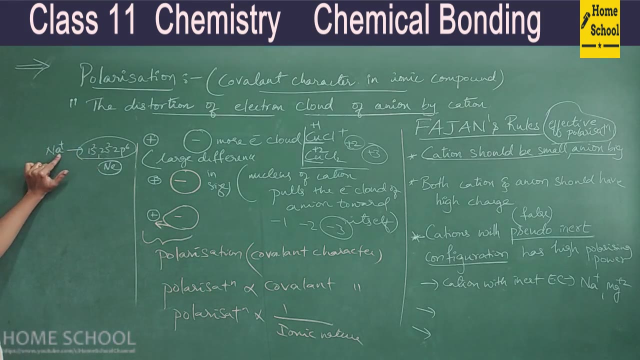 as that of neon. so that is why na plus is called cation with inert electronic configuration, inert, not pseudo inert. exact n a plus electronic configuration is exactly similar to inert gas. so i call na plus as cation with exact inert gas electronic configuration. okay, say likewise: mg plus 2 exact inert gas electronic configuration. it will show right. so na plus mg. 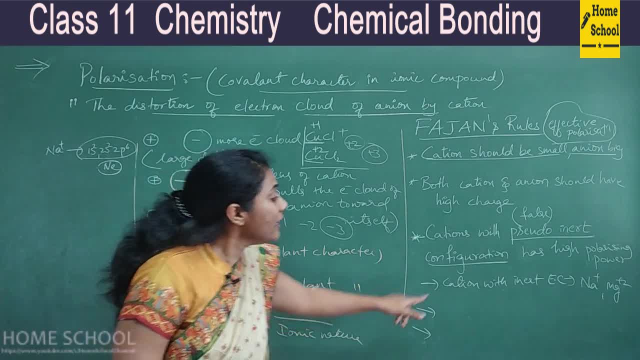 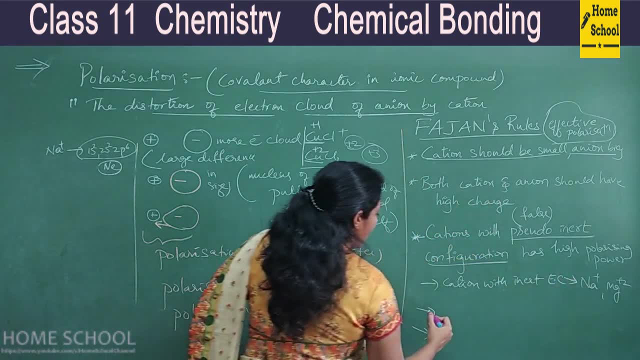 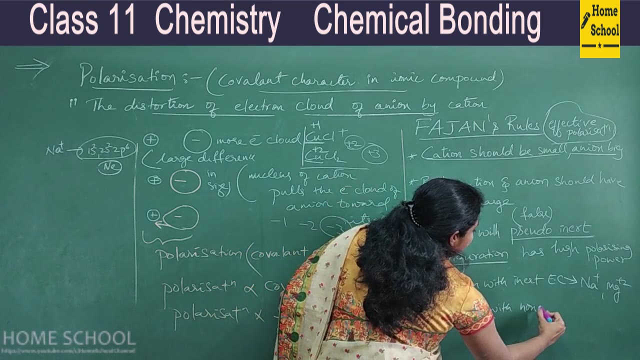 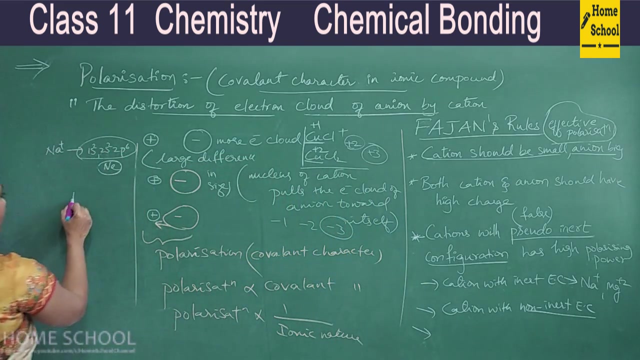 plus 2 al plus 3, all of them come under cation with inert electronic configuration- okay. and the other type of cation you see, cation with cation with non inert electronic configuration, okay. say lead, if you take up lead ion, you know it will not show. you know inert gas electronic. 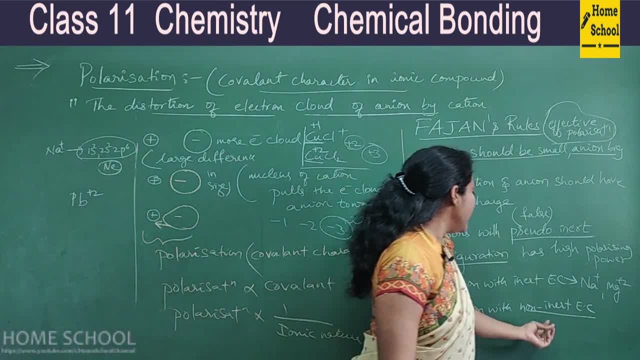 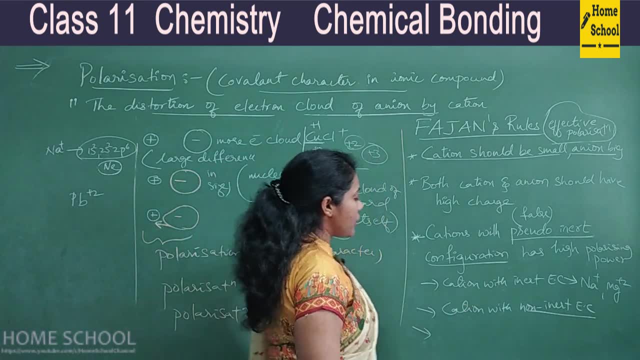 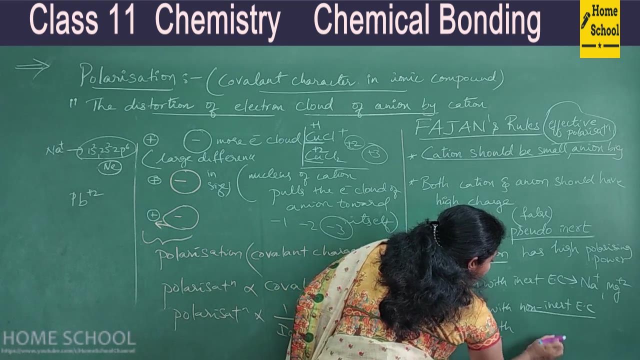 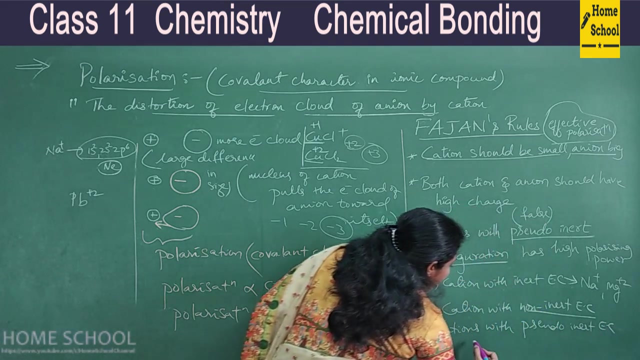 configuration right. so such cations are called non inert electronic configuration. showing cations right. and coming to third category, which is very important, cations with pseudo inert, pseudo pseudo inert electronic configuration. example for this is zn plus 2, cu plus ag plus- okay, so all of them will come. cadmium: okay, so cadmium plus 2 will come. you know all. 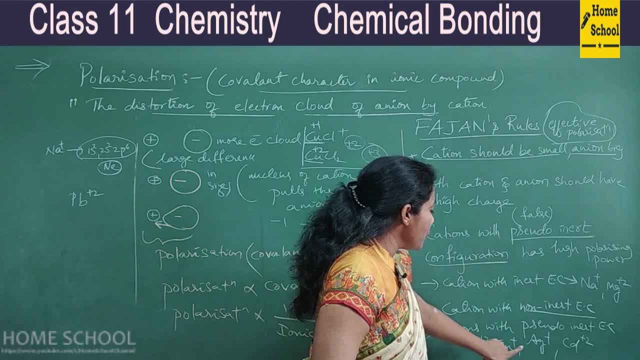 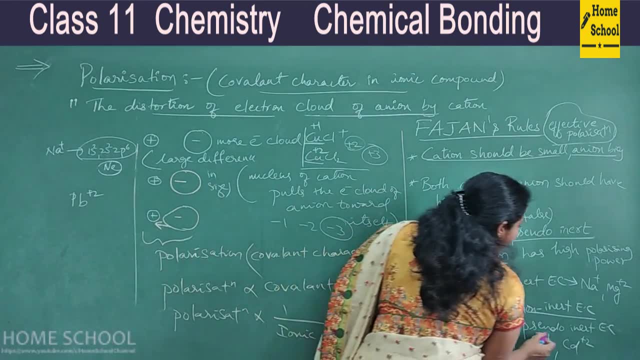 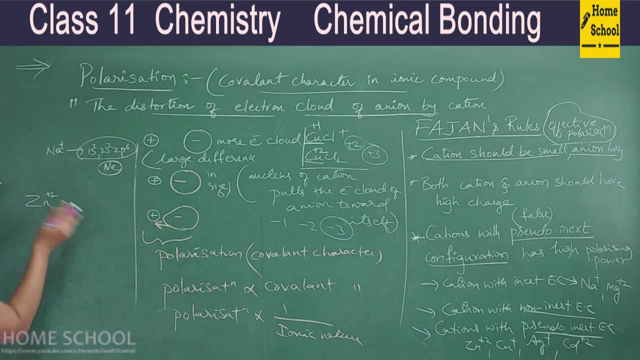 these d block elements, especially zinc plus 2, cu plus 2, ag plus 2, cd plus 2, all of them will come. so let me tell you what is this pseudo inert electronic configuration beta? good, you see, there are two exactly role models in this category. 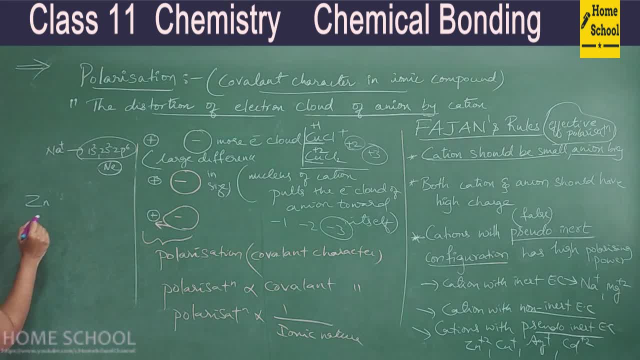 you know it's not in space N, why not? you can see λ x is minus 1 for delta x. then bequ topic for this professor in the second level. okay, you can see it is sander- cannot come down to this setting because if it will be below this setting, 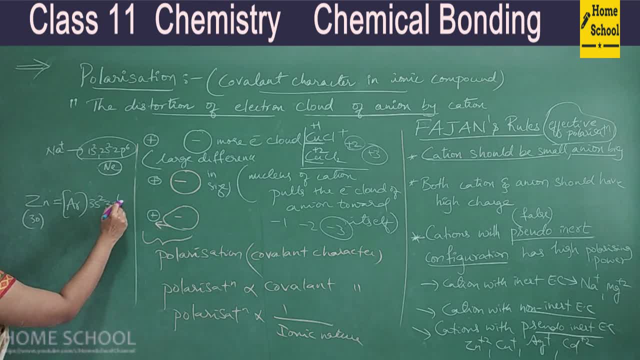 then ventral pressure will only get Fifunurate to that section and then the person other always wants to join the formation because 좋은. so observe another 4s2, okay, 3d10, okay, zn plus 2. electronic configuration is how much argon, 3s2, 3p6, these electrons? last shell means fourth shell, so in this shell two electrons. if 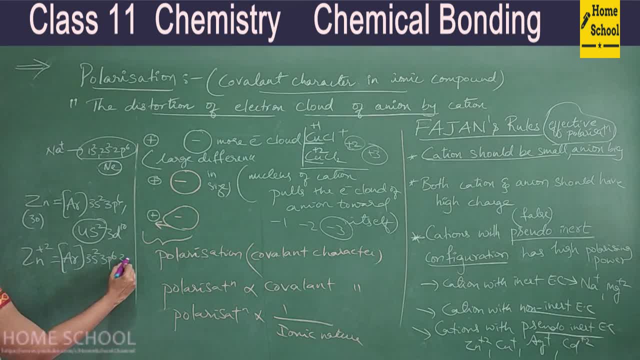 it loses, it becomes zn plus 2, so its electronic configuration is 3d10. so this is not same as any noble gas electronic configuration. this electronic configuration is not similar as any noble gas electronic configuration, but this is stable. only this is stable itself. you see all. 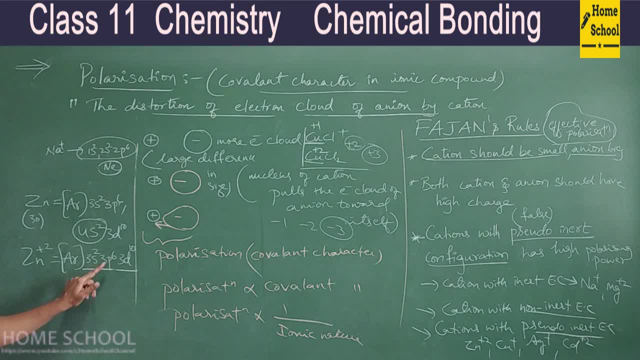 orbitals are completely filled: s orbital with 2 electron, p orbital with 6, 3 orbital with 10. that means our third shell is completely filled with 18 electron. okay, so our third shell is completely filled with 18 electron. it is completely stable, but electronic configuration is not similar electronic. 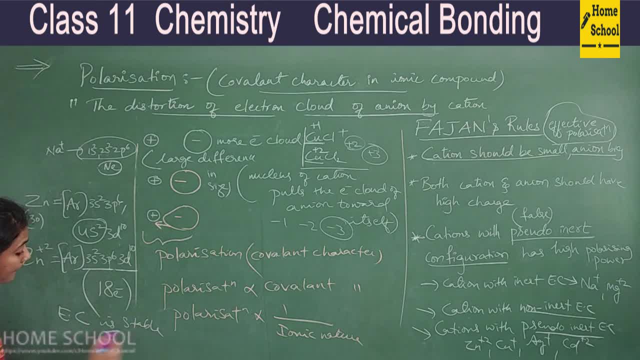 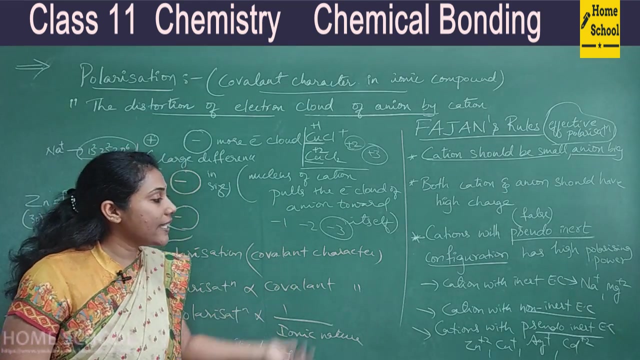 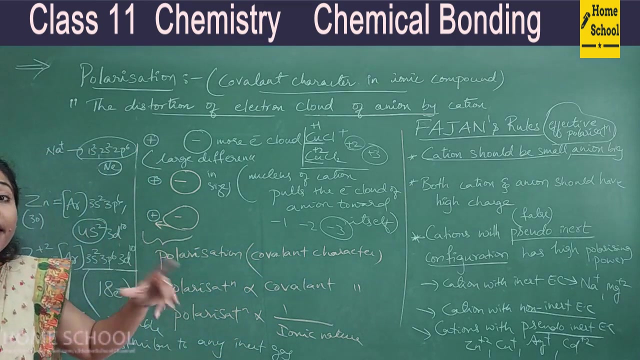 configuration is stable, right, but not similar to, but not similar to any noble gas, any inert gas, right. so such a configuration, electronic configuration, is called pseudo, pseudo, pseudo, pseudo, pseudo, pseudo, Inaut electronic configuration. okay, so usually try to remember zn plus two, copper plus cu plus ag plus cd plus two, all these cations, if they are there in a compound they will show more. 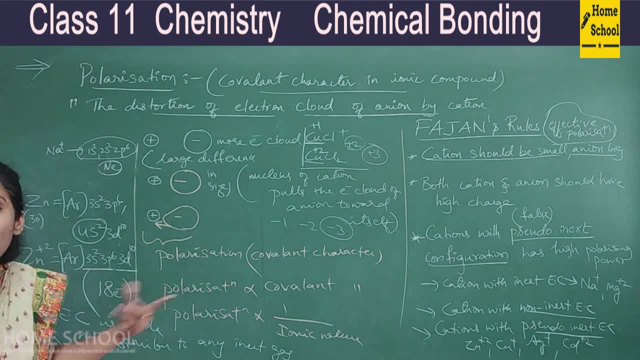 polarization: okay, they will have more polarizing power, so that's why those compounds will have more covalent character. okay, so these three points are very, very important to understand. some key points we need to understand. okay, say, for example, question can be asked this way: now let us work it out with. 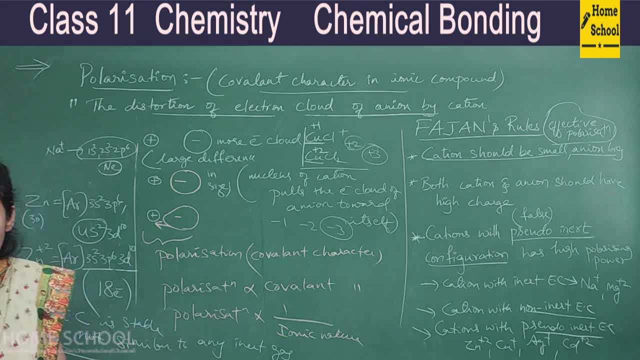 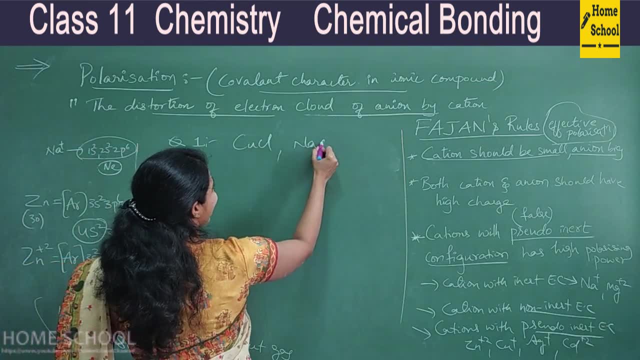 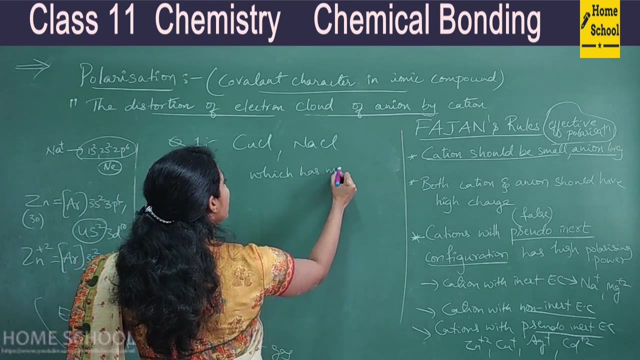 few questions so that you will get a clarity what actually I'm talking about. look at the first question. you have cu, cl and enacl, okay, so my question is: which has more? which has more covalent character? which has more covalent character? which has more covalent character? 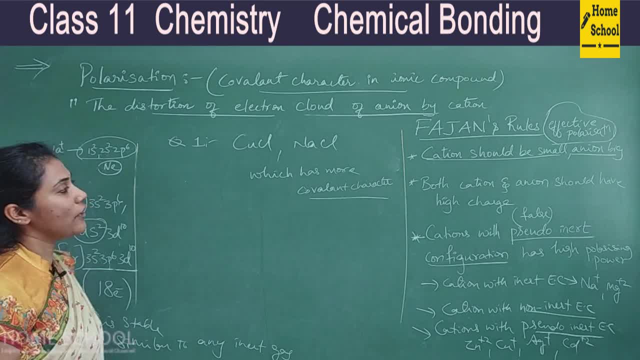 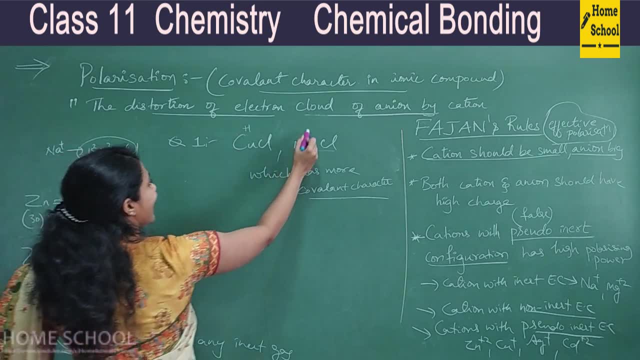 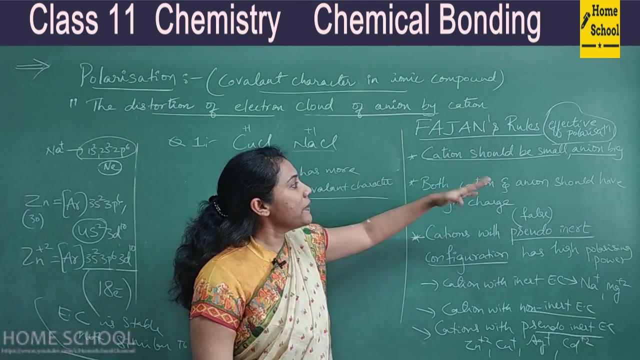 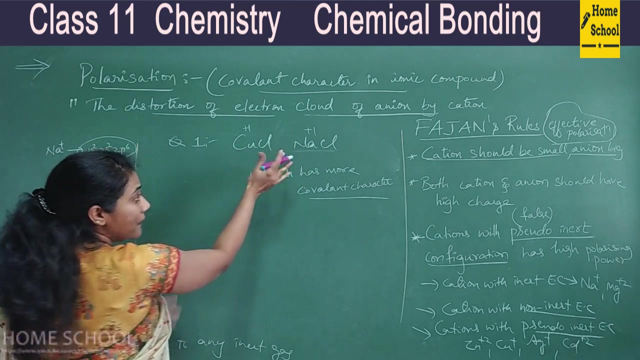 okay. so this is the question. so how do you decide? copper chloride, na plus here copper's charge is plus 1, na's charge is also plus 1, okay, so based on the charge, you can't decide. and cation should be small, anion should be weak, right? so normally bigger cation, say compared to copper sodium, comes. 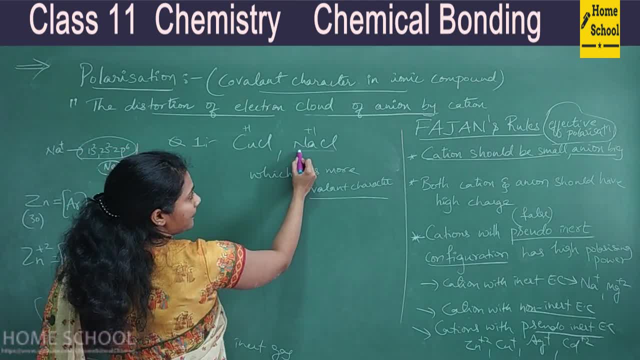 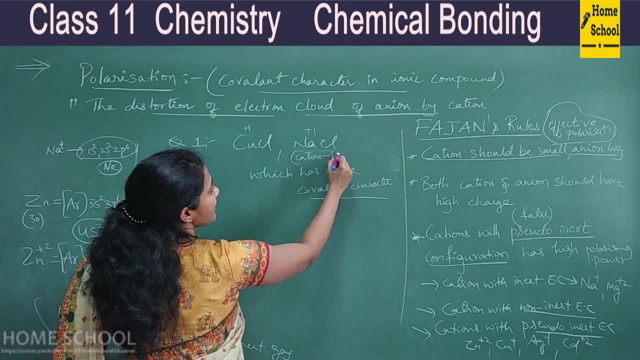 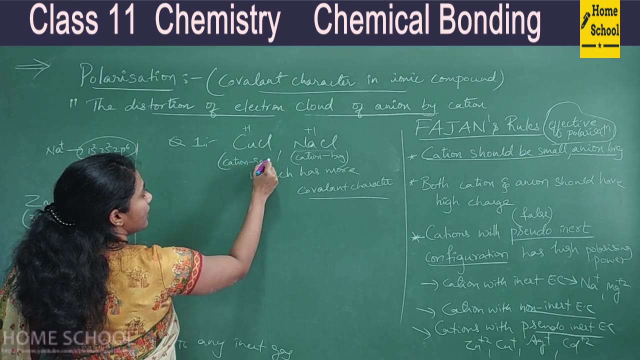 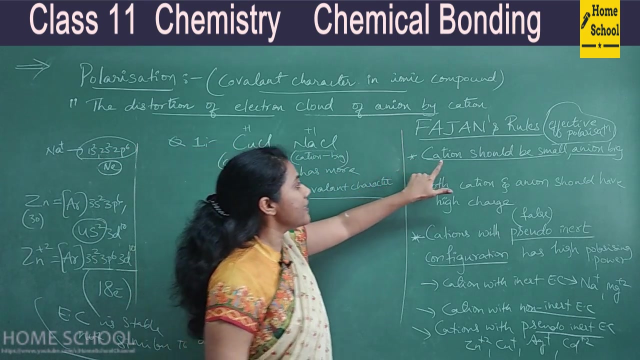 in the first group. so you know, this is sodium- is comparatively big cation. actually speaking, this is cation which is big, whereas this cation, this cation, is actually small. okay, so this is the small cation and this is the big cation. what it the point says, cation should be small, anion should. 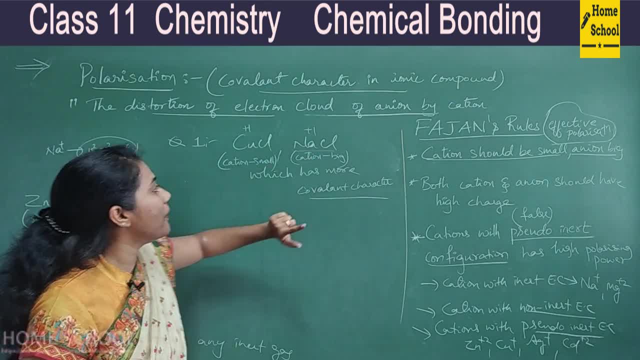 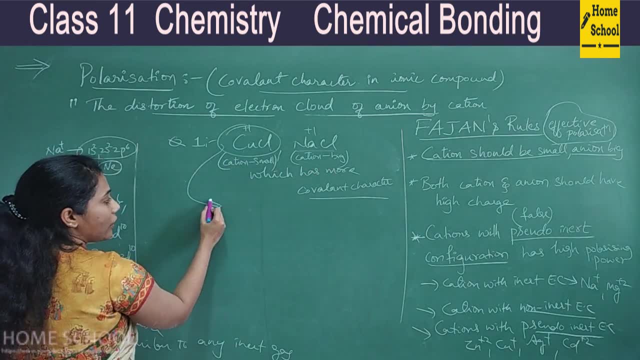 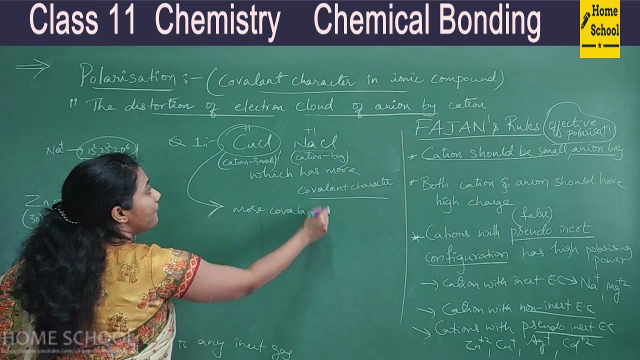 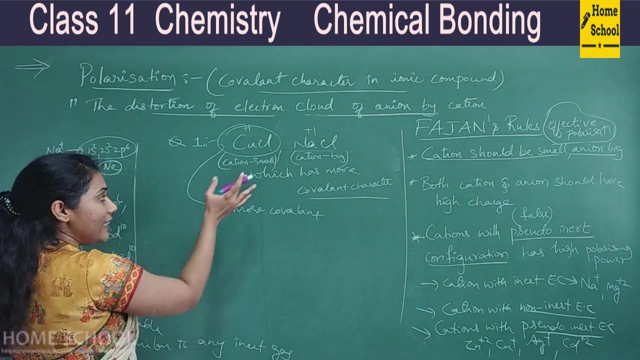 be big. so anion is common in both the compounds, whereas cation copper is small, sodium is big. so we can say: copper chloride, copper chloride is more covalent, isn't it? because compared to sodium, copper is smaller. cation sodium is big, we know. first group elements are bigger. right, and that is one point you can concentrate. 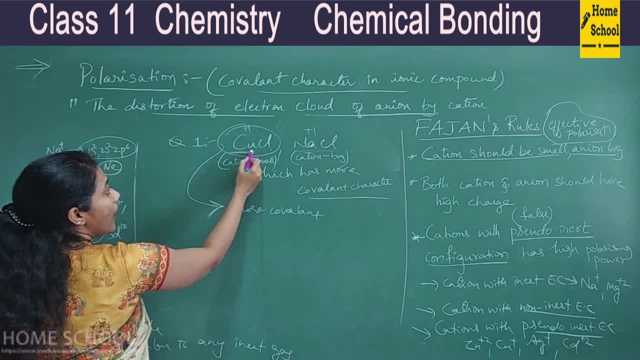 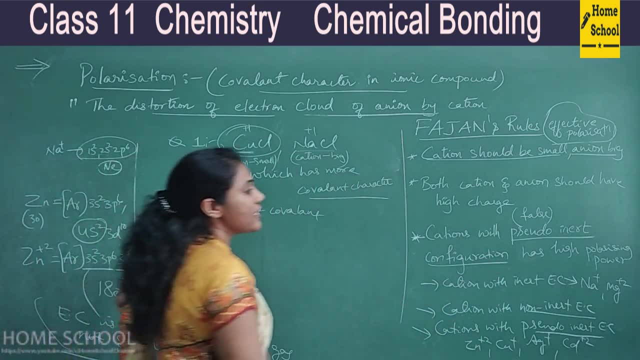 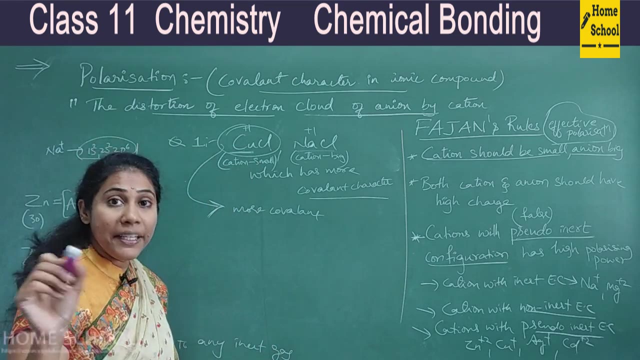 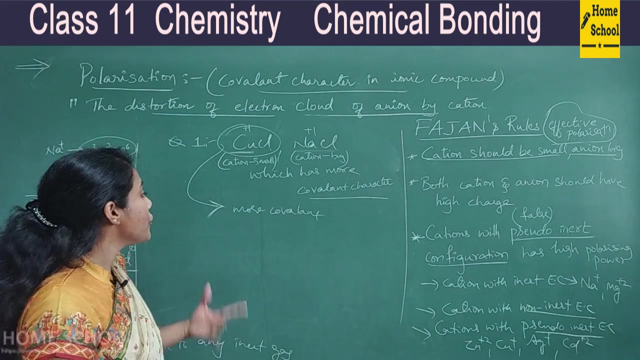 then the other point, looking at this copper, what is copper? copper is cation, cation with pseudo inert electronic configuration. what is our third point says: cations with the pseudo inert configuration have high polarizing power, high polarizing power, high polarization, high polarization, more covalent character, isn't it so? based on this point also, whenever you find 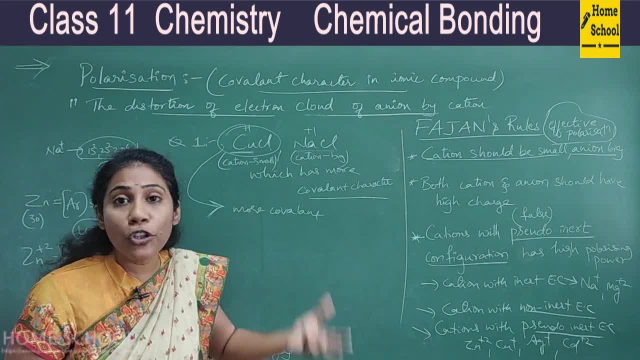 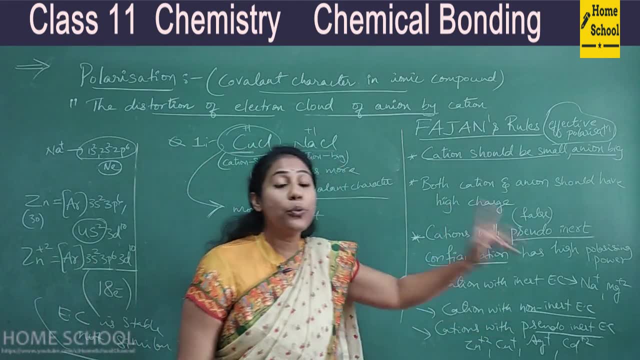 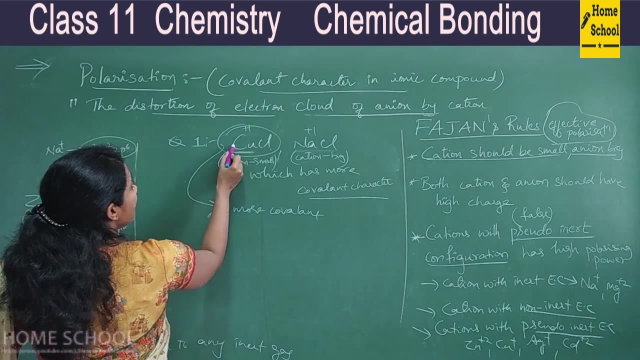 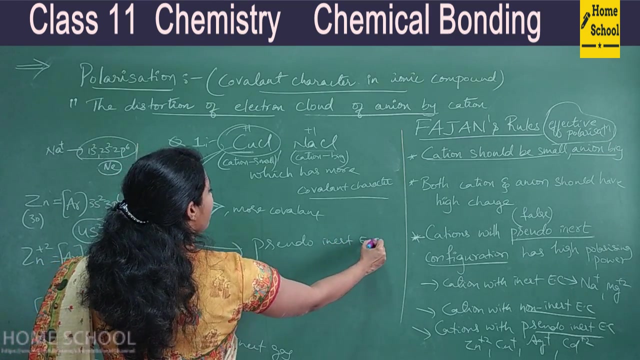 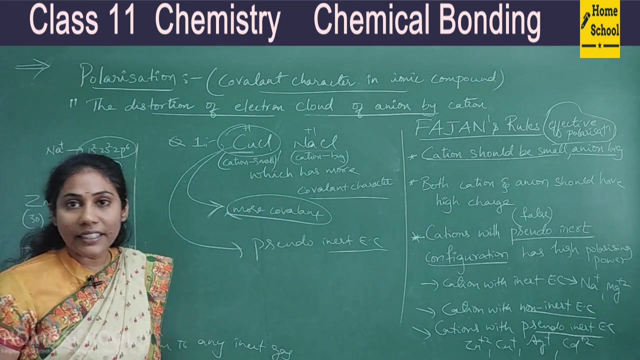 these cations. definitely they have more covalent character because all these cations will come under the cations with pseudo electronic configuration. so one is size is small. the other reason is what this particular copper has: pseudo, pseudo inert electronic configuration. so that is why you know this copper chloride has more covalent character, clear. so this. is how you can decide, like among a given compounds which one is more covalent character. so if you see that copper wasило- NO, Sette Schorr observations- those copper chloridesnic here were more covalent because they were both separate configurations. you know they were not. 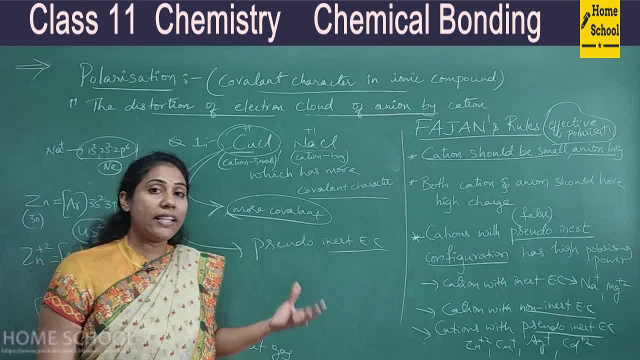 different aspects. they were both also dichromasterized, very differentiate likeンet they were not Because of a relativeSí ofнеciation. if A zero, one is the nanomamm concrete, all the two sayc anyways covalent, and which one is less covalent. So this is one important type of question. 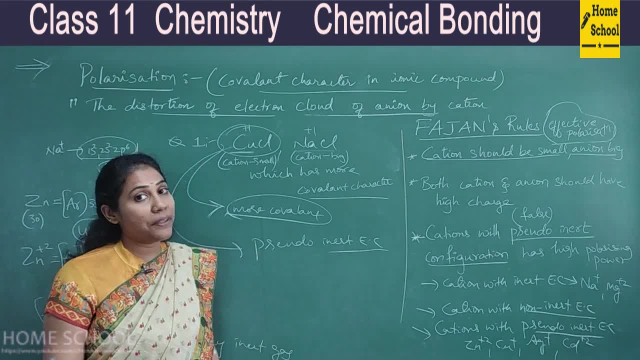 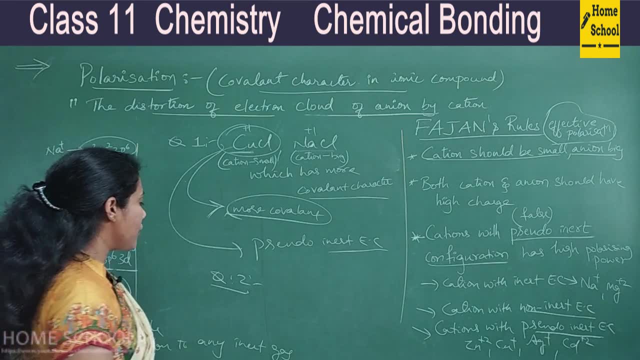 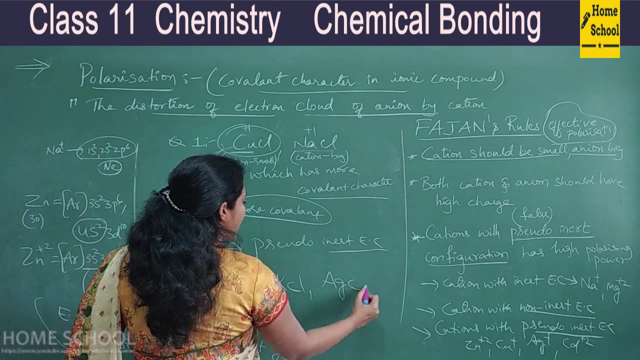 for your competitive examinations. So you have to be very, very careful. and coming to second question, for this you are giving answer in a comment section, So please try this. you have KCL and you also have AGCL, So tell me which one has more covalent character. My question is: 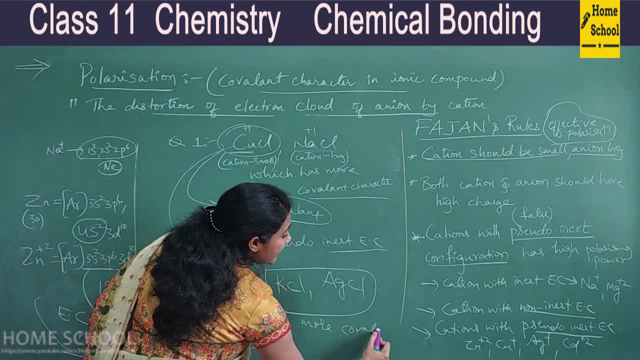 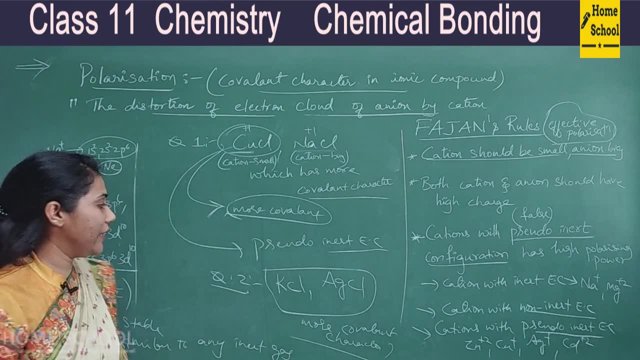 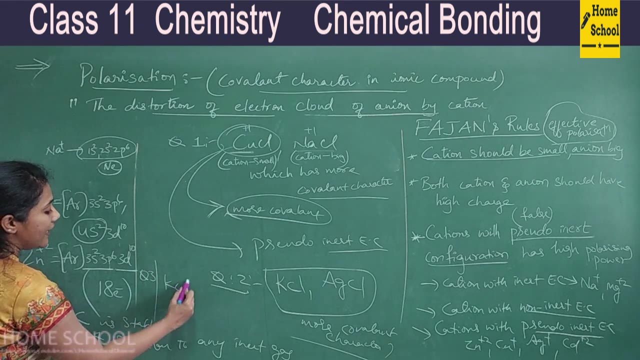 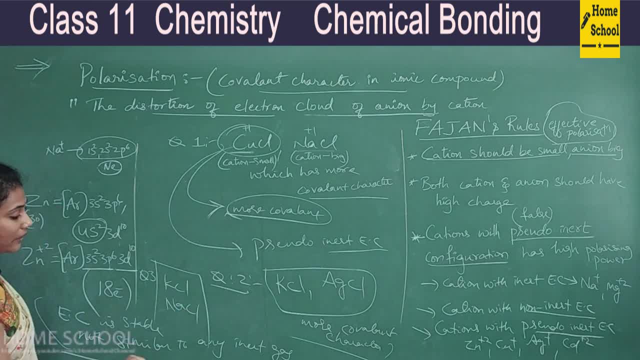 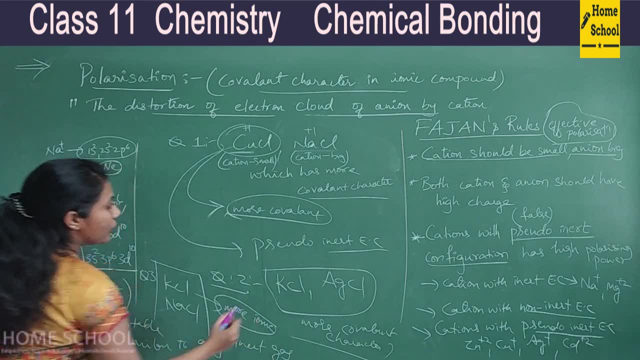 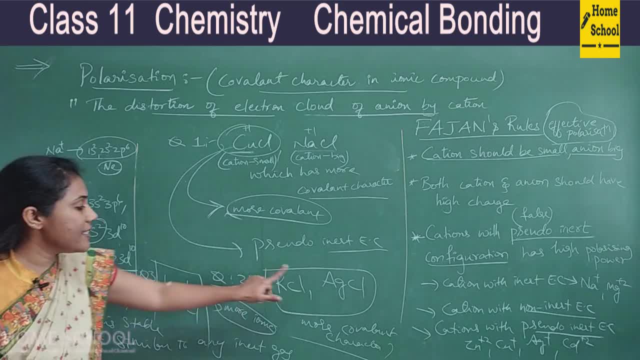 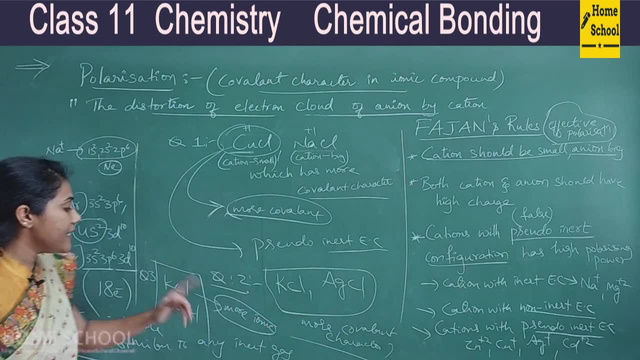 with these questions. So two questions I asked you. One is this KCL and AGCL? among them, which one is more covalent, which has more covalent character? Second question is: KCL and NACL, and tell me which is more. 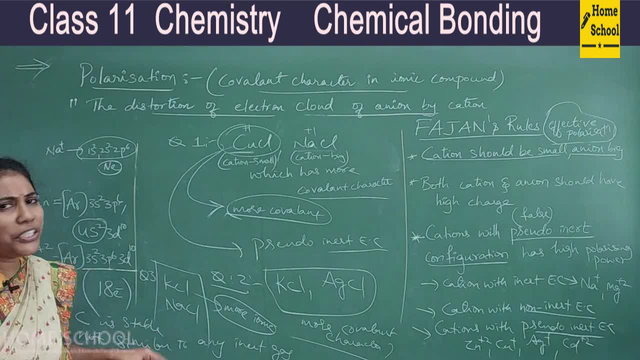 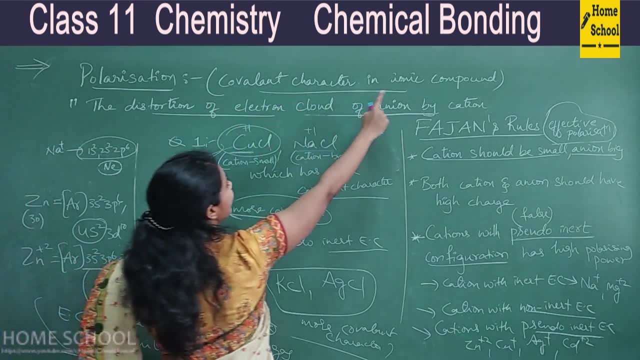 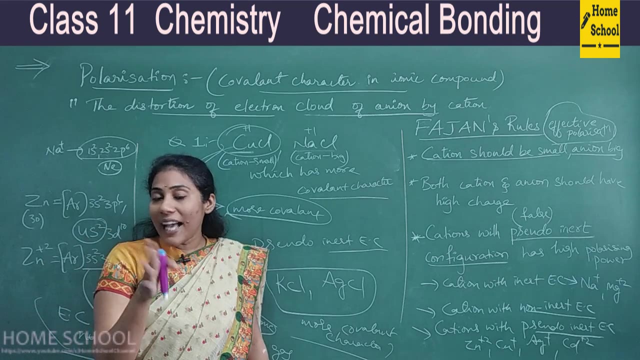 Ionic. Don't forget to post your answer in the comment section. Let me know who is answering first. Okay, So that is all about covalent character in ionic compound. I mean entire things about polarization. Okay, And now we will go for other aspect. So now every covalent. 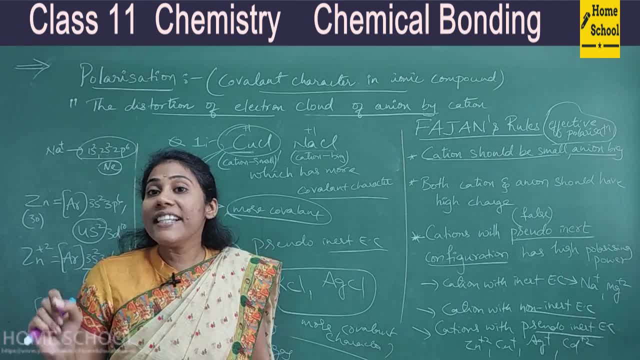 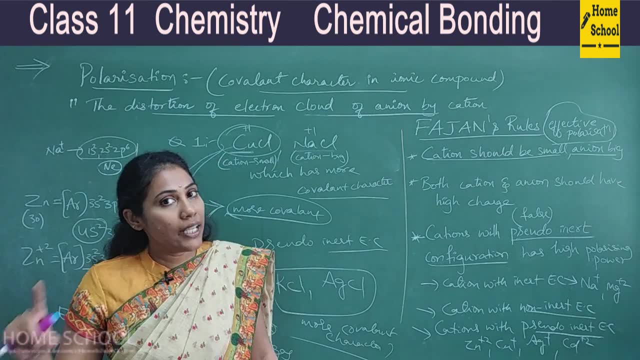 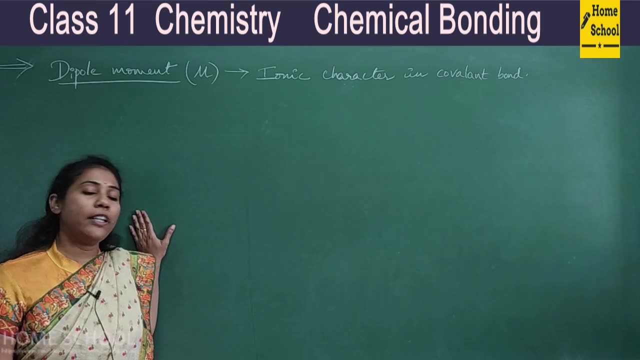 compound has ionic character, isn't it? So how do we decide that ionic character? You know that is with the help of a concept called dipole moment. So let us understand everything about dipole moment. See, guys, this dipole moment is also one of the very, very important concept that 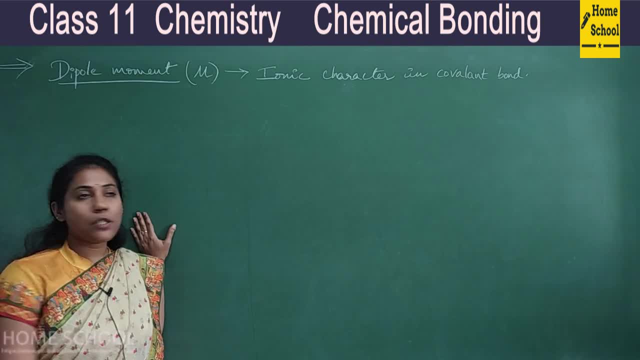 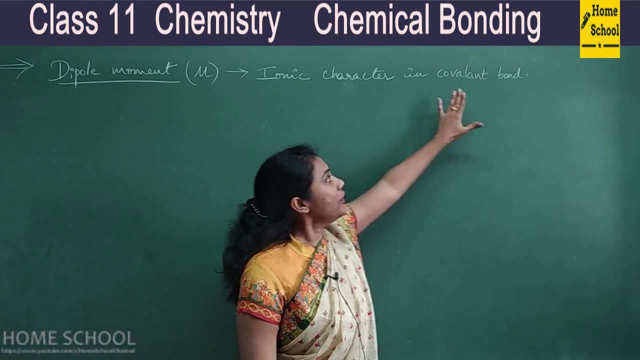 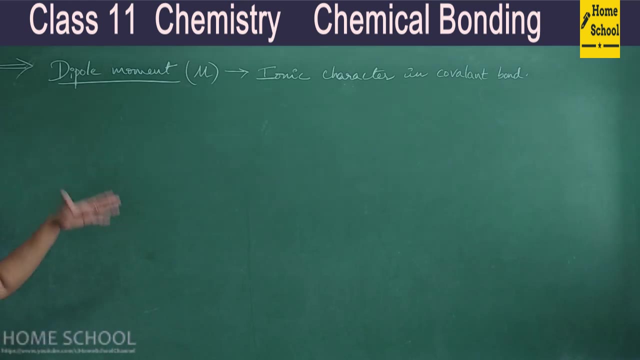 you have to concentrate. So, as I have already explained you, dipole moment will help you to decide ionic character in covalent bond. Okay So, let us understand what actually we mean by this dipole moment And how do we find this dipole moment? Okay So, let me take a covalent compound, HCl. Okay So, 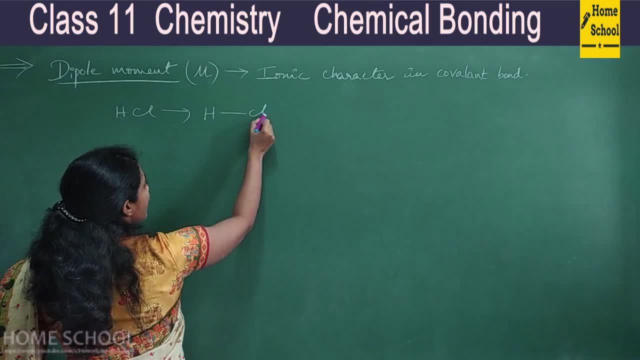 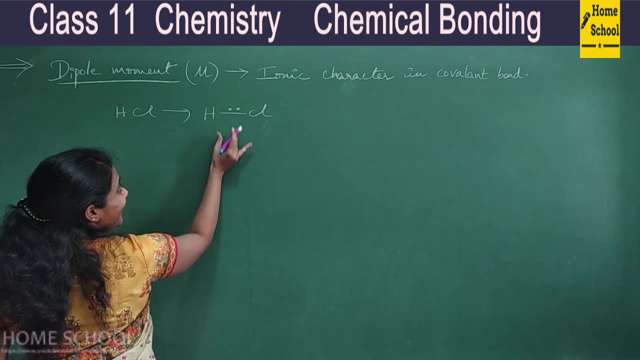 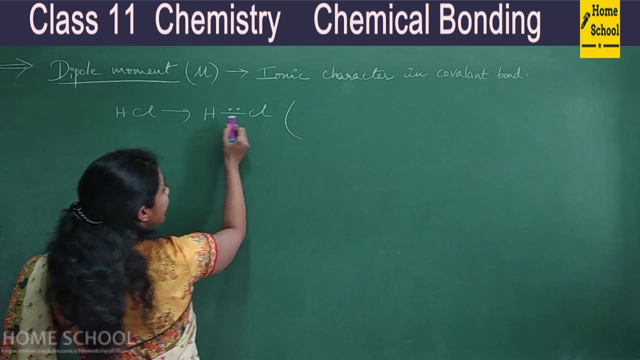 it has a covalent bond between hydrogen and chlorine. This covalent bond, which means the presence of two electrons exactly in between hydrogen and Cl. But there is electronegativity difference between hydrogen and Cl, Right? So there is. 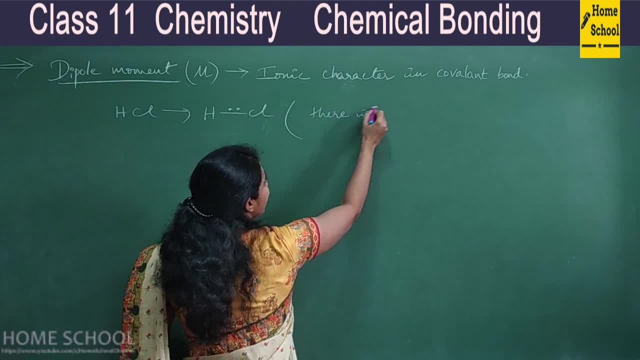 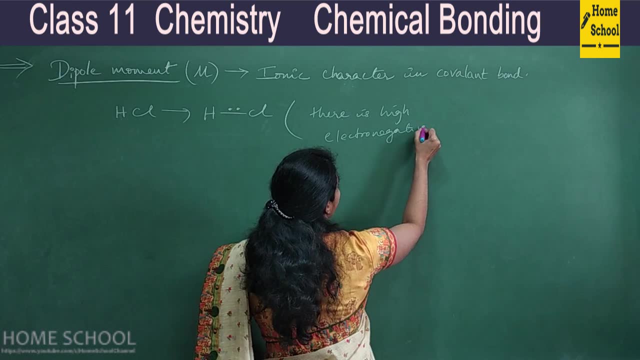 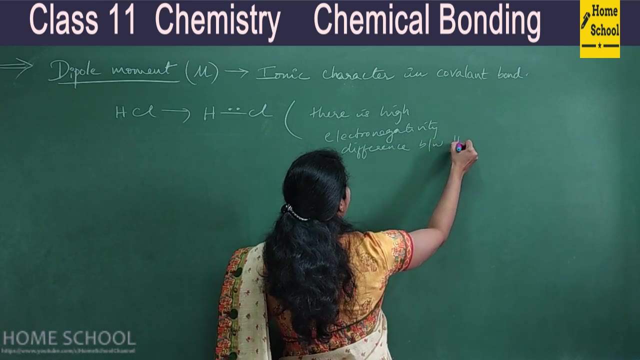 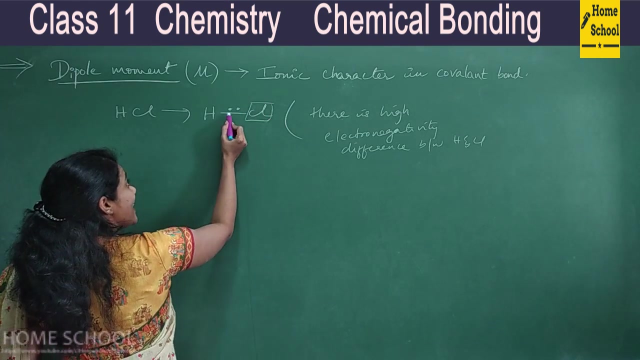 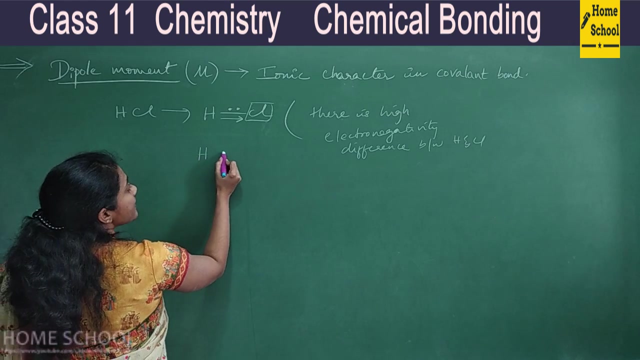 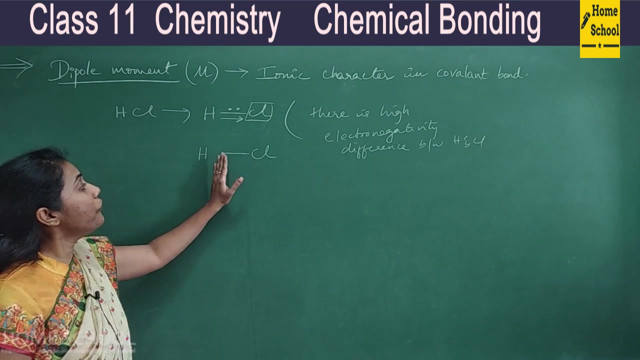 There is high electronegativity difference between hydrogen and Cl, So Cl is more electronegative here. So this has a ability of pulling this bond towards itself, Right? So what happens? So what happens? A bond is slightly moved more towards Cl. This moving of bond towards Cl creates So 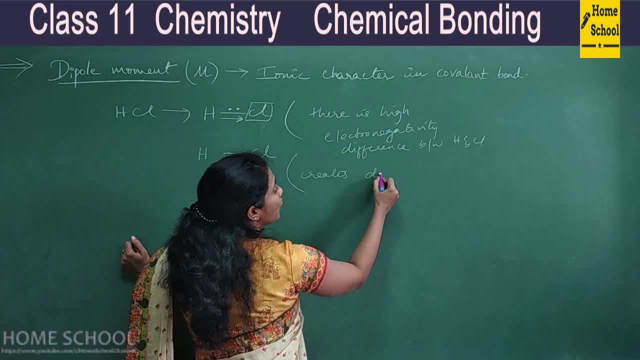 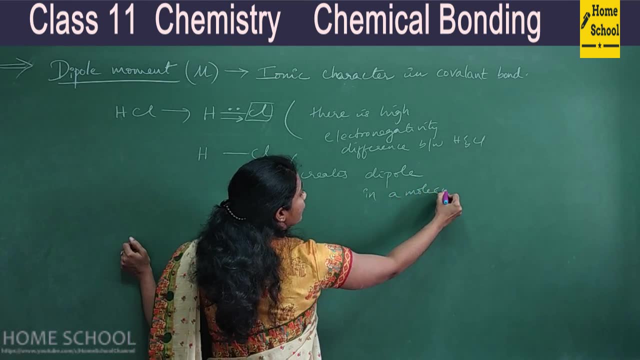 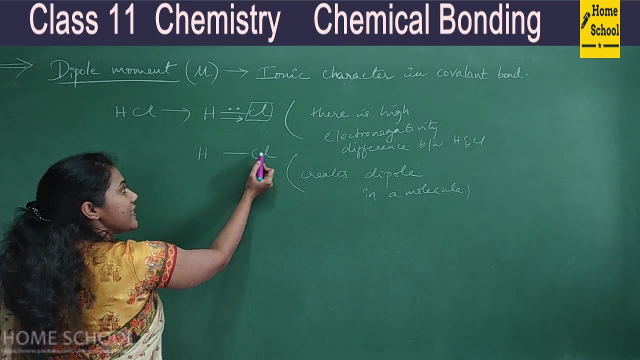 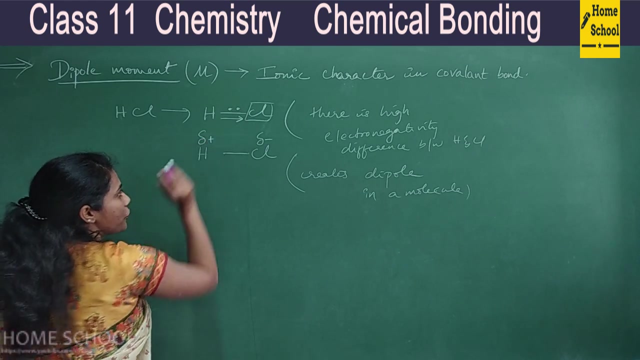 this particular concept creates dipole, Creates dipole in a molecule. Okay, So what do you mean by dipole? Dipole in the sense charge creation. See, when a bond is slightly moved more towards Cl, Cl will have a slightly negative charge, Hydrogen will gain a slightly positive charge. That means: 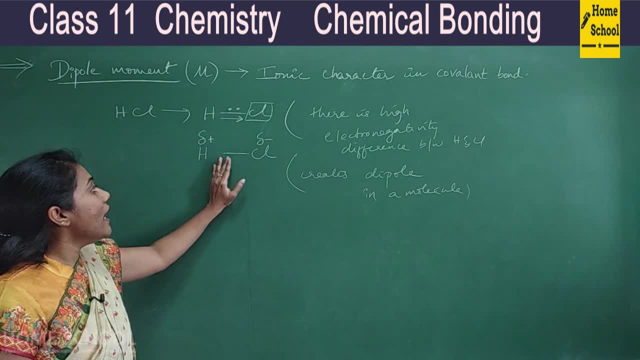 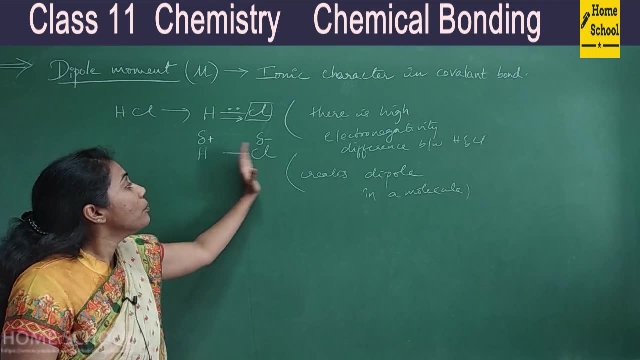 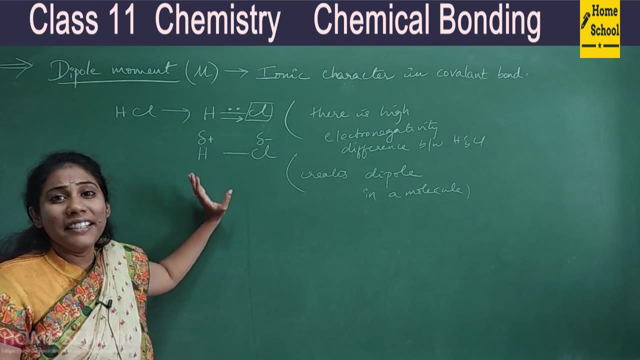 see, in a bond there was hydrogen's electrons. Now it is not completely belong to hydrogen. It is not even shared. You know that shared electron was moved more towards Cl. It is like hydrogen have lost that electron- Not completely lost, Slightly, it is losing its electron Right. 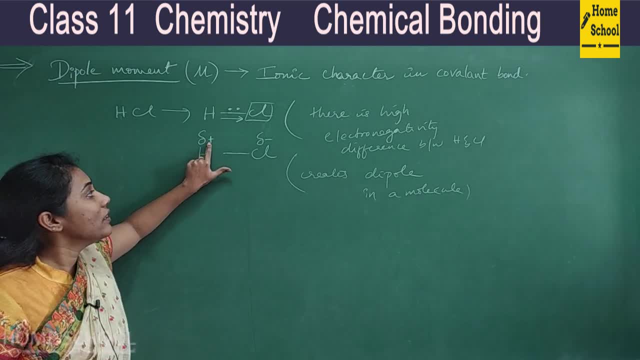 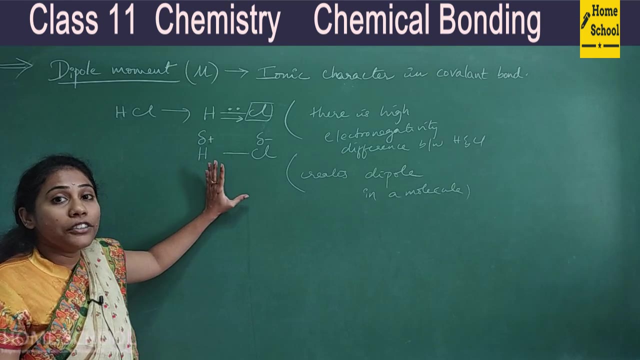 So that is why a slight positive charge on hydrogen. Okay, So this delta meaning in chemistry is slightly positive. Whenever we write delta positive, it means hydrogen is not completely positive. It has not completely lost electron. It is in a, you know, deficiency of electron. It is. 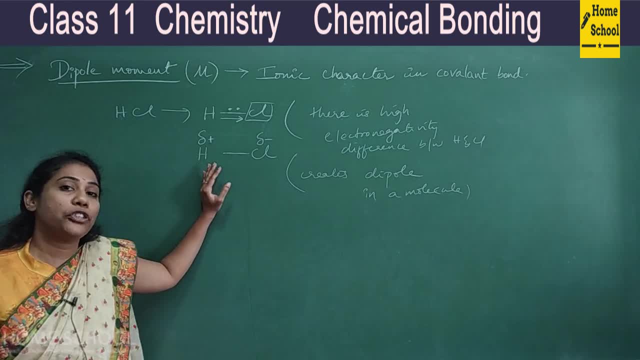 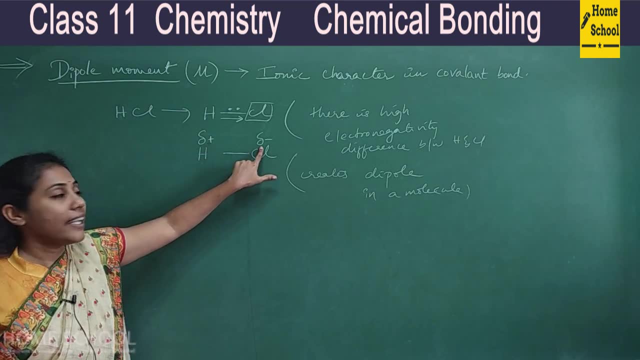 having a deficiency of electron, Slight deficiency of electron, So that is indicated with this sign: slightly positive, And this we call it a slightly negative charge. So that is why a slight positive charge on hydrogen is slightly negative. Okay, So it has not completely. took the electron of 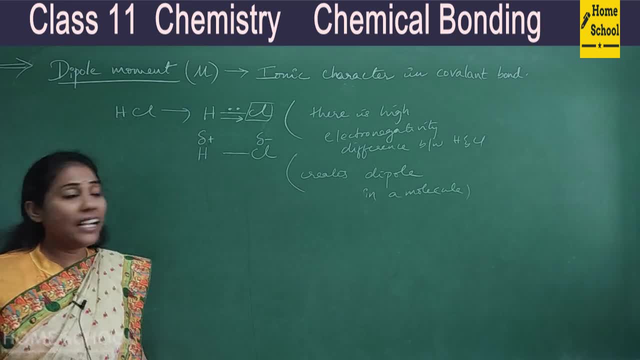 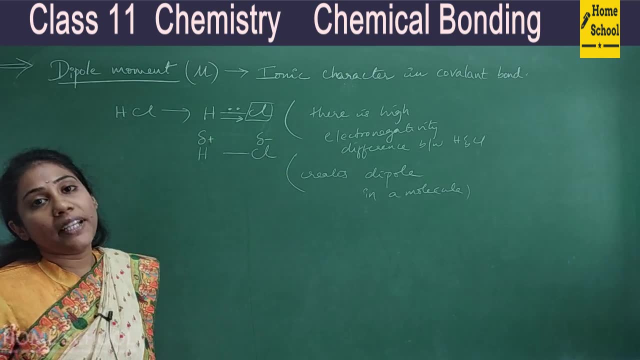 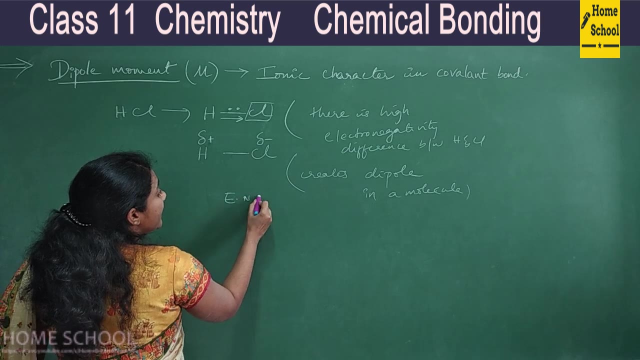 hydrogen. Just the bond is slightly moved towards Cl because this is more electronegative. So bond will always move towards the atom which is more electronegative. So why the bond has moved towards Cl? Because electronegativity of Cl is more than electronegativity of hydrogen. Okay, So that is. 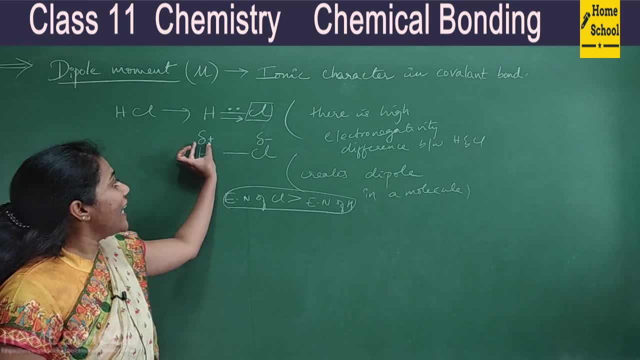 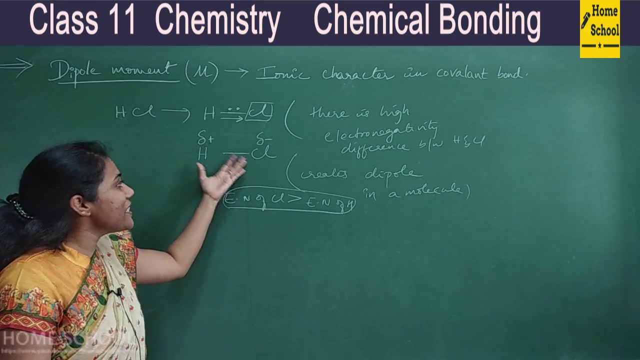 the reason bond has moved towards Cl. So that is the reason bond has moved towards Cl. So that is the reason bond has moved towards Cl. So this charge creation, slight charge creation in a molecule is called dipole. That is why we say ionic Right. So this is what ionic character. 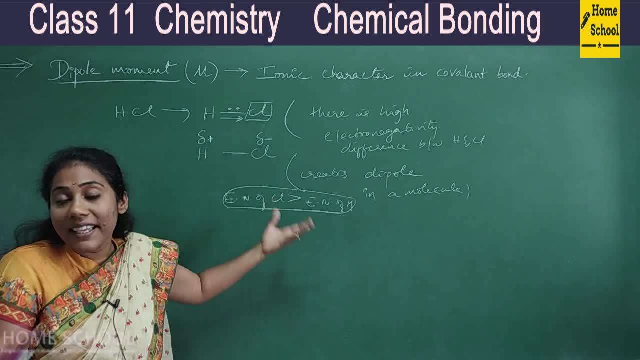 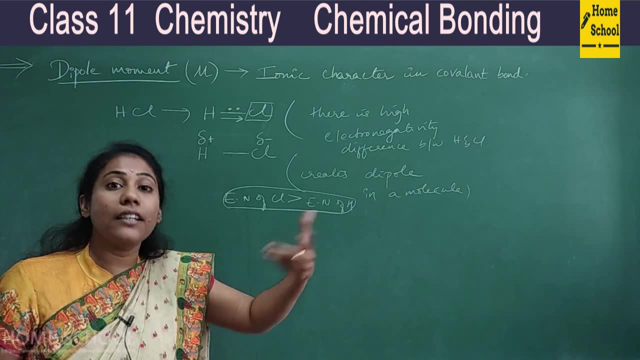 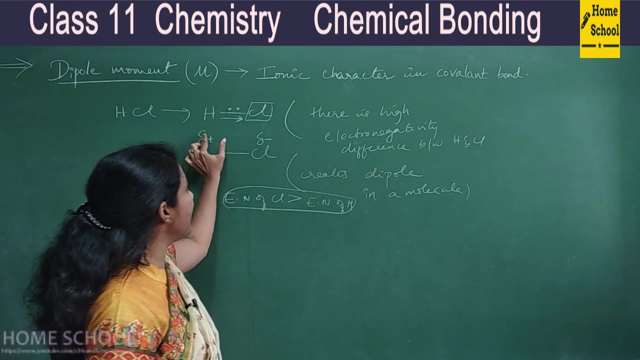 Right. So it is like a positive part is there negative part is there in a compound Right? Slightly positive, slightly negative. This is what we say ionic character generation in a covalent bond. That is what we mean by dipole. Dipole means what? Observing this slight 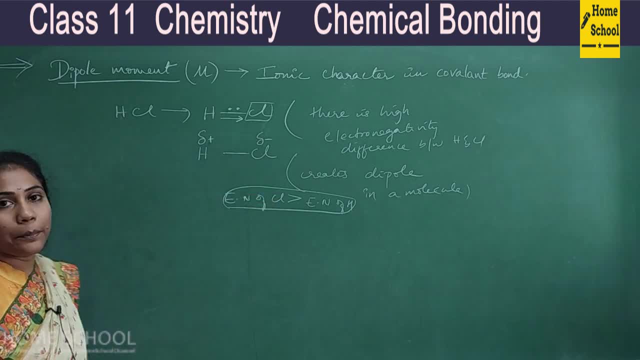 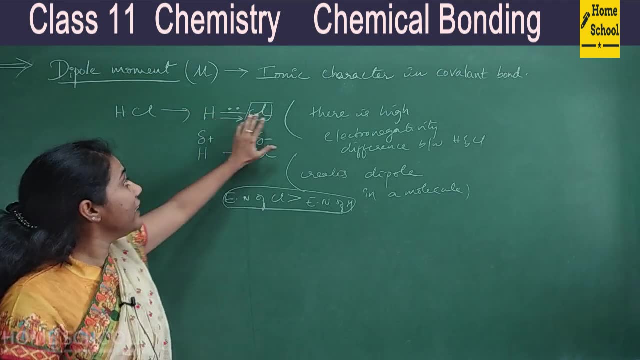 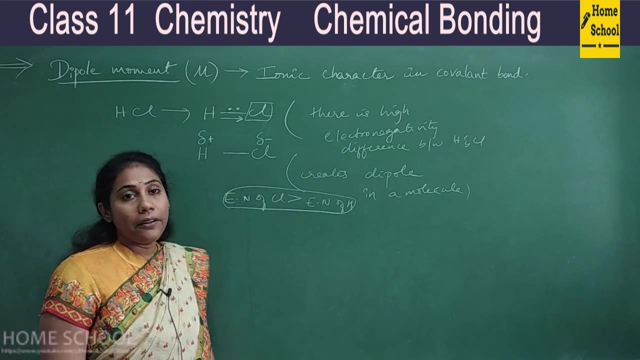 charge generation charges in a molecule is called dipole. Okay, So you will observe dipole only when there is a high electronegativity difference between the two atoms. Okay, So this is how ionic character is observed, even in a covalent bond. And now the strength of dipole. 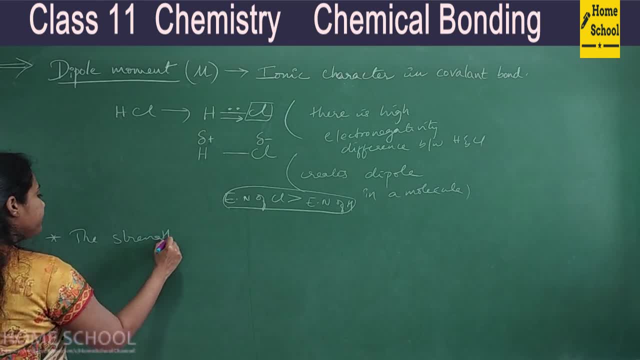 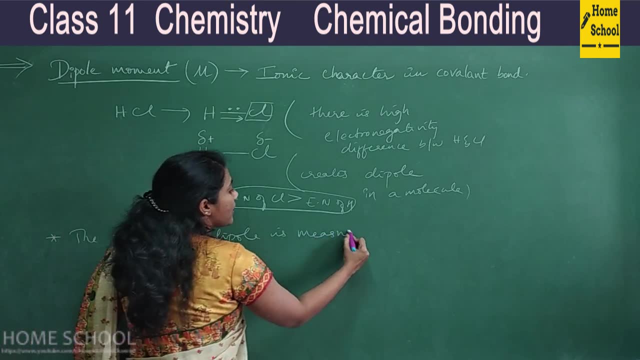 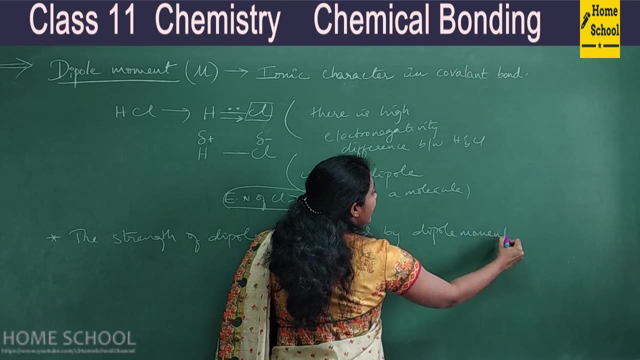 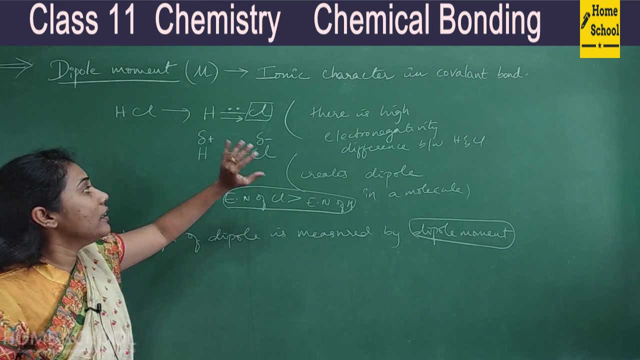 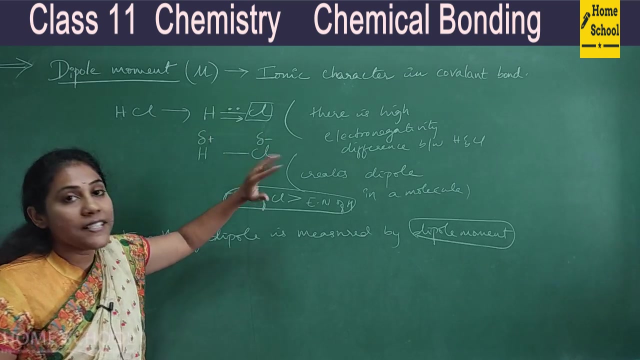 the strength of dipole is measured Is measured by a concept called dipole moment. Okay, So what is dipole moment? Dipole moment is used to measure the strength, how much extent the charges have been developed in a molecule. You know, if the charge on two atoms is more, then we say more ionic character is there in a. 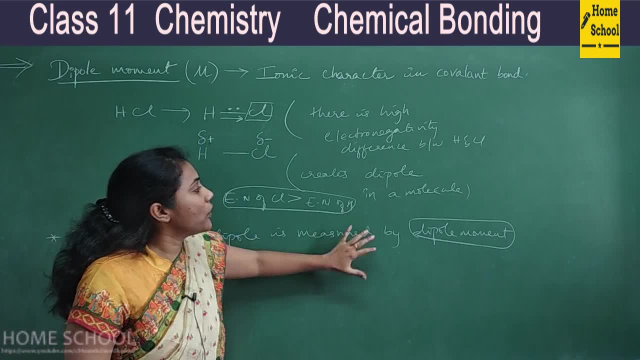 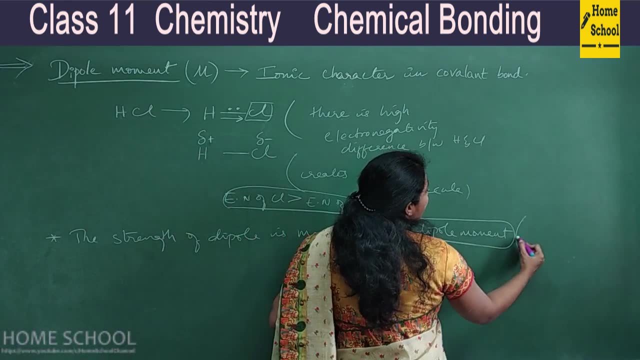 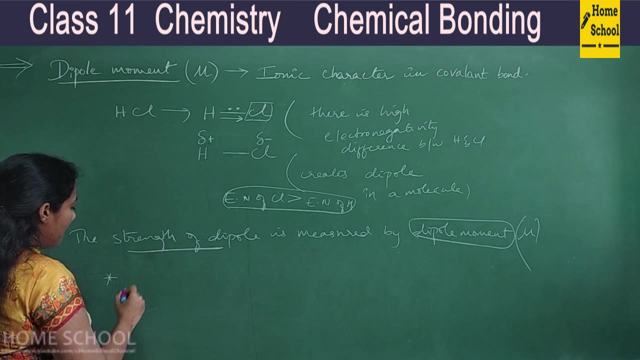 covalent bond Right. So the strength of this charge formation is measured by a concept called dipole. In other words, strength of dipole is measured by dipole moment, which has a symbol nu. Okay, So if I have to give the definition of dipole moment, it is nothing, but you know the product. 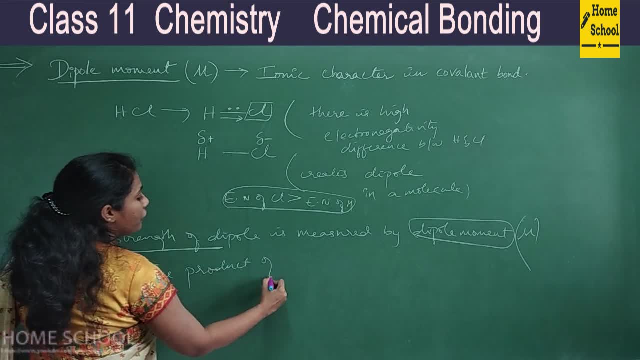 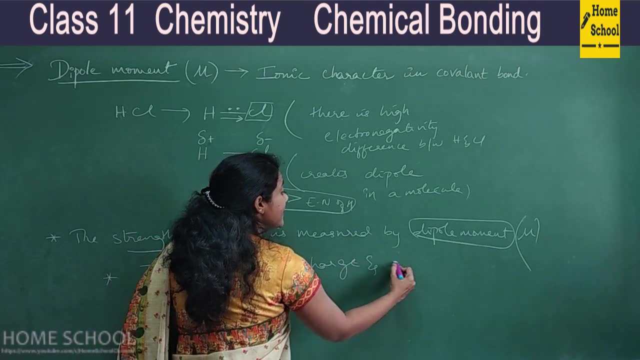 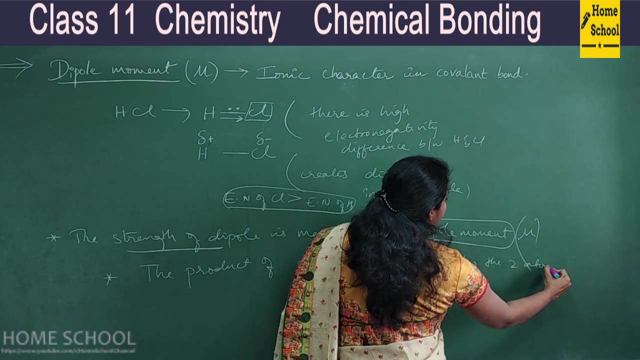 of it is the product of charge, charge and distance. Distance between two atoms. distance between two atoms: Right, Like the difference in the distance between the two atoms, the between the two atoms. okay, so that means say this is what the formula we write, mu is equal to. 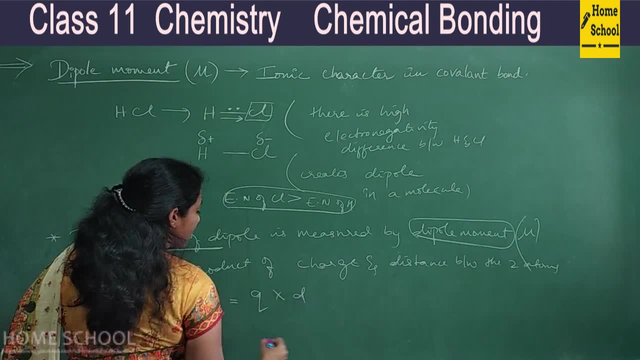 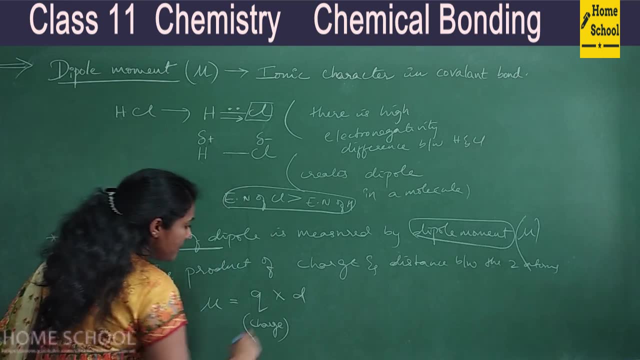 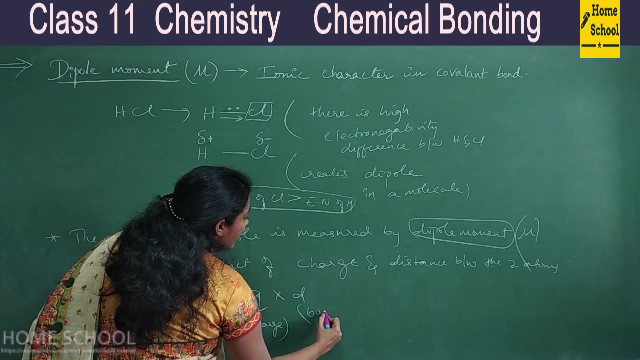 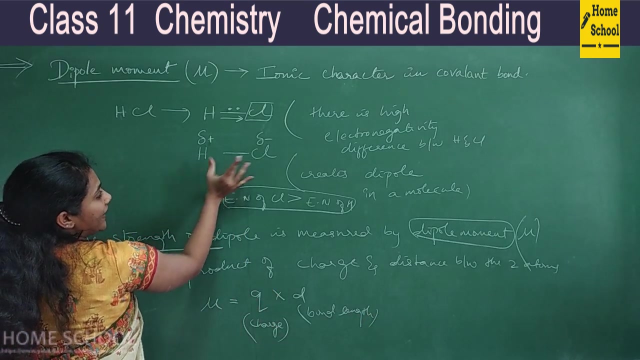 charge q into d. so what is q here? q is nothing but charge of ion, I mean charge of atoms, and d is distance between the atoms. so distance between the atoms is nothing but what bond length? right, that's what we can also call it as bond length. bond length is the distance between the two atoms. 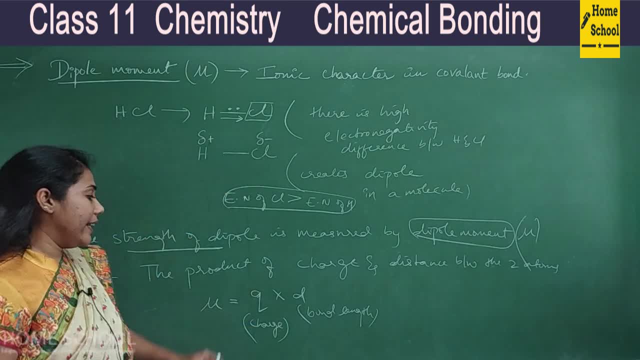 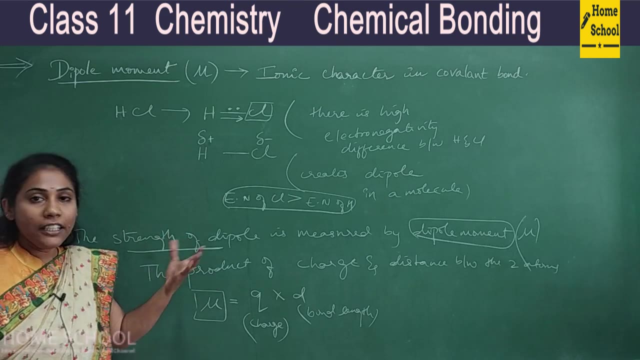 you know this distance. we will call it as bond length. so charge into bond length or distance. if you do, you will get the value for mu. that is dipole moment. looking at the value, you can say whether a compound has more ionic character or less ionic character. more the dipole moment. 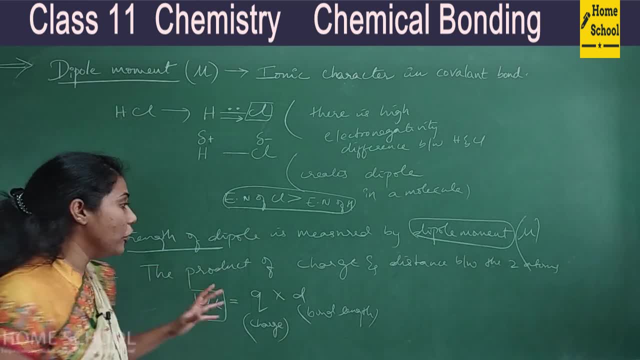 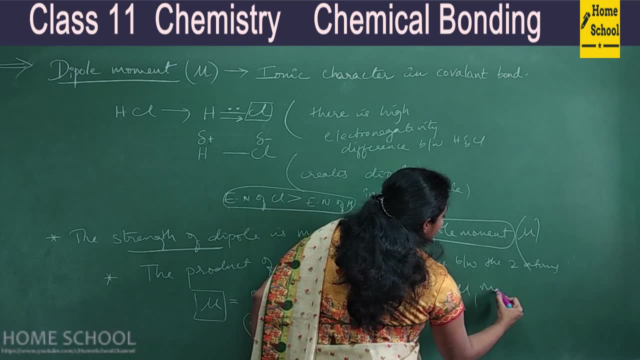 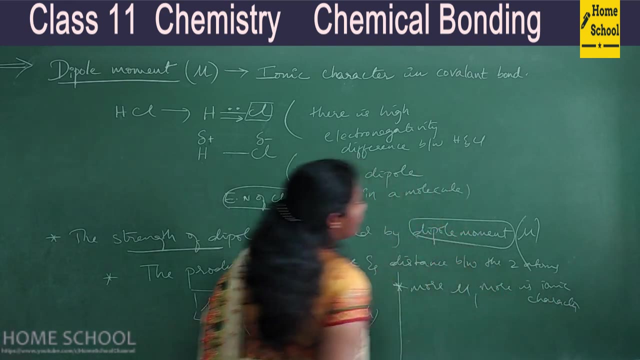 more ionic character is there in a motion along that graph. okay, so that is the value of typing in position in that graph. so, covalent compound, okay. so how do you decide more? if you have more nu, then more is ionic, ionic character, right? so this is what you need to understand, and few more things. let's, let's come. 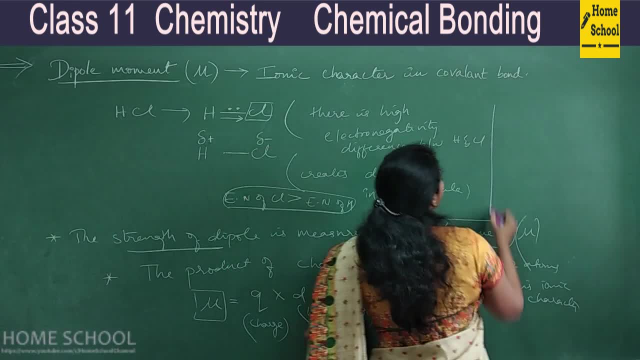 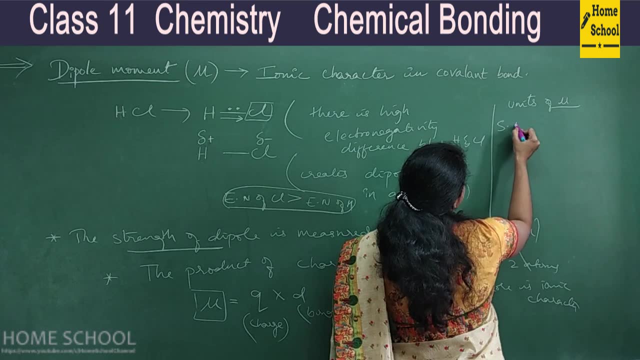 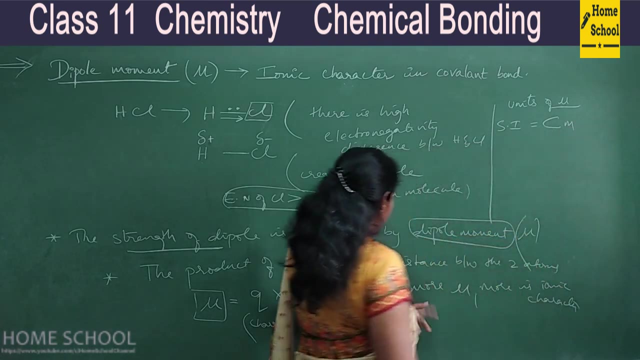 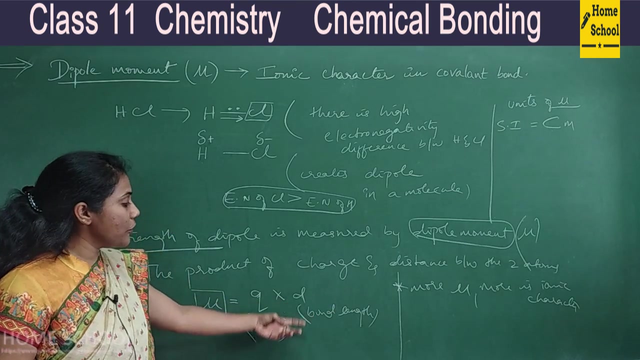 to the unit of nu here. so you should have an awareness about units of dipole. moment, that is nu. in si system, that is in mks system. the unit is coulomb meter. okay, c for coulomb charge. you know, charge unit is coulomb and distance it's like bond length is nothing but distance unit is meter. 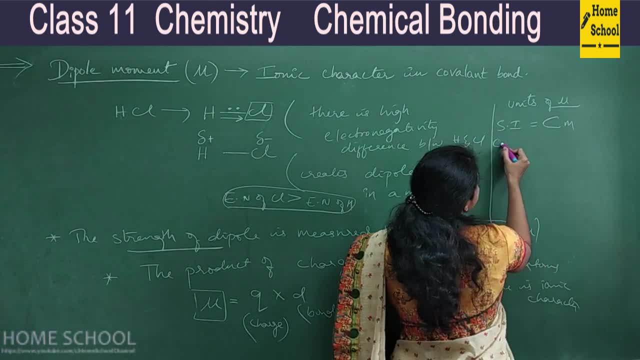 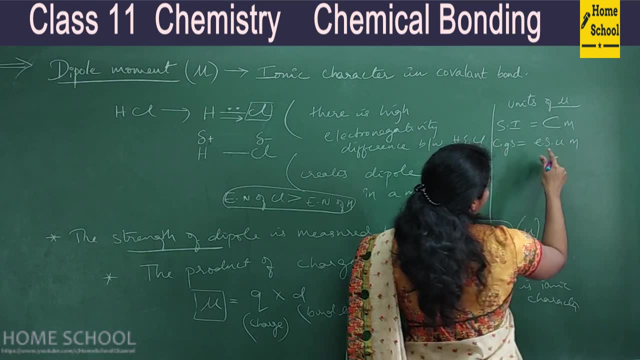 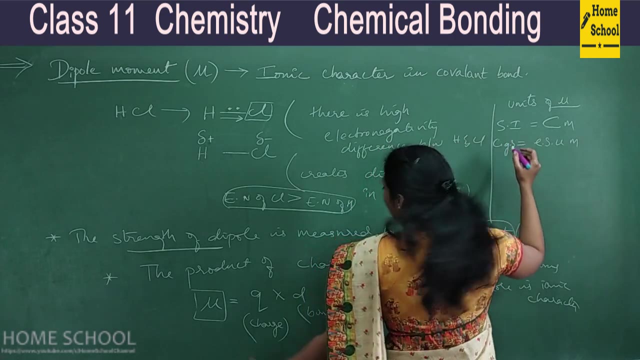 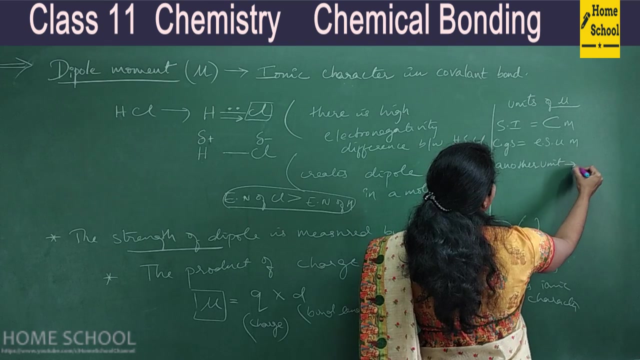 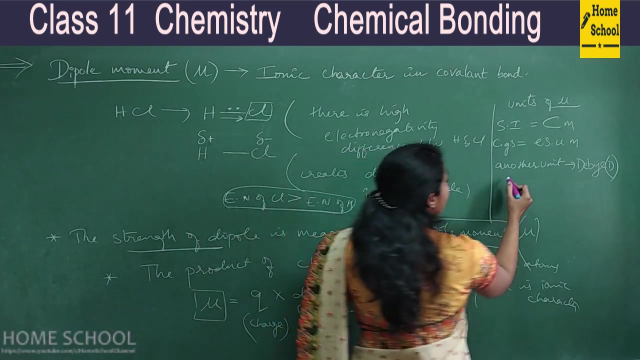 right, so coulomb meter is the unit in cgs system. the unit is esu into meter, esu. electrostatic force is called as esu, esu into meters. okay, so, uh, and dipole moment has another unit, another unit okay, which we famously call it as debi. debi, which is represented as d, okay, so here you need to understand one debi. 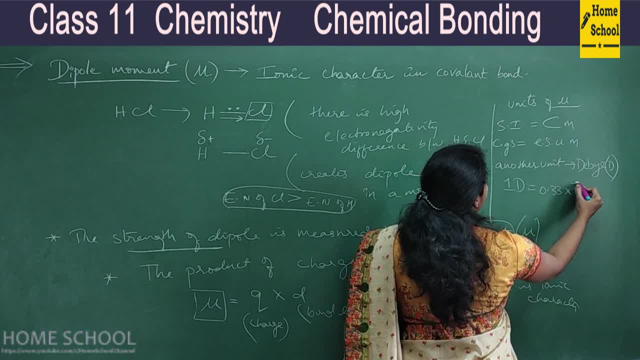 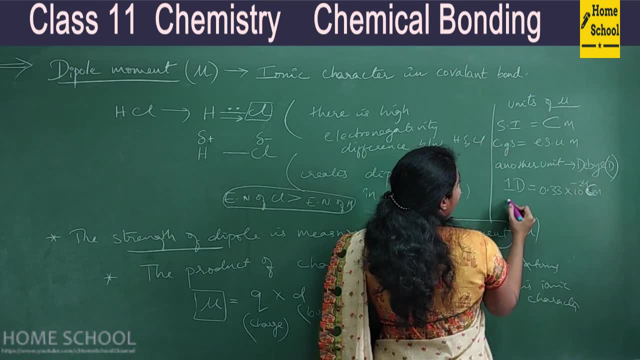 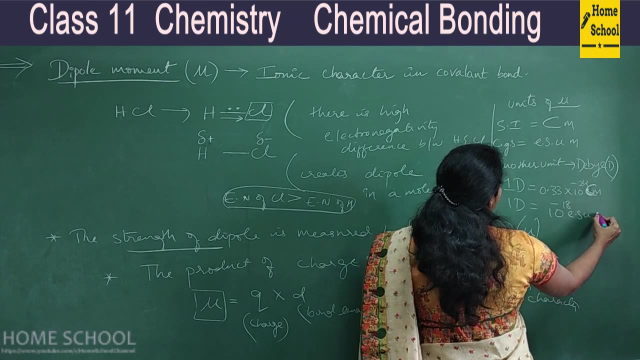 is equal to 0.33 into 10 power minus 24 coulomb meter. coulomb meter, it's not centimeter, it is centimeter, okay. or one debi is equal to 10 power minus 18 esu into centimeter, okay, so one debi's. 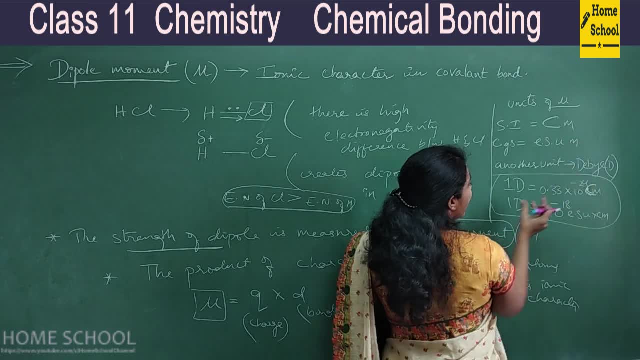 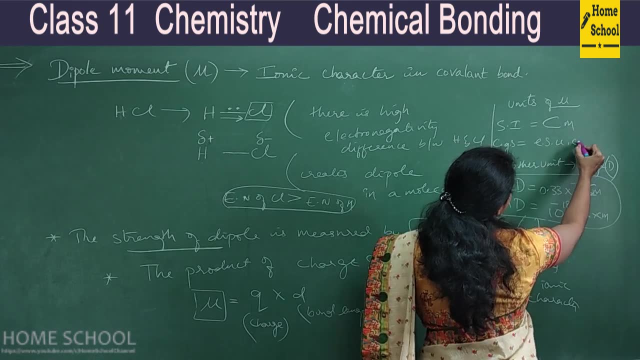 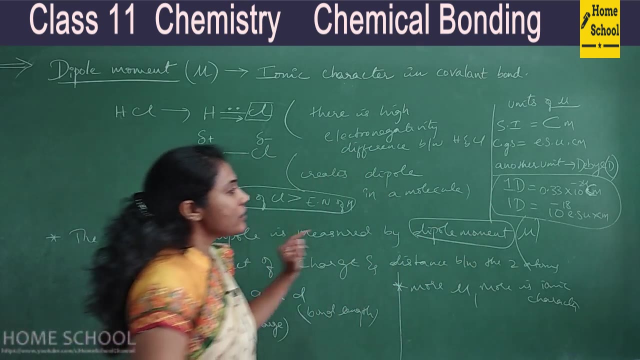 value is this much in coulomb meter units, and one debi is this much in esu centimeter unit. sorry, here it should come centimeter right in cgs system. so these are the units of. you know that Kirane u1 and u2 in centimwrart. so we have k3 in dzd. so one debi is 1 centi troubled meter. 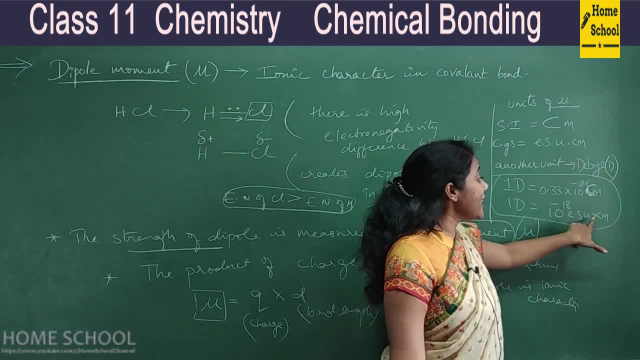 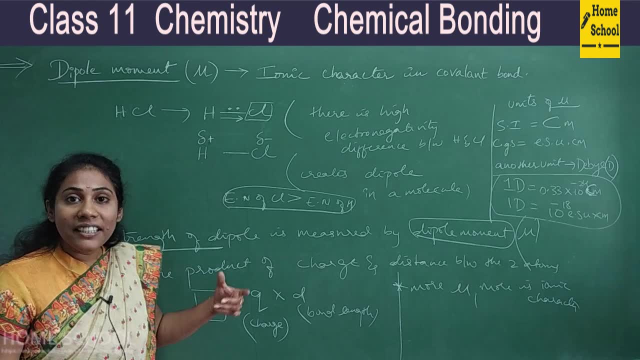 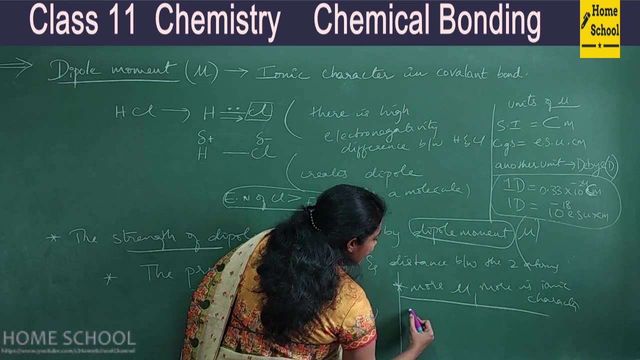 okay, then this is how youboy makes the difficult Blake, because k1 is değrary in it, then b goes in to lady and dibi is to cold moment. okay, so the most important unit is deep ae. div buy is just a unit, okay. so one dibi is this much coulomb meter and one debi is this much ESU centimeter. so this: 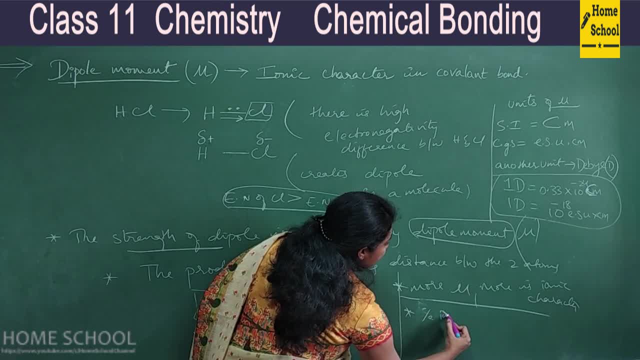 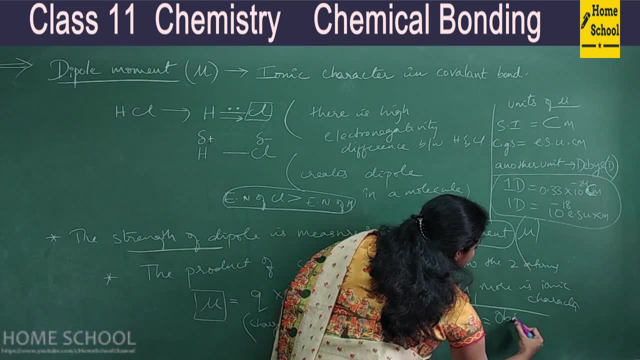 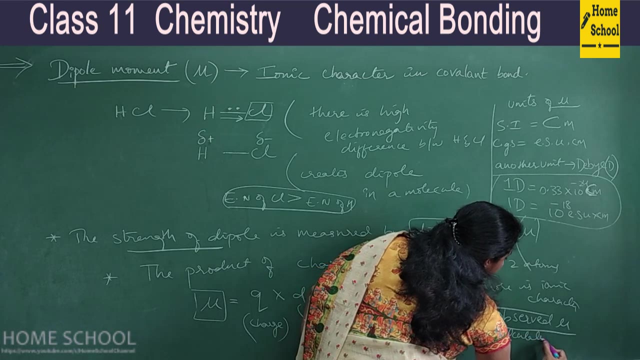 is what you need to understand. and now you know we can actually calculate the percentage ionic, ionic character in any covalent compound. the formula is observed: observed dipole moment divided by calculated dipole moment into 100. okay, so this formula is very, very important, guys. 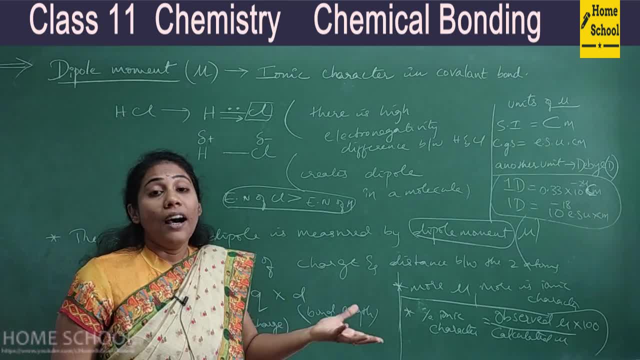 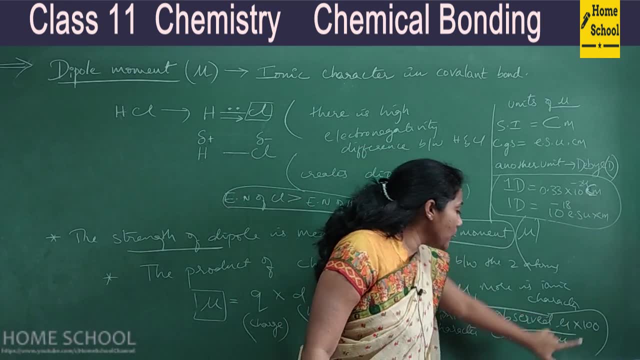 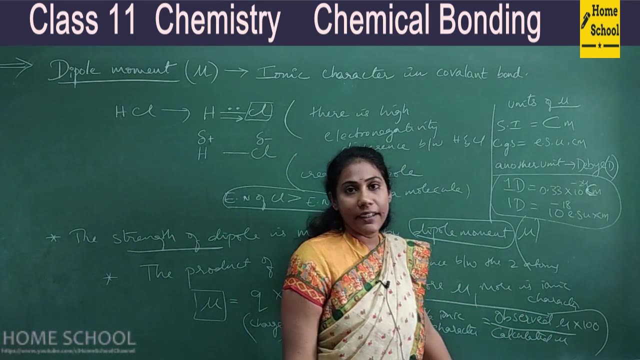 so percentage to how much percent ionic character is there in a particular compound? that if you want to calculate the formula is this: observed dipole moment divided by observed dipole moment, divided by calculated dipole moment into 100. so now we will see one problem where we can apply this formula. 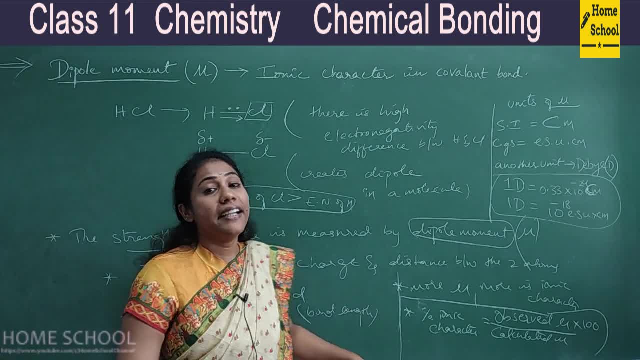 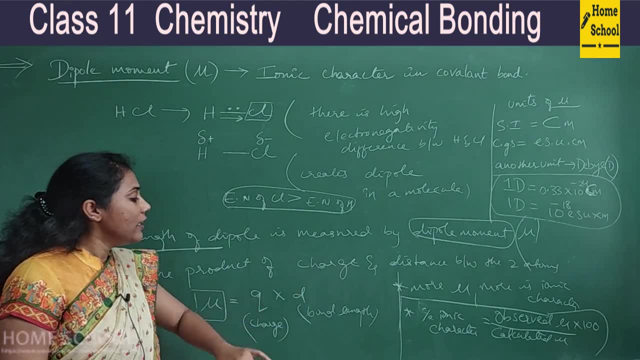 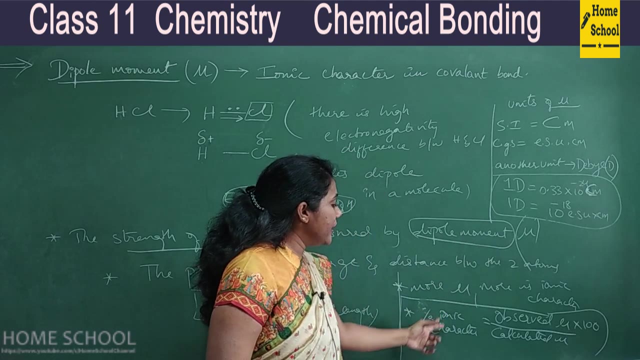 so that you will get an idea how actually we calculate dipole moment. so what is the major formula of dipole moment? it is the charge into bond length, that is, the distance between the two atoms. okay, so these are the values and this is how we can calculate percentage ionic character. let's see one problem here. 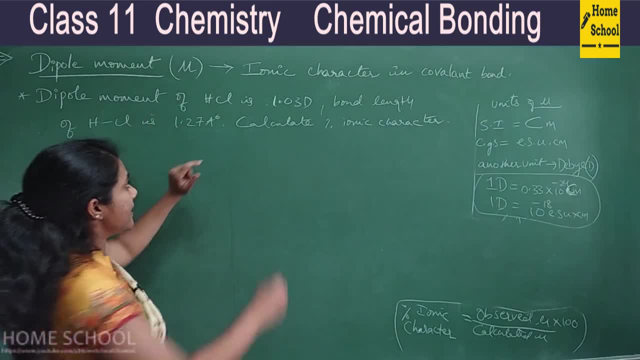 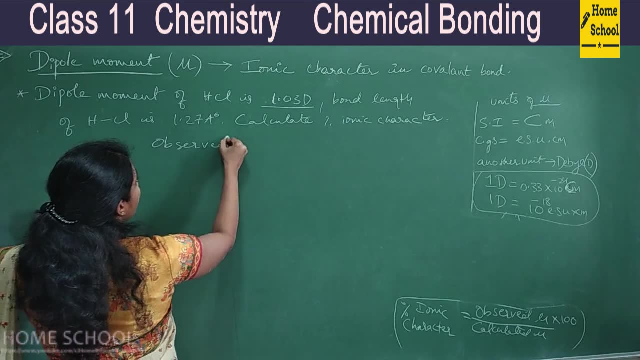 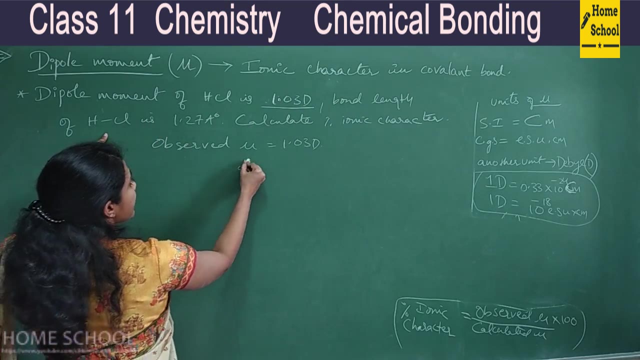 see this problem guys. dipole moment of hcl is 1.03 d. that means it's a observed observed dipole moment. they have given 1.03 d. bond length of hcl: they have given that is d. they have given 1.27 angstrom calculate: 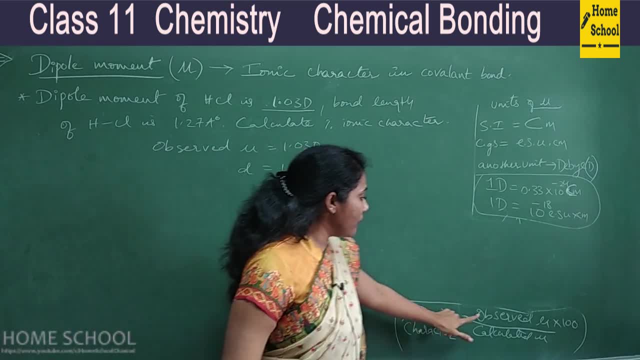 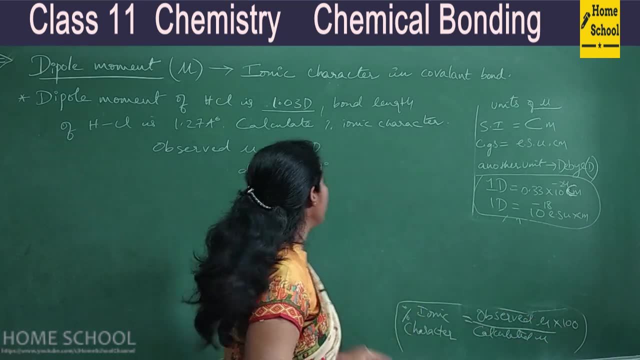 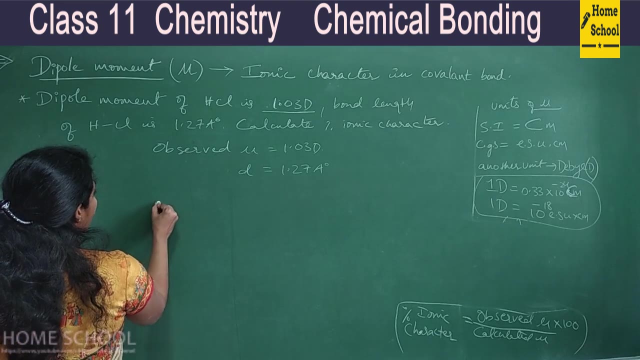 percentage ionic character. what is the formula here? we have observed you observed dipole moment divided by calculated dipole moment into 100 observed dipole moment. they gave. we have to calculate calculated dipole moment, right. so how do you calculate dipole moment it is charge into? 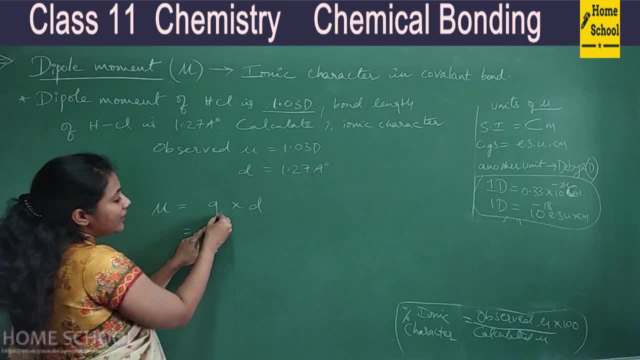 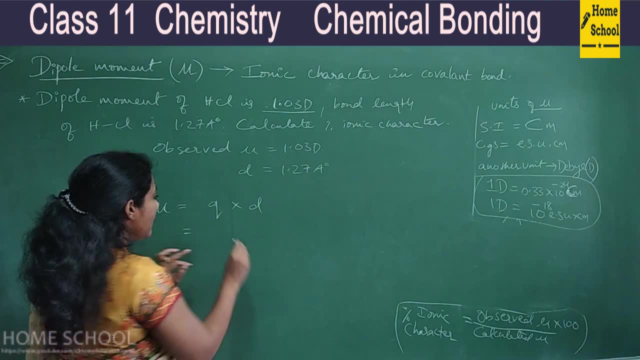 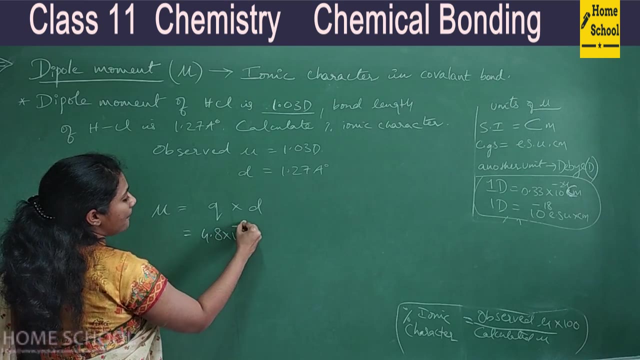 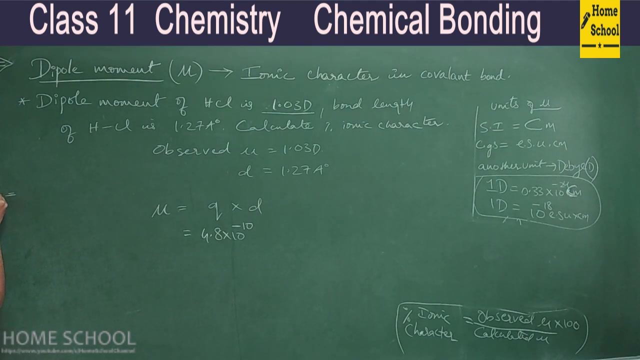 distance, isn't it? so what is the charge here in esu centimeter? let us calculate new in esu centimeter units. I am calculating. So charge value in ESU centimeter is how much 4.8 into 10 power minus 10.. Okay, So charge, we know. charge of an electron is how much 1 unit charge. 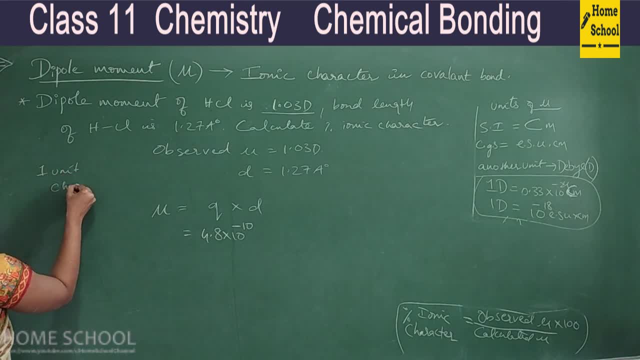 1 unit charge value is how much? 1.6 into 10 power minus 19 coulomb. It is in coulomb, But in electrostatic units its value is 4.8 into 10 power minus 10 ESU. we say Okay So. 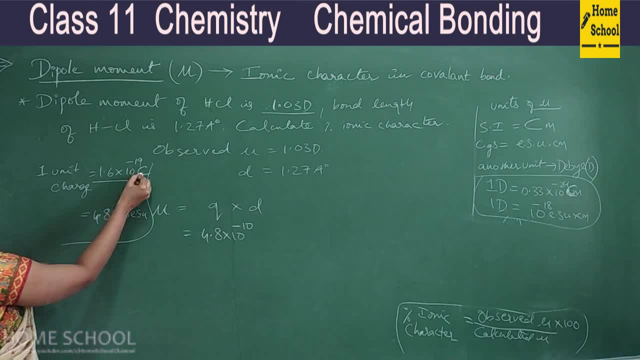 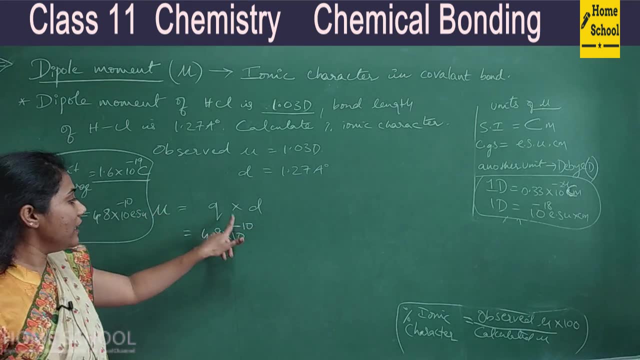 in ESU charge value is this much. In coulombs charge value is this much. So I am calculating. you know the new value in ESU centimeter. So I took charge value in this units 4.8 into 10 power. 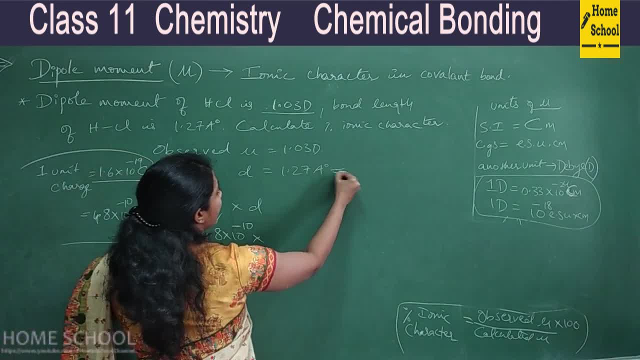 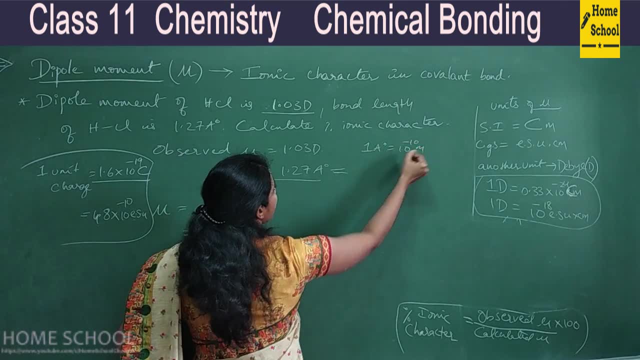 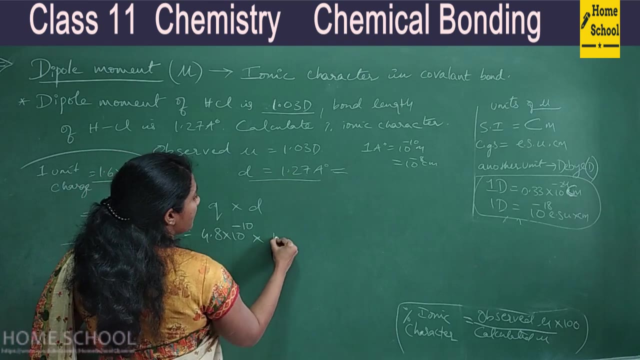 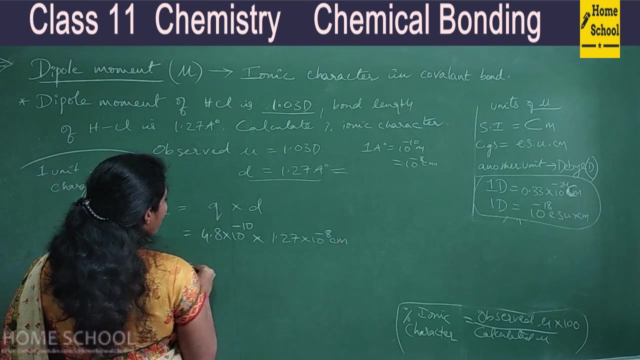 minus 10 into distance, Distance. I need to take it in centimeter. So we all know: 1 angstrom is equal to 10 power minus 10 meter, which is equal to 10 power minus 8 centimeter, Right? So how much? 1.27 into 10 power minus 8 centimeter. So what is the new? 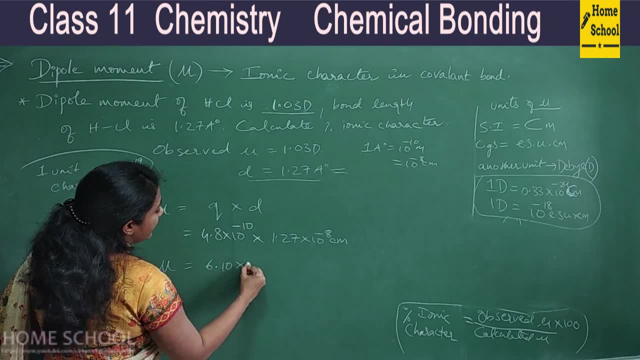 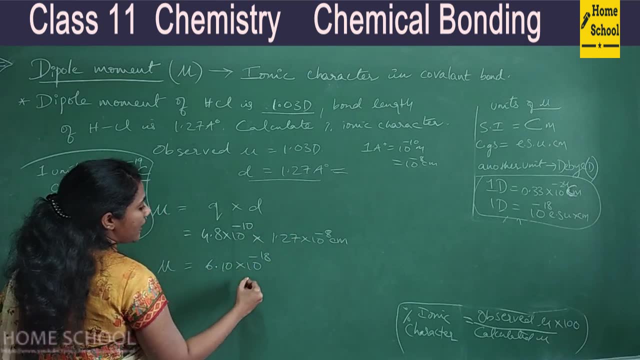 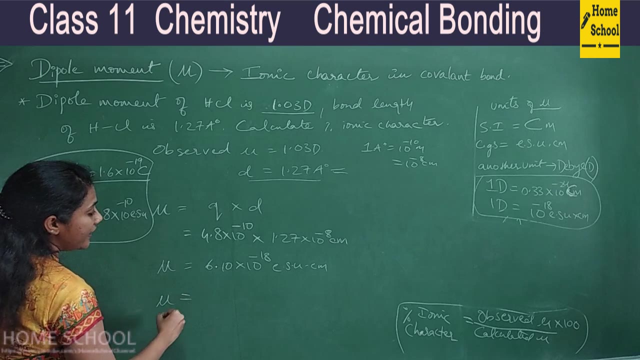 value you will get here: 6.10 into 10 power right minus 8, 10 power minus 10 into 10 power minus 8 minus 18 ESU centimeter And convert this in Dubai unit, It is 6.10 into 10 power minus 18. 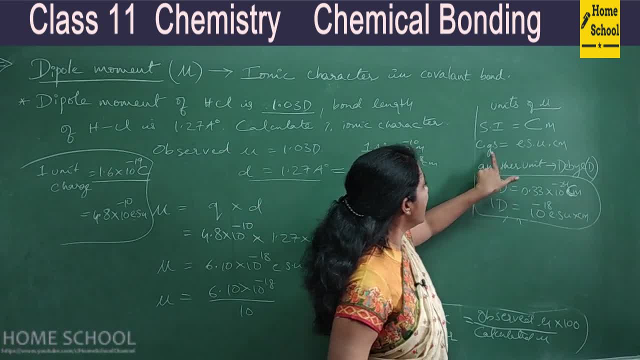 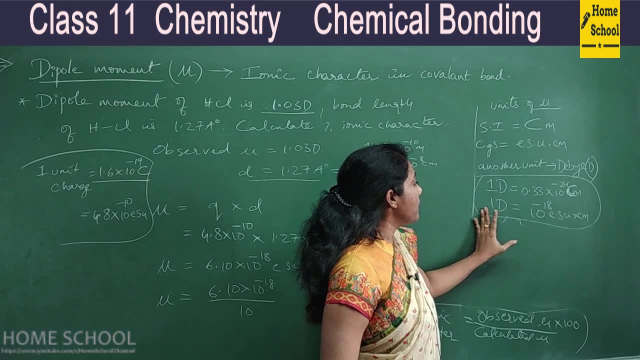 divided by 10 power. See, if you want to convert 1 Dubai in you know CGS- from CGS units to 1 Dubai, it is 1 Dubai is equal to 10 power minus 18 ESU centimeter Right. So I will divide by 10 power. 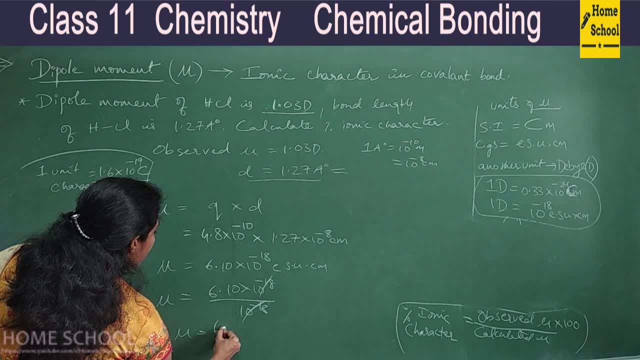 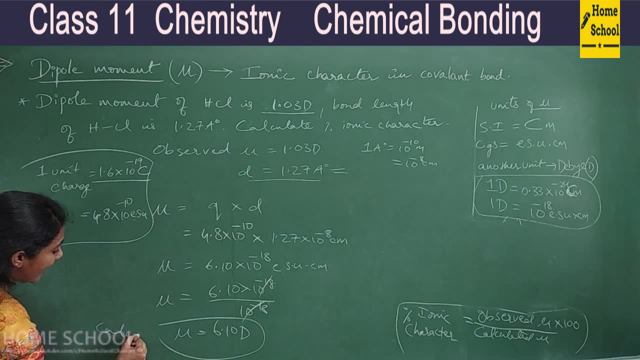 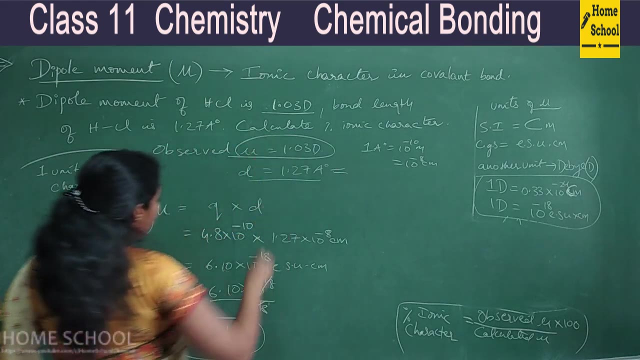 minus 18.. This gets, So new value is 6.10, Dubai. Okay, What is this dipole moment? This is actually our calculated dipole moment. So now you have observed dipole moment that is given in a question. This is our. 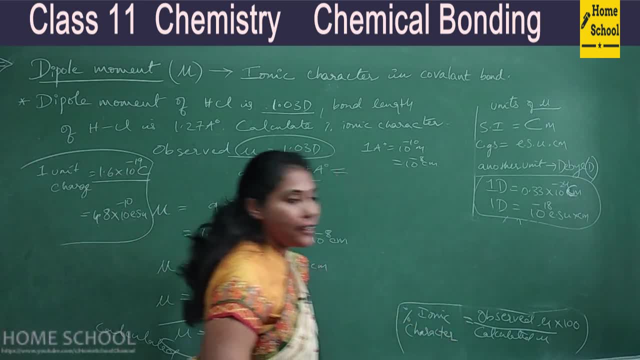 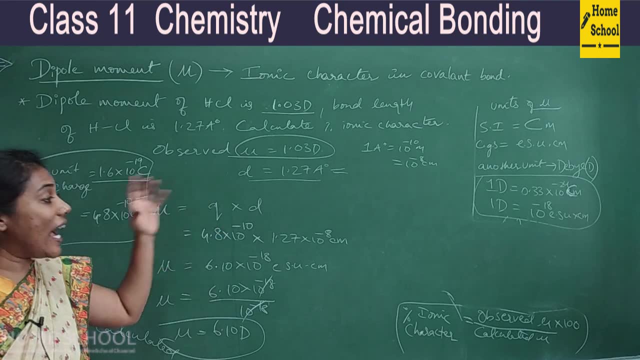 calculated dipole moment. So use the formula and find out. So post your answer in comment section. Okay, So calculate. post the percentage ionic character that is there in HCL bond, Right? So this is how we can calculate dipole moment. See, guys, using dipole moment, we can. 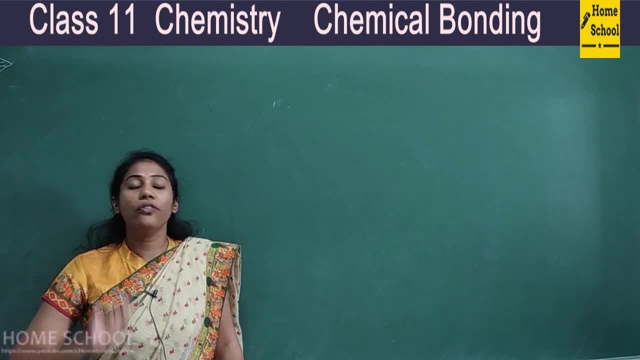 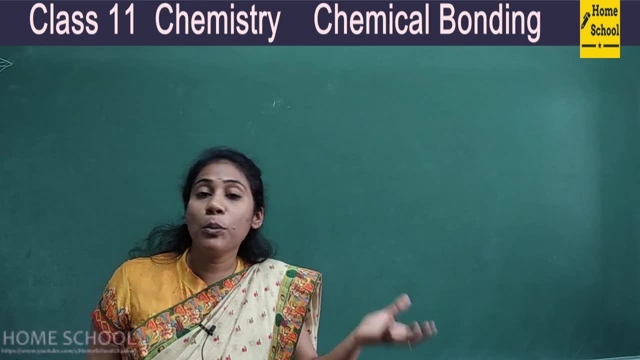 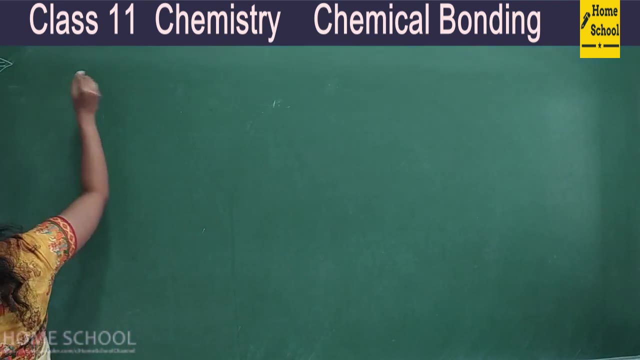 decide the shape of these covalent molecules, or from knowing the structure of covalent molecule, we can say whether dipole moment is there or not. Okay, So that is what we will try to learn now You know, identifying dipole moment from structure. 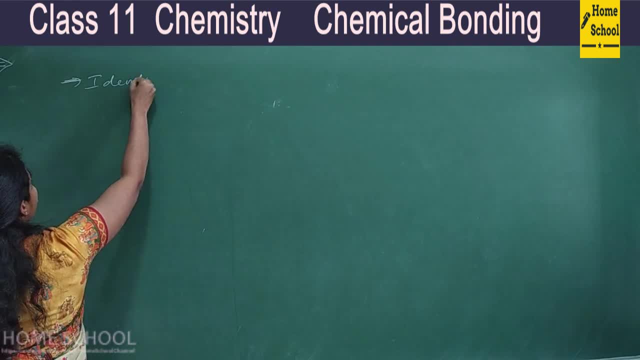 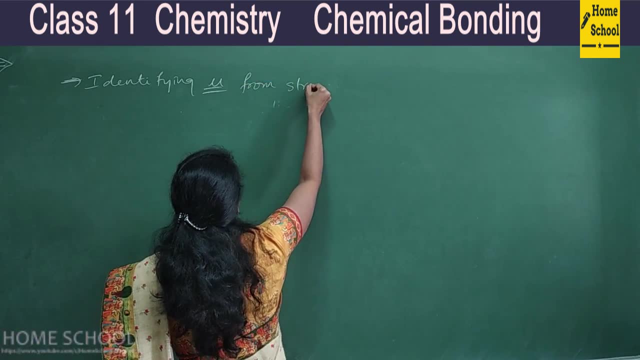 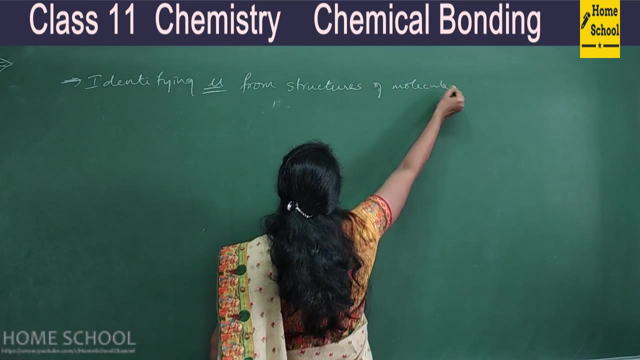 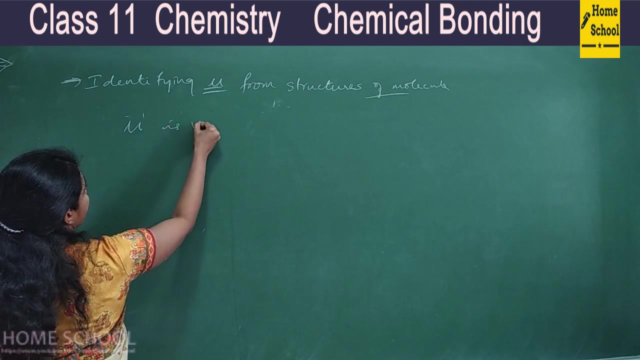 So what I am dealing is identifying dipole moment from structure of molecules, Structures of molecules. So this is also very, very important thing one must understand. First thing you need to learn is your dipole moment is vector quantity. So we know the properties of vectors Right. So vector quantity. 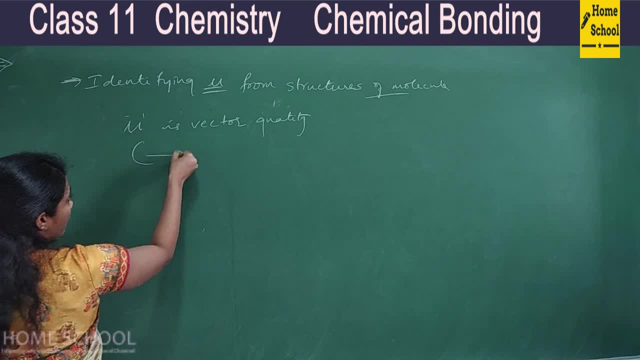 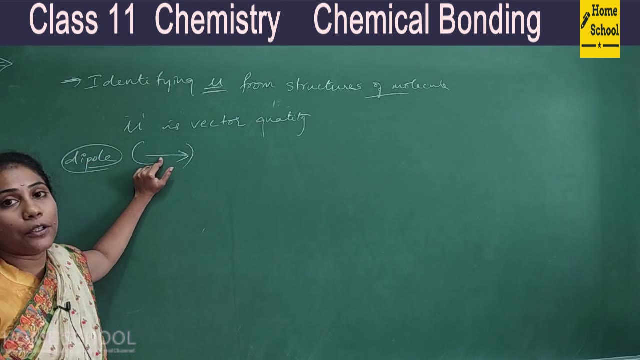 is vector quantity. It will be mentioned with the help of arrow mark. Dipole moment is mentioned with the help. of you know dipole, Especially not the dipole moment. Dipole in a molecule can be represented with the help of arrow mark. Okay, 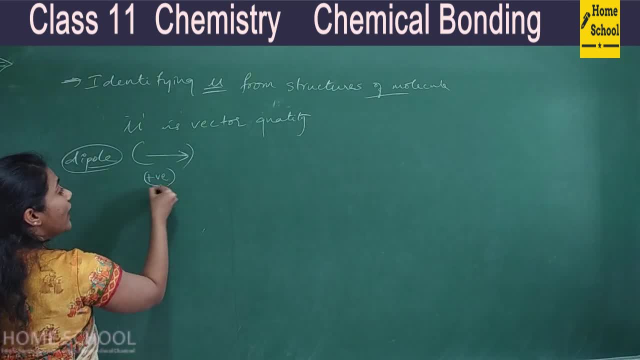 So you have to show arrow mark from positive atom to negative atom. Okay, For example, you see, carbon dioxide. Carbon dioxide has a linear structure. How do you know that carbon dioxide has a linear structure? You will understand this in VSEPR theory that you will study next. Okay, So just as of now, 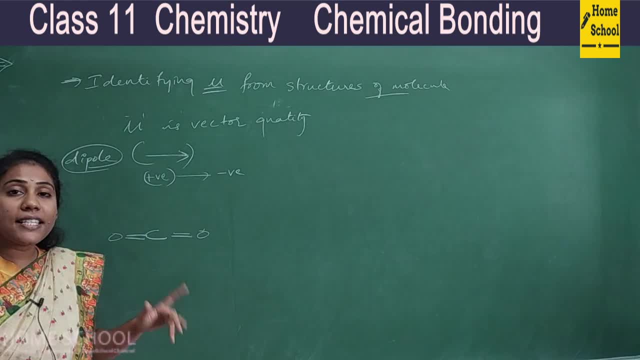 this is the structure of your carbon dioxide And I want to decide whether carbon dioxide shows dipole moment or not. Okay, So if dipole moment is there, then we say this particular compound hasyou know, ionic character. if dipole moment is not there, then we say this will not have ionic character. okay, so how do you? 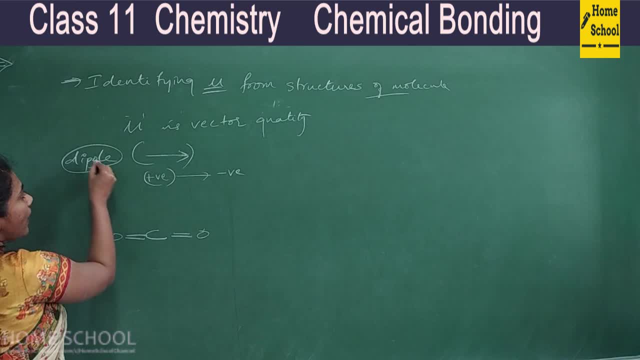 decide. you see, this is a positive part, this is a negative part. so how will you show the dipole? it's a vector quantity. see, dipole will always move from positive to negative side. so this is a vector and this here also dipole. you will observe, oxygen is electronegative, carbon is 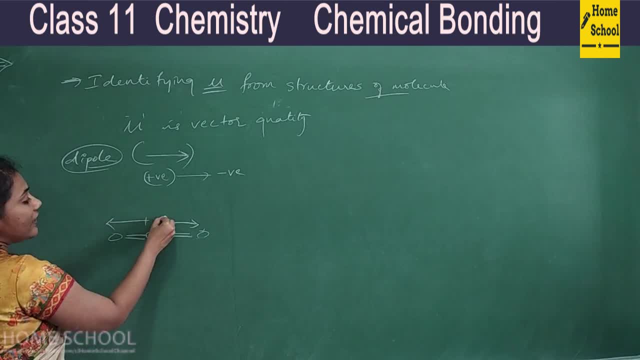 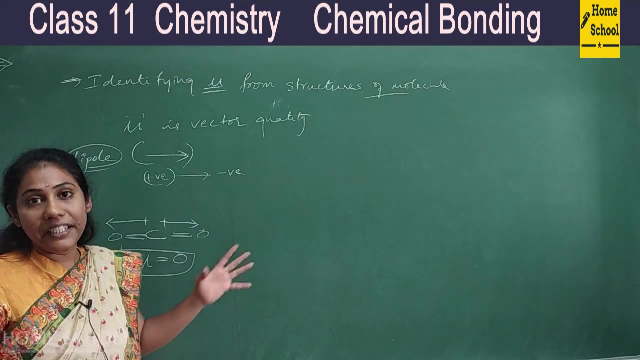 electropositive. so this is the dipole you will show and vector quantity in opposite direction will get cancelled. right? so what is the dipole moment here? dipole moment is zero. okay, so i say this particular molecule is not having any ionic character. okay, so this is how, from structure you. 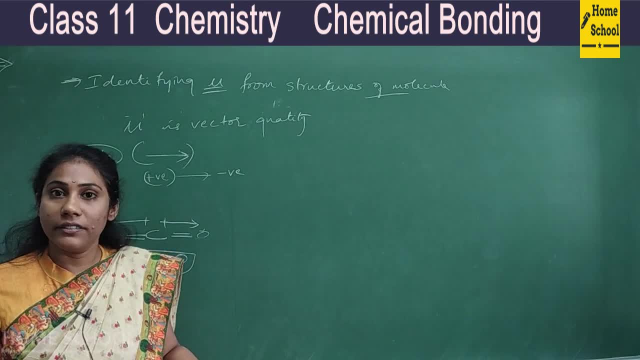 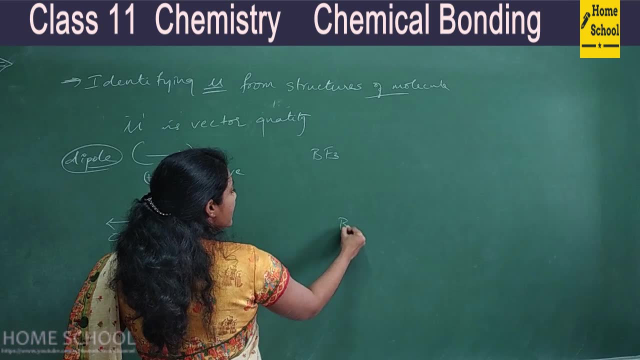 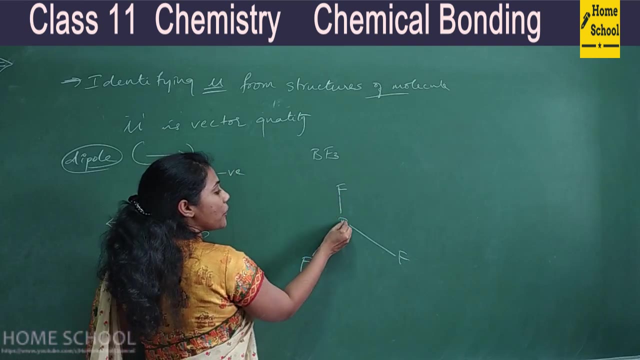 can decide whether dipole moment is there or not. okay, fine, and you know another molecule. let me take b, b, b, the structure of bf3. it is planar, it is planar. and how will you show the dipoles here? this is positive, this is electronegative. so here the dipole is always from positive side to negative. 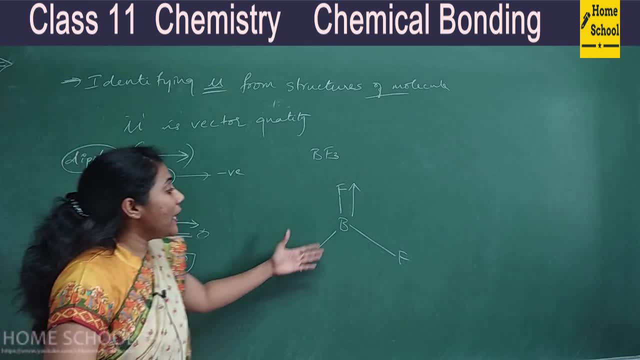 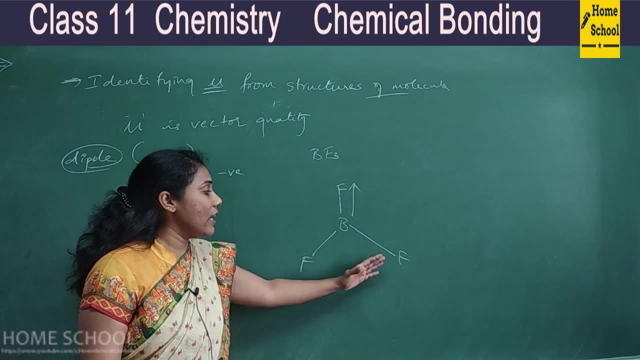 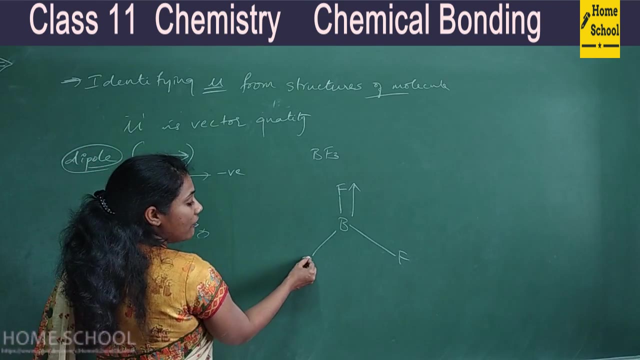 side. that's how you have to show the dipole. okay, from understanding dipoles, dipole is a vector quantity. by understanding this dipole or these vectors, you can decide whether dipole moment is shown by a compound or not. and this bond, how will you for this bond? how will you show the dipole? positive, negative, so dipole you. 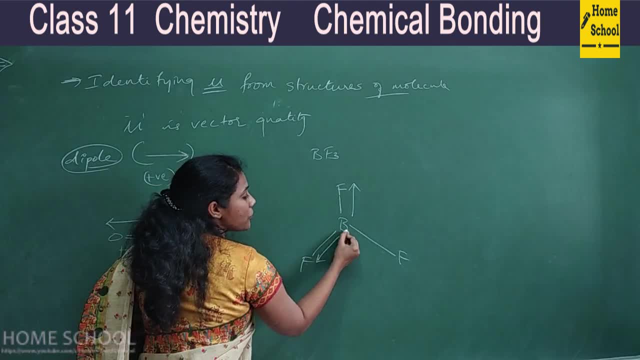 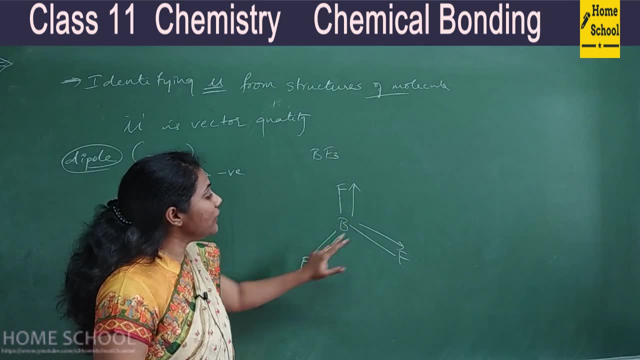 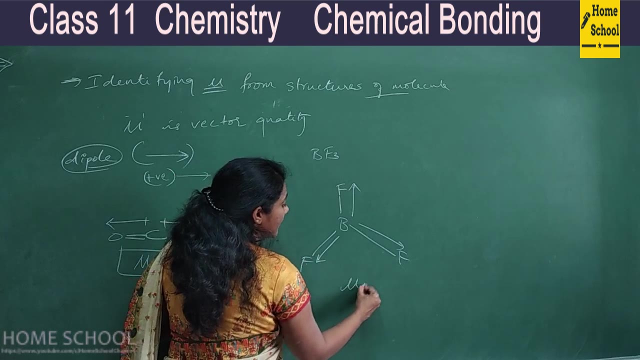 have to show this way for this bond. how will you show the dipole positive, negative? so dipole is this way and it is planar. okay, so for planar, and this is how the dipoles are, okay. so all in different directions and the molecule is highly planar. so here also, dipole moment will be zero, remember. for 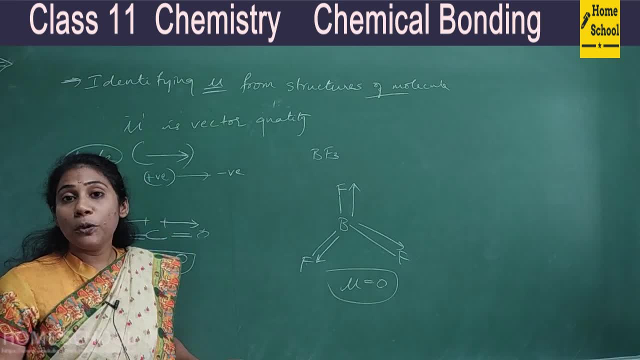 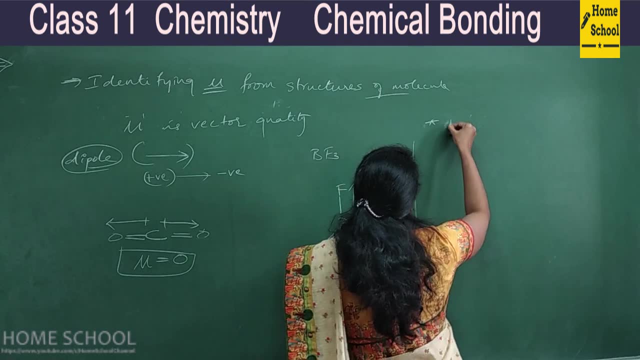 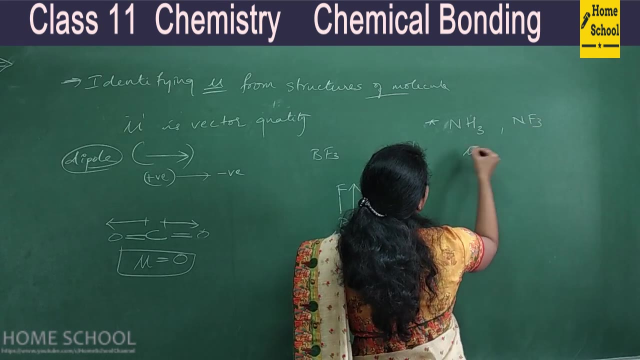 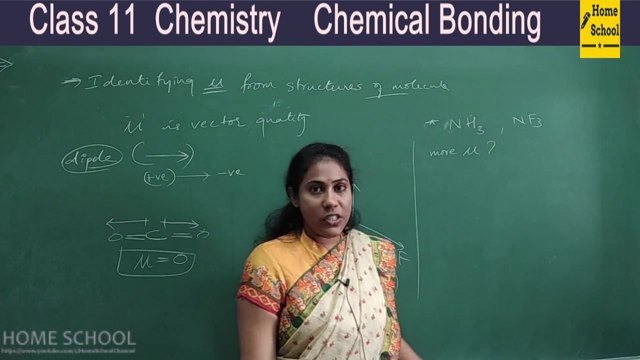 any planar molecule, the dipole moment will be zero. okay, fine. now, coming to very, very important example, i'll compare the dipole moment of nh3 and nf3. so if i ask you which has got more dipole moment among these two, which has got more dipole moment, then you can decide based on their structures. okay, so what? 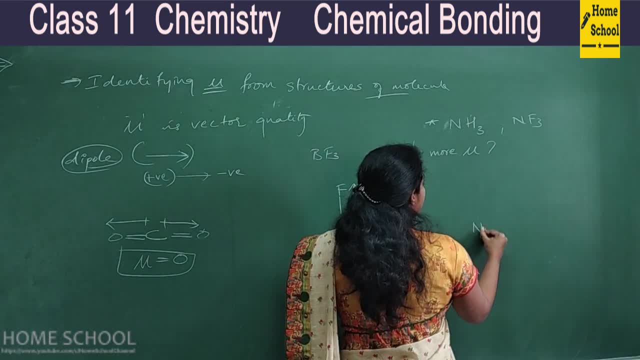 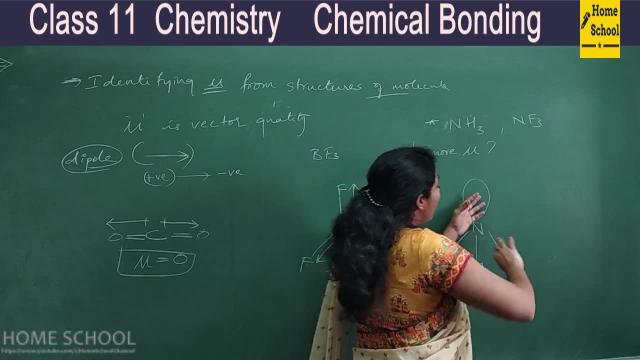 is the structure of nh3. structure of nh3 is pyramidal right. nf3 is pyramidal right. so this is the structure of nh3 and this is the structure of nf3 and this is the structure of nh3 and this is. there is a lone pair. this is out. and how do you decide that this? 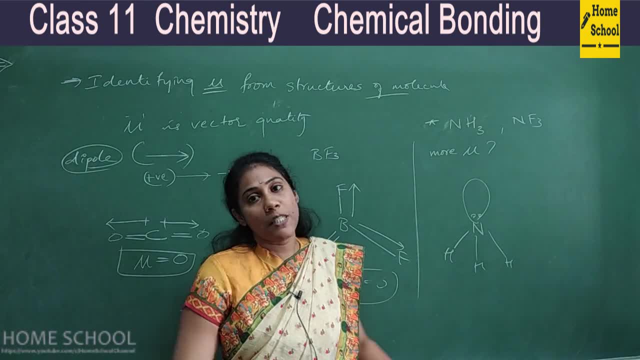 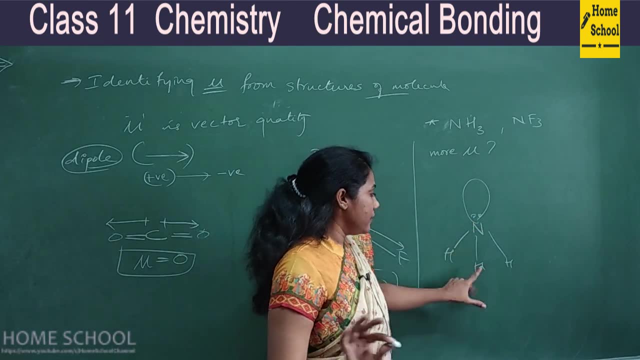 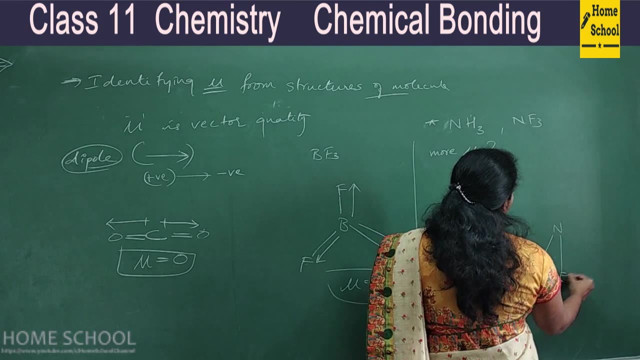 is a structure and this is how we will write. it is based on the vesper theory. hold on, about vesper theory, we will discuss in our next class, okay, so, uh, this is nh3 structure, okay, and nf3, nf3, f, yes, yes, and a lone pair: okay. so how will you show a dipole for this bond? 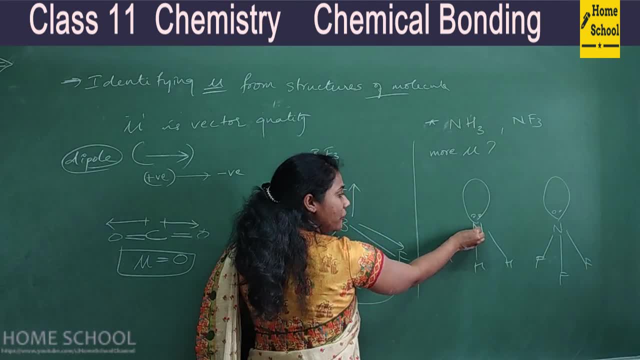 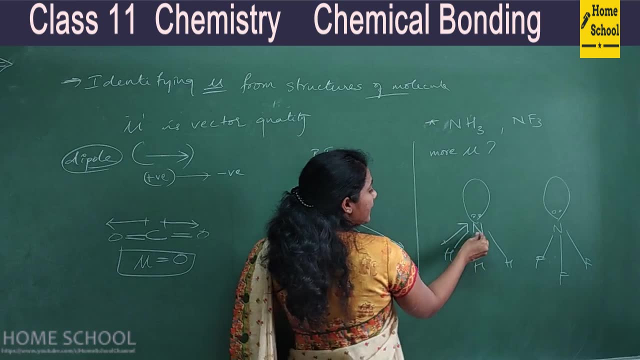 for this bond, nitrogen, more negative, electro negative, hydrogen, electropositive, positive to negative. you have to show the arrow mark. i mean vector. okay, and how will you show the dipole for every bond? you have to show the dipole from the direction you are deciding whether it will show. 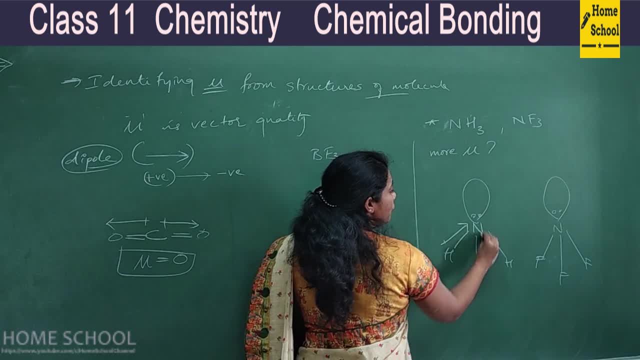 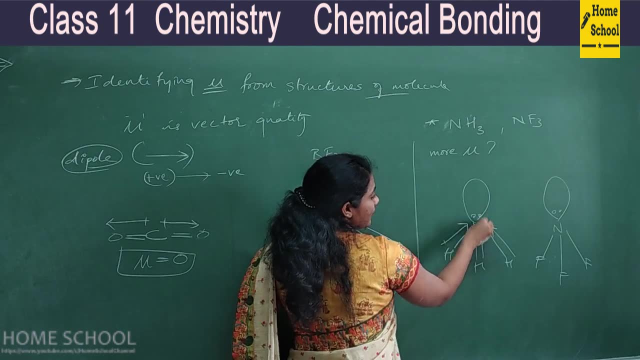 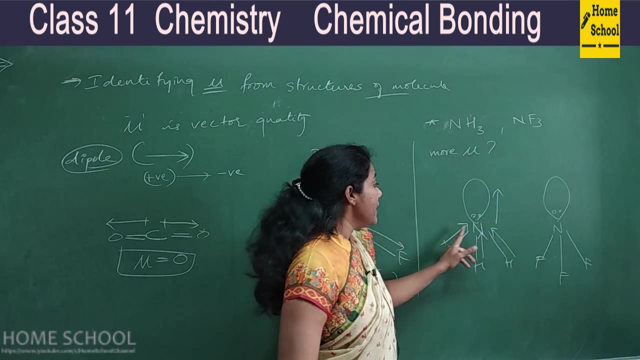 dipole moment or not? okay, so nh bond, how will you show the dipole? like this, nh bond dipole like this: and nitrogen and lone pair. between nitrogen and lone pair, lone pair is more negative. so dipole is like this: see, all arrows are moving in a same direction. say the resultant vector is very much. 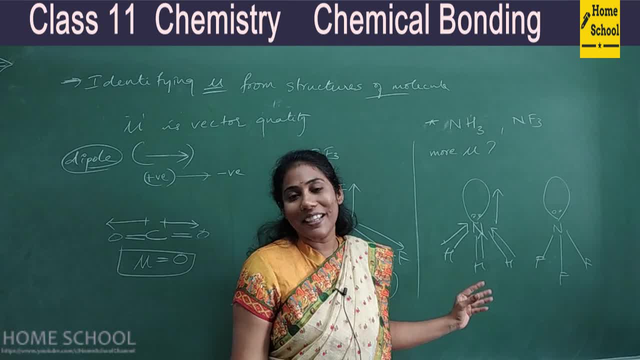 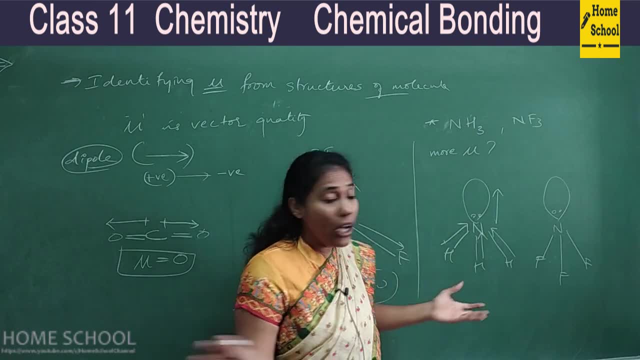 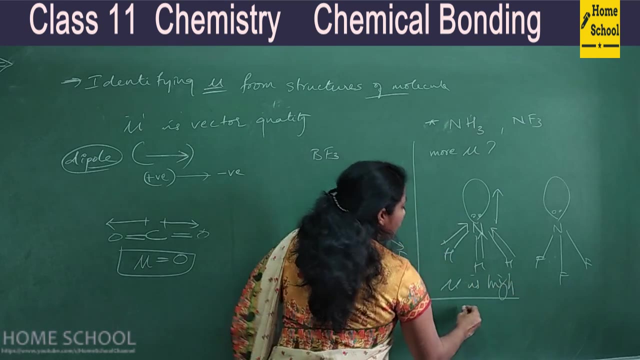 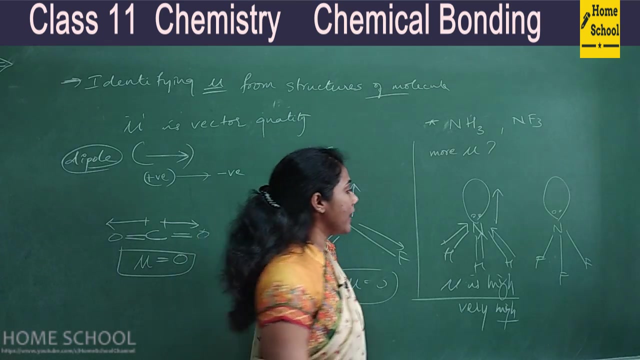 strong, right? so you must know some basic properties of vectors here, okay? so when all these vectors are moving and joining at a single point, the resultant vector is very strong. so here dipole moment is high, dipole moment is very high, dipole moment is very much high, okay, so very high, very high, because the resultant vector is very, very strong, right, okay? 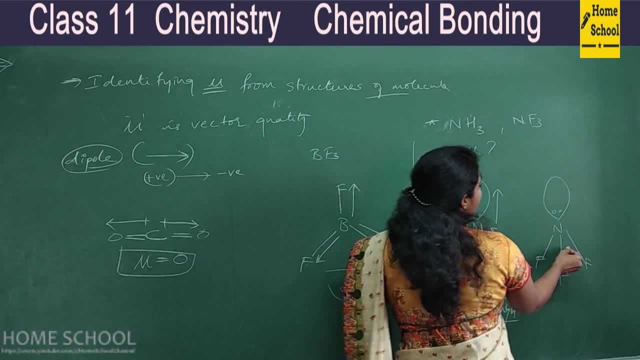 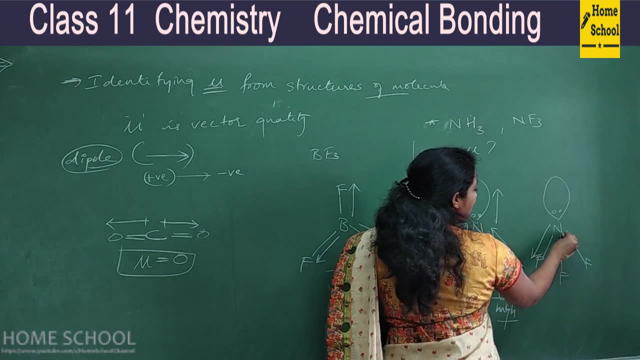 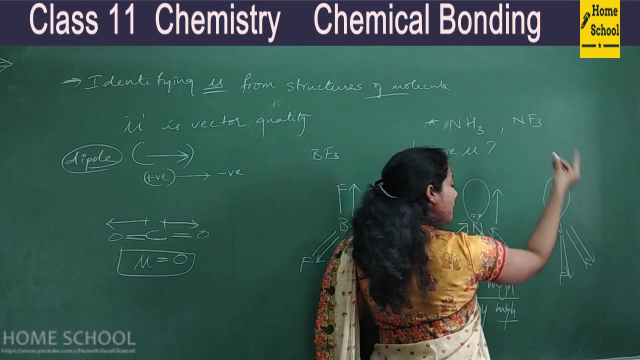 and coming to nf3. so how will you show the dipoles for a bond? compared to nitrogen, fluorine is more electro negative, so the dipole is like this. and for this bond dipole is like this. for this bond dipole you will show like this: and here, between nitrogen and lone pair, lone pair is more negative. 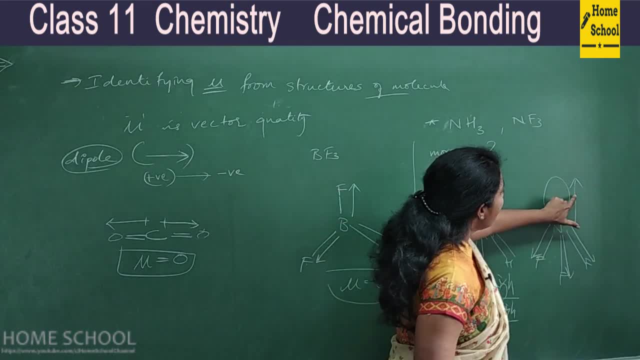 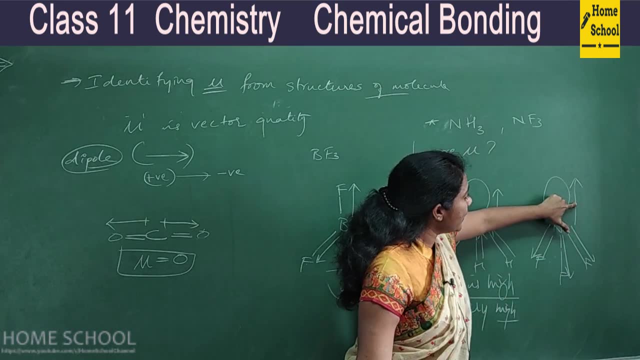 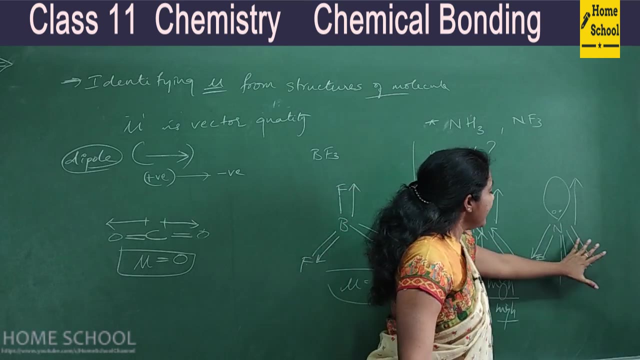 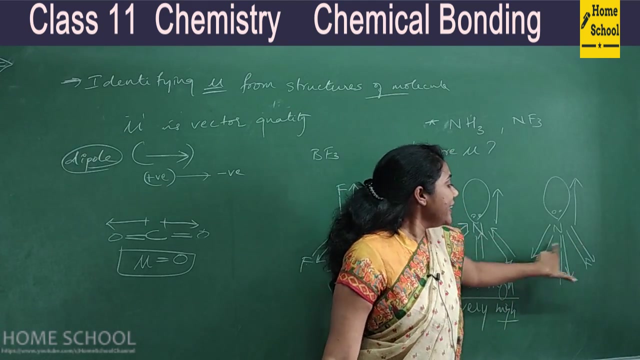 so dipole you will show up and here you see, one arrow direction will get cancelled with another arrows direction, right? so if you take this above arrow and any one below arrow, they will get cancelled, right. so the resultant dipole is due to only two arrows. the resultant dipole is due to only any two bottom arrows. okay, so that's. 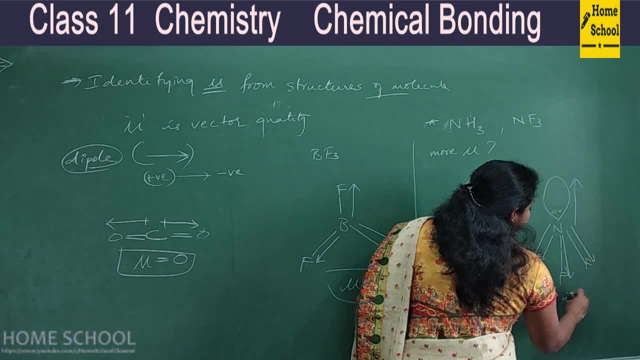 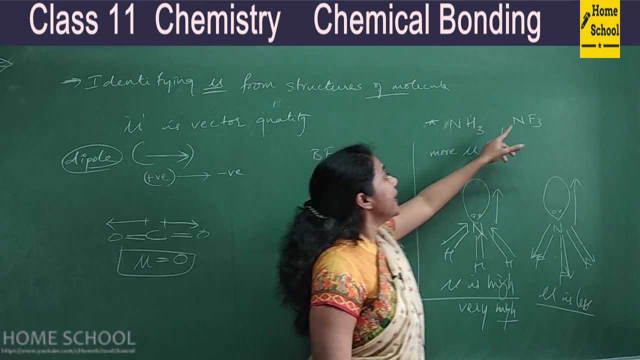 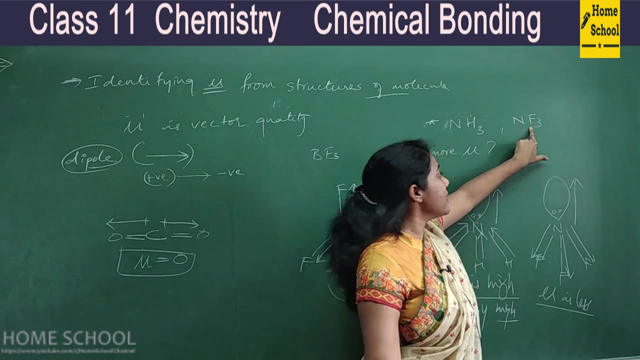 why here you will observe dipole moment, but the dipole is less, dipole is less. see the moment you see here you would think that nf3 has got greatest dipole moment because, uh, you know, electro negative elements are three, right, fluorines are three, but no, nh3 has got more dipole moment, that has decided.